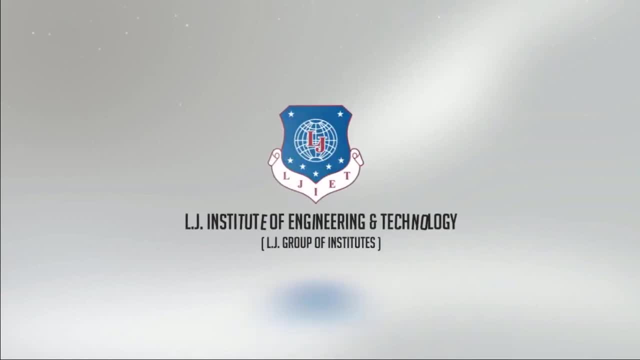 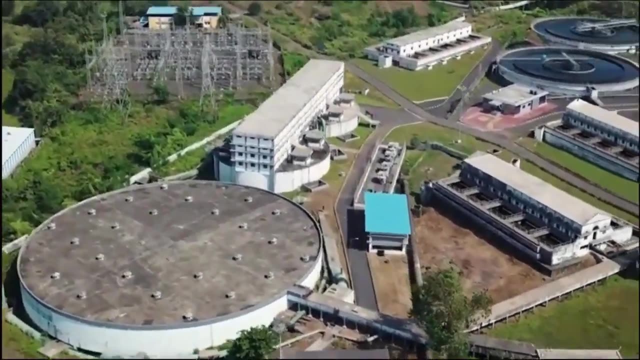 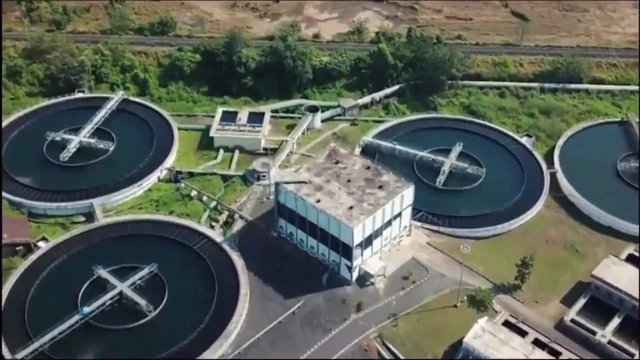 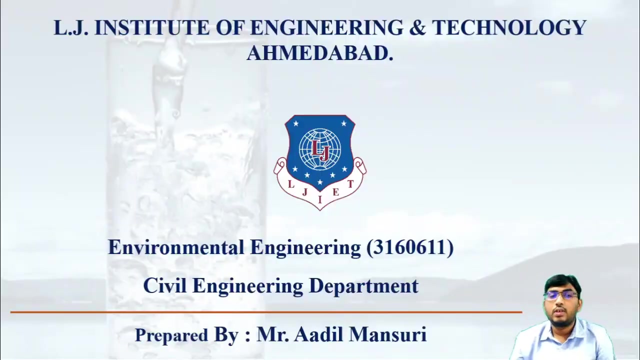 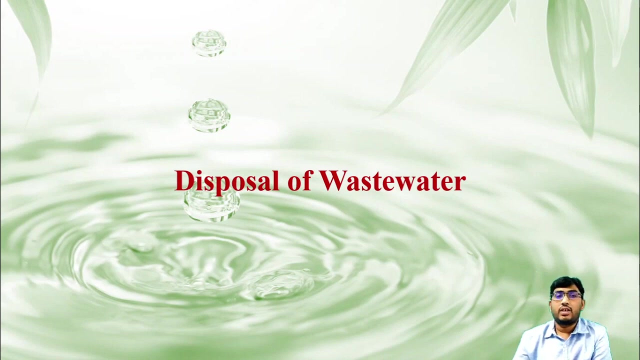 Welcome back students to the video lecture series. I am Adil Mansuri from Civil Engineering Department of LJ Institute of Engineering and Technology. So, my dear students, in the previous video we had already discussed regarding the BOD and the first stage of BOD. right In this video we will start with disposal of wastewater. 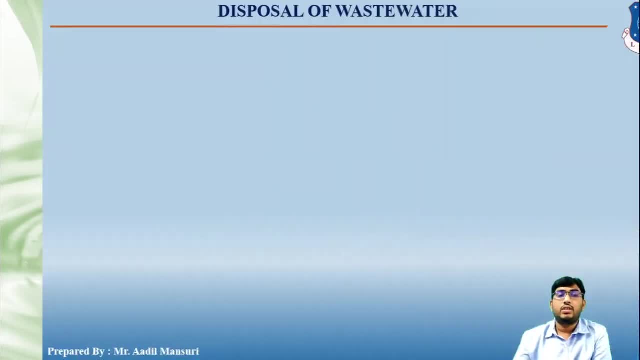 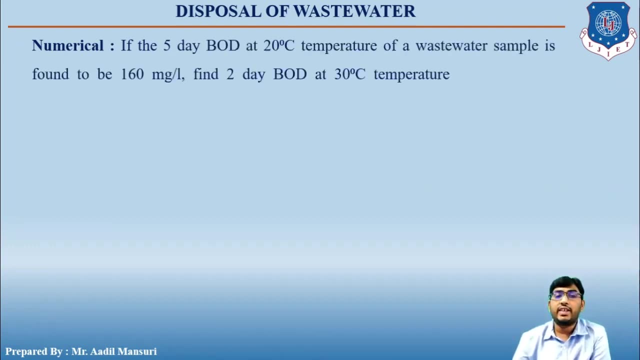 But before that we will continue with the numerical of BOD. So the data says: if the 5-day BOD at 20 degree centigrade temperature of a wastewater sample is found to be 160 milligram per liter, then find 2-day BOD at 30 degree centigrade temperature of the 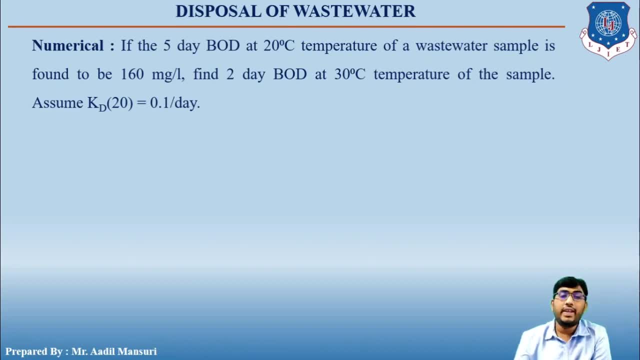 sample. We are told that assume Kd 20, that is coefficient at 20 degree to be 0.1 per day. okay, So let us start with the solution. So we are given the 5-day BOD at 20 degree. 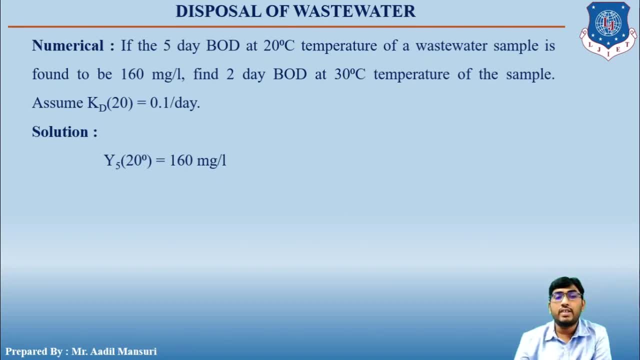 That means y5 at 20 degrees is equal to 160 milligrams per liter. Okay, so BOD is represented as y. okay, So if it is 5-day BOD, then we write in subscript as y5 in the bracket at 20 degree. 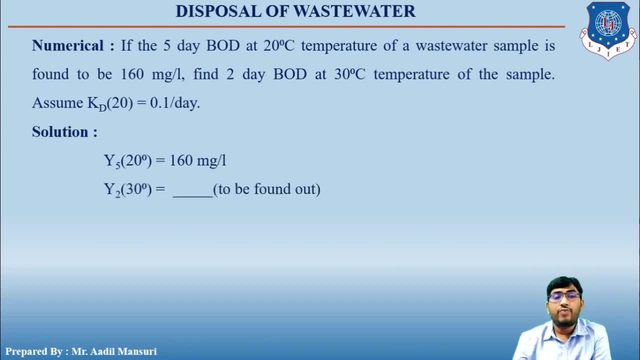 centigrade. Okay, Then we need to find out the 2-day BOD at 30 degrees centigrade. Now we are given constant Kd at 20 degree as 0.1 day per day, And the 1-day BOD is represented. 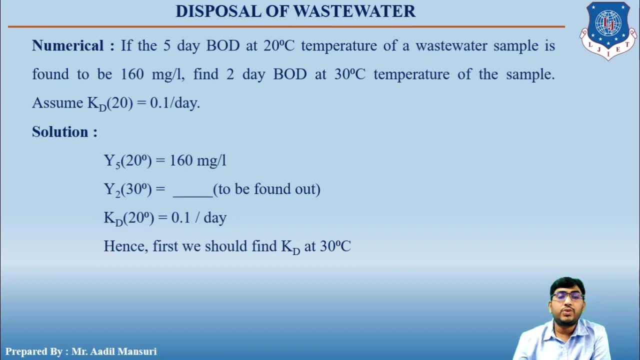 at 0.1 degree centigrade. Okay, Now we are given the 3-day BOD at 20 degrees centigrade, right? So first we should find out constant at 30 degree centigrade, Now to find out the constant. 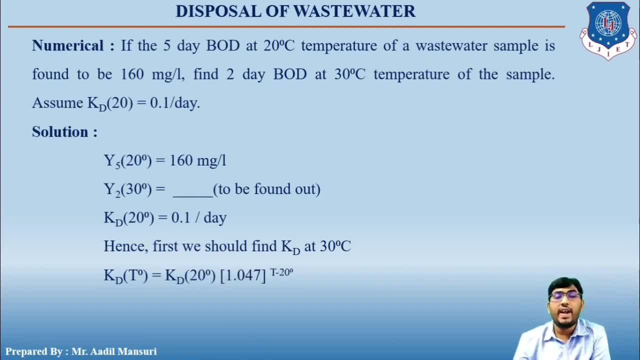 we have formula that Kd at any temperature T equals to Kd at temperature 20 degree centigrade into 1.047 raised to T minus 20 degree. That is, T should be the temperature at which we need to find out the constant. ok, So if we need to find out the constant at 30 degree centigrade, 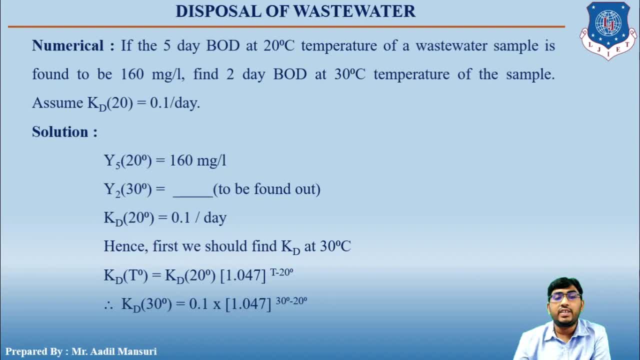 then we can write that Kd 30 degree equals to Kd at 20 degrees, 0.1 into 1.047 raised to 30 degree minus 20 degree. ok, So Kd at 30 degree comes out to be equals to 0.158, ok Now. 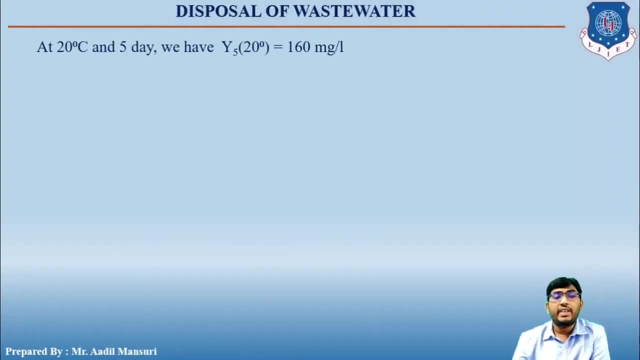 at 20 degree centigrade N5, 5 day, we have: Y5 equals to 160 milligram per liter. Now, from the equation of Yt right, Yt equals to L into 1 minus 10, raised to minus Kd T. ok, Now Yt is given as 160. 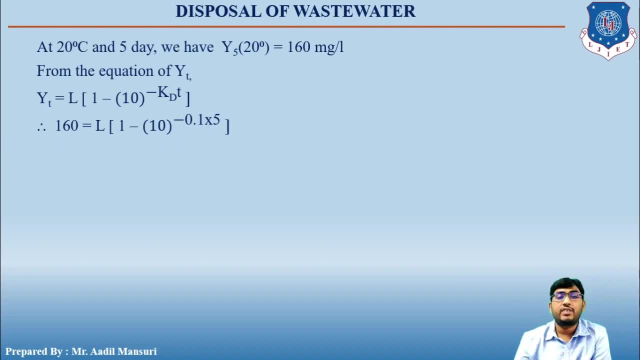 equals to L. 1 minus 10. raised to minus Kd is already at 20 degree, that is, 0.1 into 5, ok, Fine. So this comes out to be equals to 160, equals to L into 0.6837.. Therefore, L is equals. 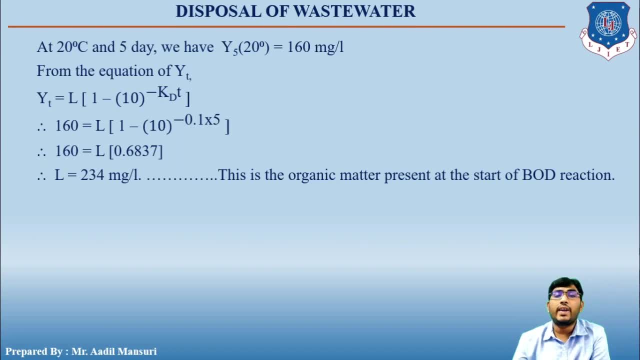 to 234 milligram per liter. So this is the organic matter which is present at the start of the BOD reaction. ok, Now again. Yt equals to L into 1 minus 10, raised to minus Kd T. 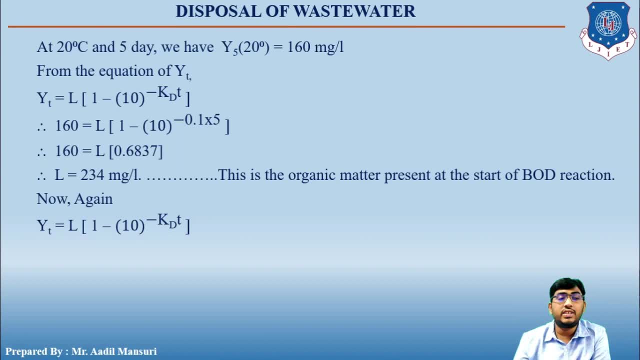 we know the formula right Now. we have received this L. we have already found out the L. that is initial concentration, right, So we can find out BOD concentration at the required day. ok, So we required at 2 day, right, that is, after 2 days. 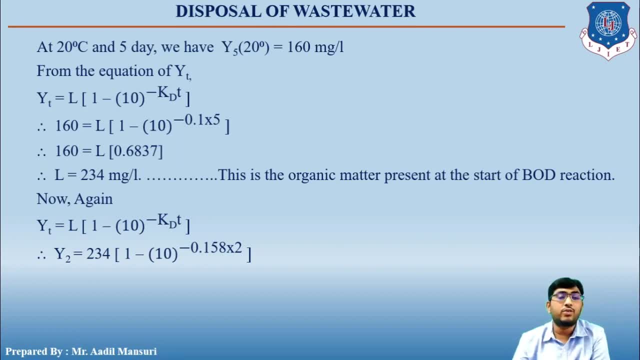 So Y2 will be equals to L In place of L. I am putting 234, 1 minus 10 raised to minus Kd T right where if you are finding at 2 day at 30 degree, then we need to take the constant Kd at. 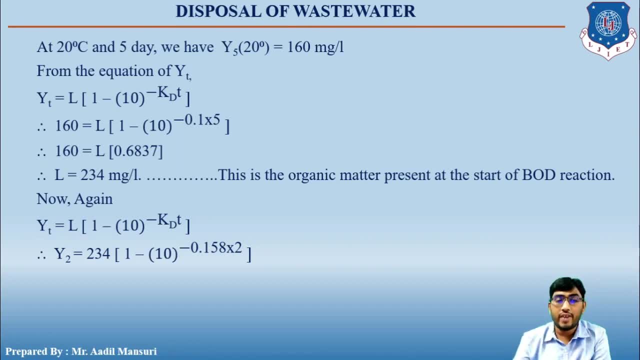 30 degree. So we are getting the constant Kd at 30 degree, right? So we are getting the constant Kd at 30 degree that we have found out, that is equals to 0.158 into 2, right? So this comes. 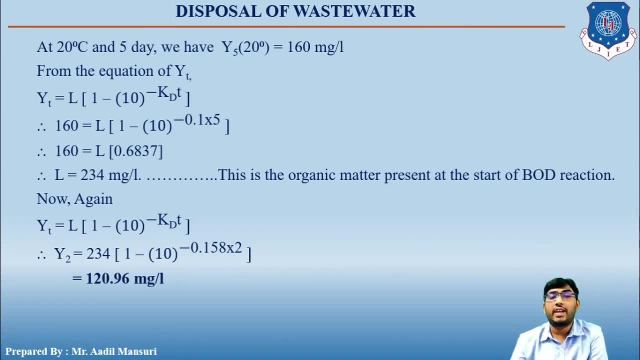 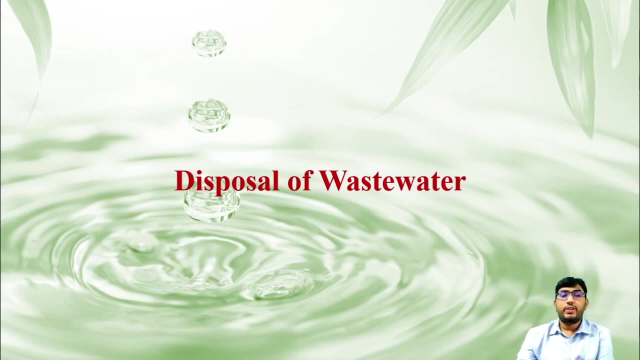 out to be equals to 120.96 milligram per liter. ok, So this is the numerical for finding out the BOD. ok, Ok, students. So let us now start with the next topic, that is, disposal of wastewater. 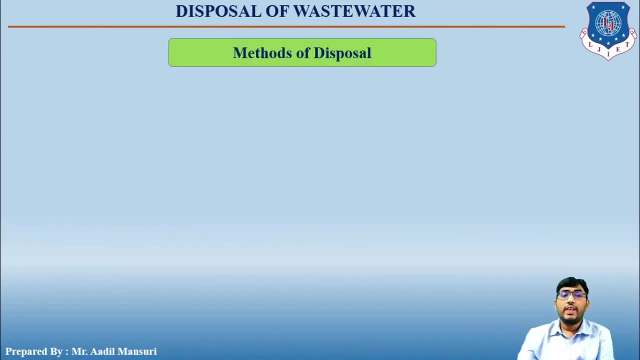 ok, So there are various methods of disposal. There are two types basically. First one is natural methods, right, and another one is known as artificial methods. So in natural method consists of by dilution, that is, by diluting the wastewater, and second one is the land treatment Talking. 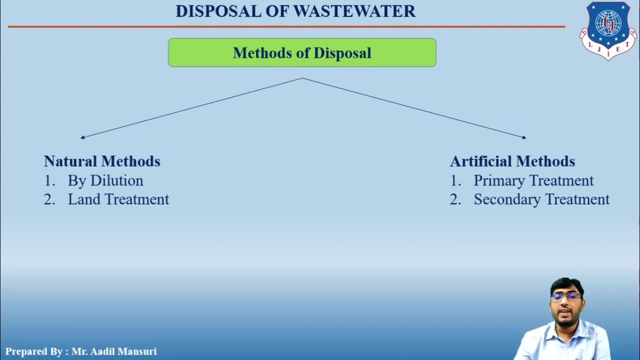 about the artificial methods. there is a primary treatment and the secondary treatment. So let us now start with the dilution. So dilution is predominant natural method of disposal. ok, and disposal by dilution is the process where the raw or treated sewage 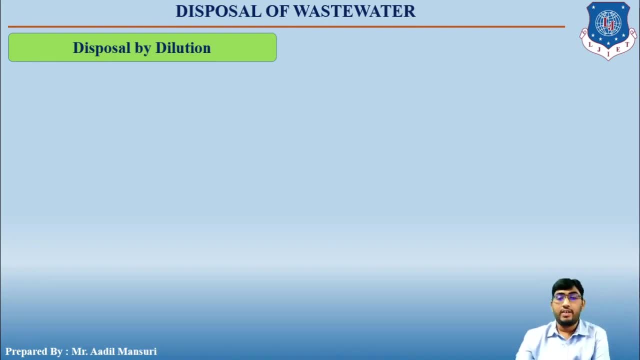 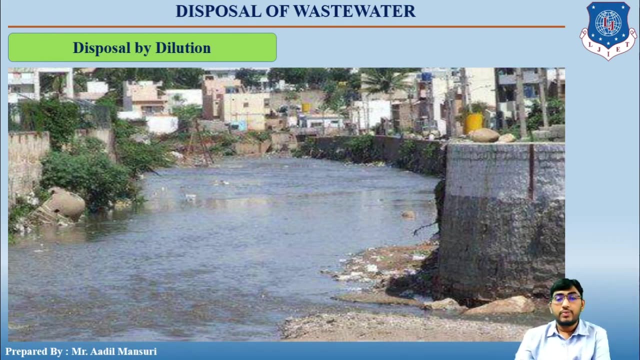 is discharged into water bodies such as rivers, lakes, sea, etc. ok, Now the discharged sewage, in due course of time, is purified by method of disposal, Which we call as the animal- jijjayi. ok, This is a process that is done for sure of day, due to the end of day. So the source: 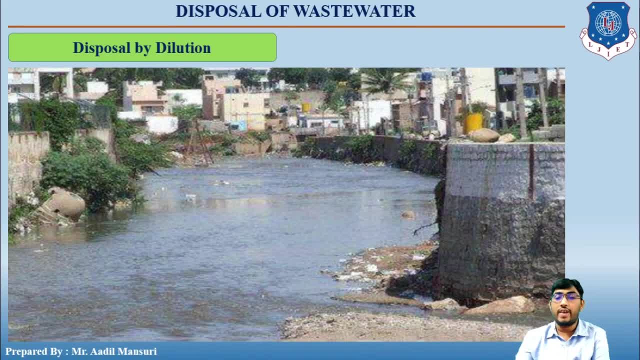 of the discharge of sewage is downpour of water, So the water that is거든요 to the wastewater by self-purification process of natural waters and the sewage is mainly purified due to the oxidation of organic matter by bacteria using the dissolved oxygen which is present in the 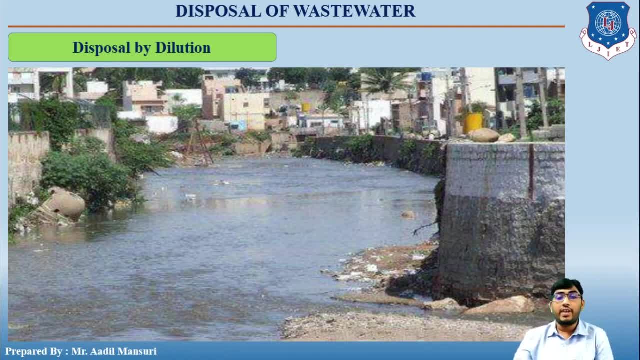 water bodies. Now, the degree of treatment given to the raw sewage before disposing it into any river will depend not only upon this quality of raw sewage, but also on the self-purification capacity of the river and the intended use of its water at the downstream side. 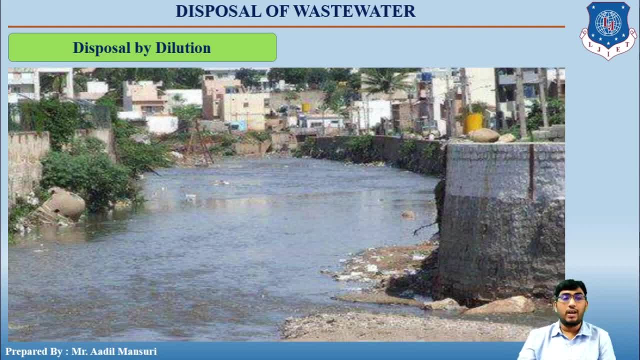 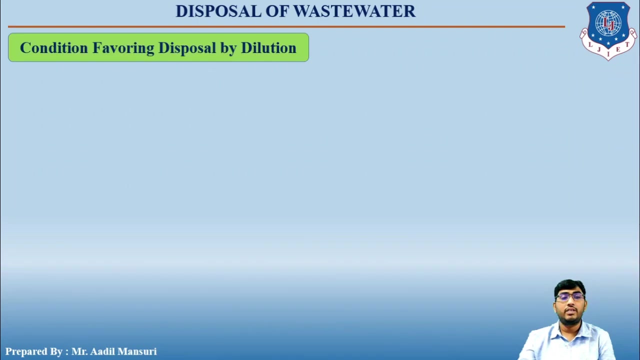 This method can be used only for the towns or cities which are located near the river or sea or have a large lake which can be used as a source of disposal. So you can see in the picture. so let us move ahead. so let's talk about the condition favoring disposal by dilution. okay, 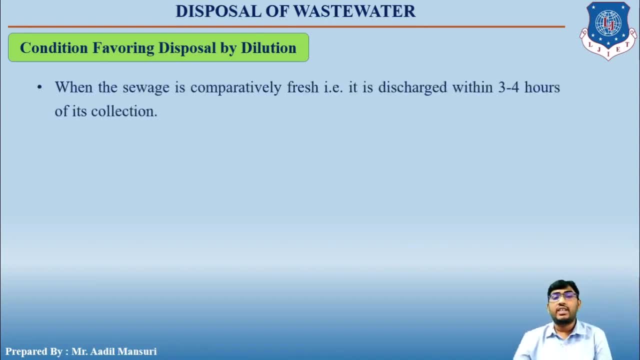 so when the sewage is comparatively fresh, that is, it is discharged within three to four hours of its collection, then you can go for disposal by dilution. okay, then, when the floating matter and settlable solids have been removed by primary treatment, then you can use dilution methods. 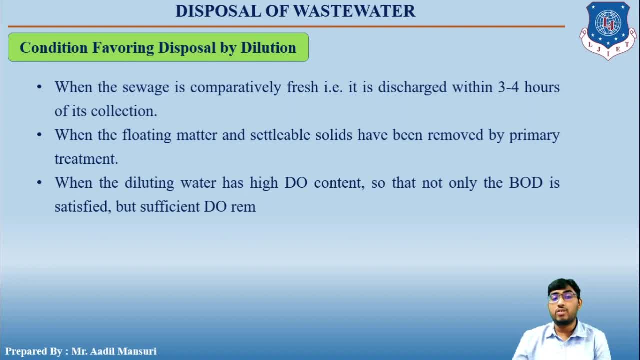 Then when the diluting water has a high dissolved oxygen content, so that not only the biochemical oxygen demand is satisfied but also sufficient dissolved oxygen remains available for the aquatic life. okay then, where the dilution water are not used for the purpose of navigation or water supply for at least some reasonable distance on the downstreams from the point of 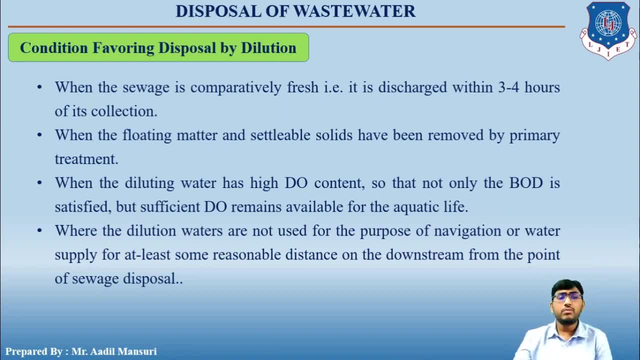 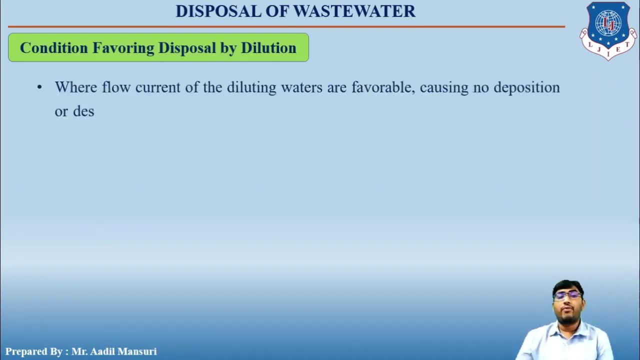 disposal. Next, you can go for dilution, where flow current of the diluting waters are favorable and causing no deposition or destruction of the aquatic life. okay, it means that swift forward currents are helpful, as they easily carry away the sewage to the point of unlimited dilution. On the other hand, 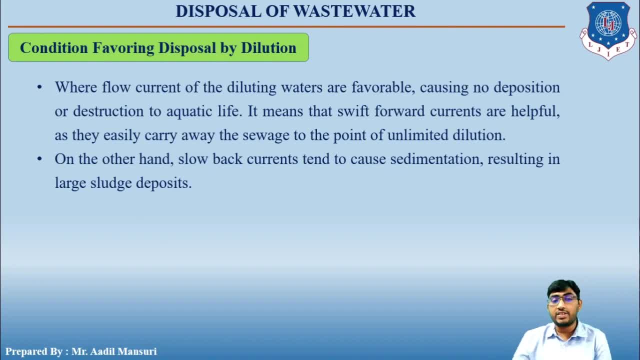 slow back to the point of unlimited dilution. Now you can also use the dilution process where the waste water does not contain industrial waste water having toxic substances and where the outfall sewers of the city or the treatment plant is situated near some natural waters. okay, 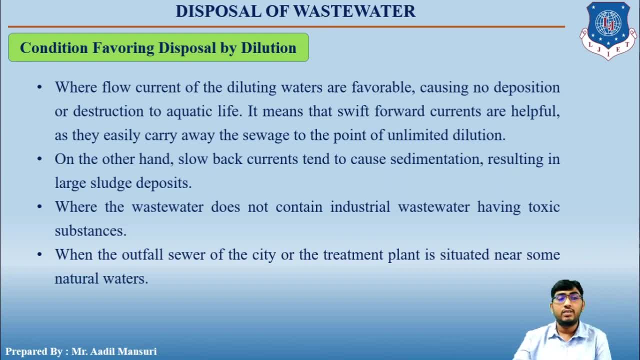 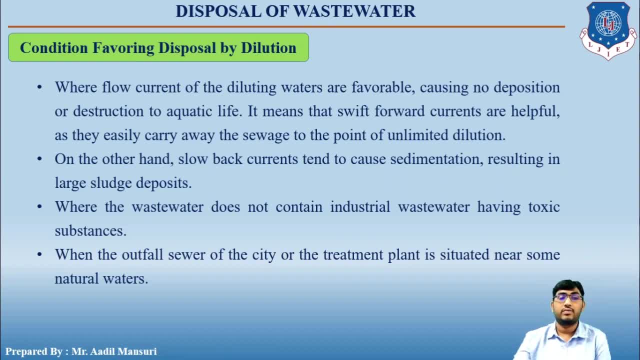 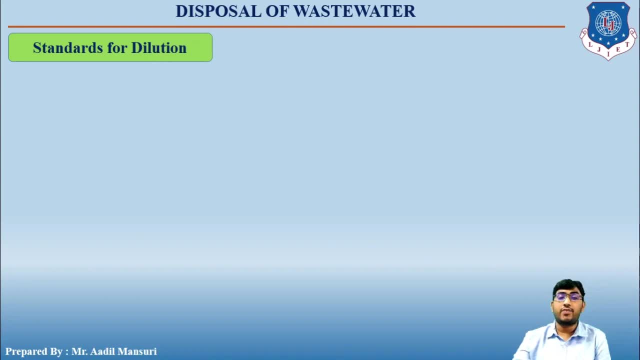 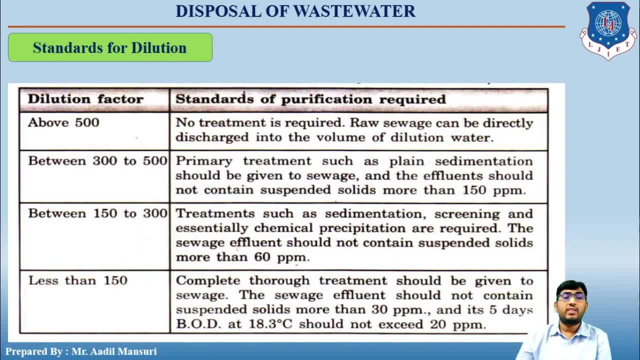 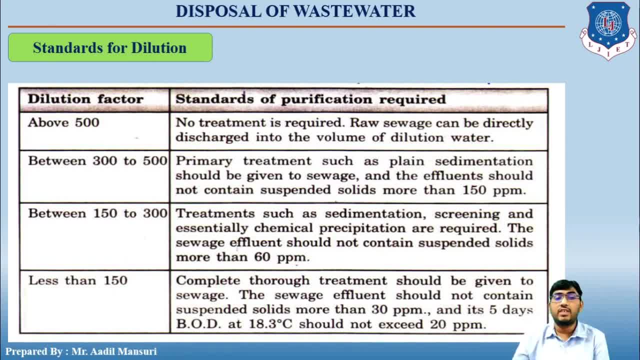 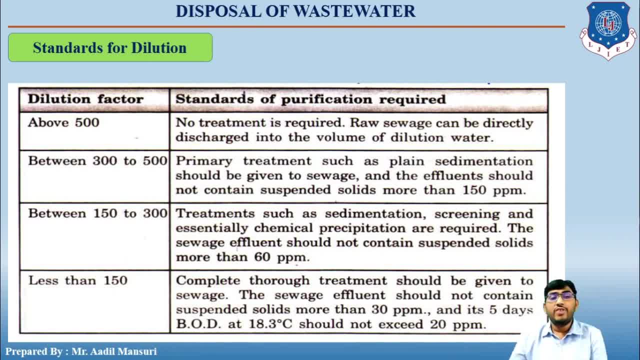 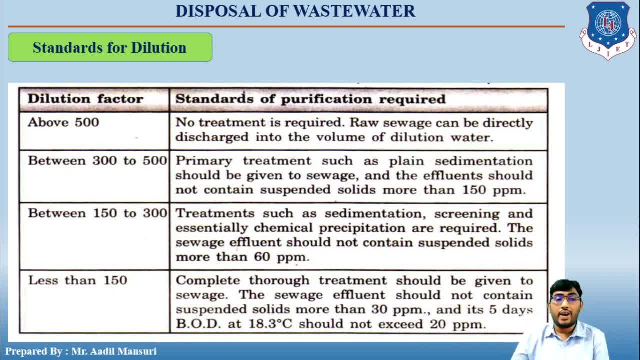 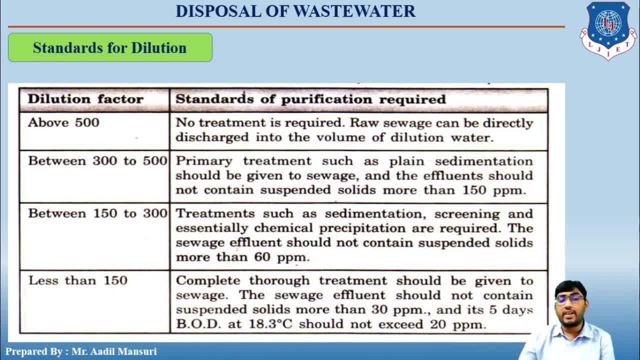 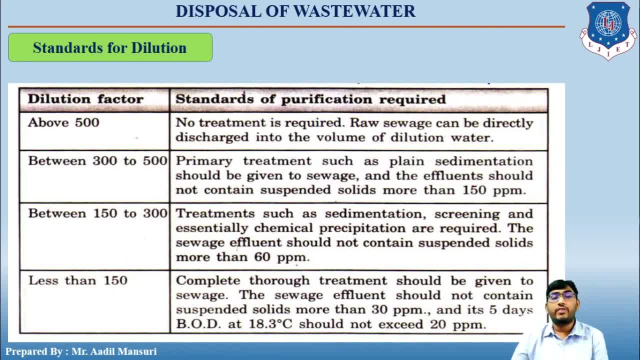 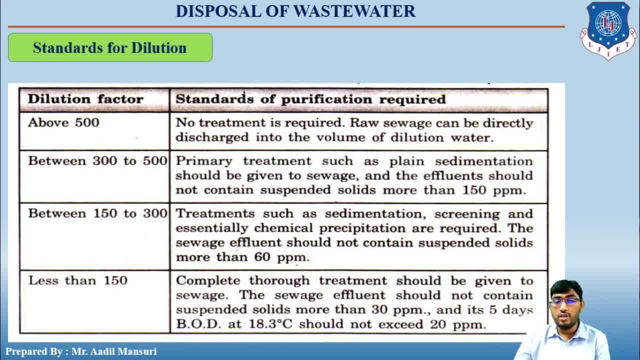 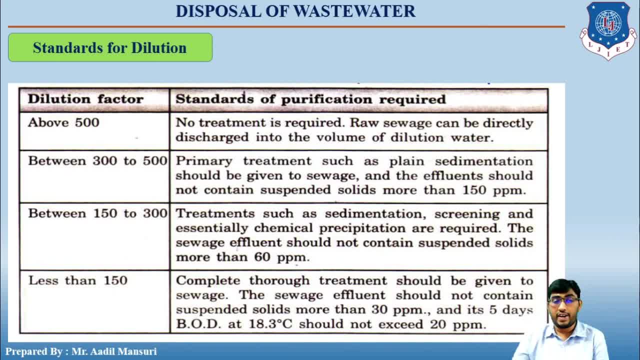 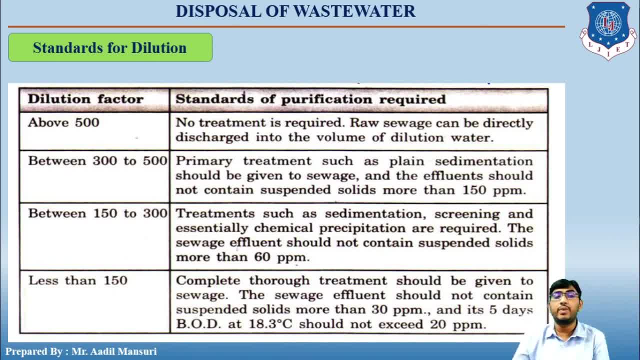 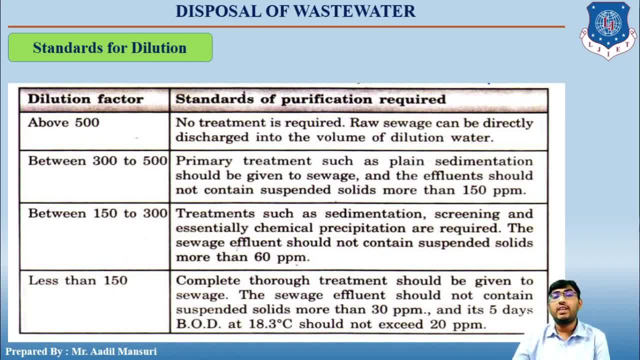 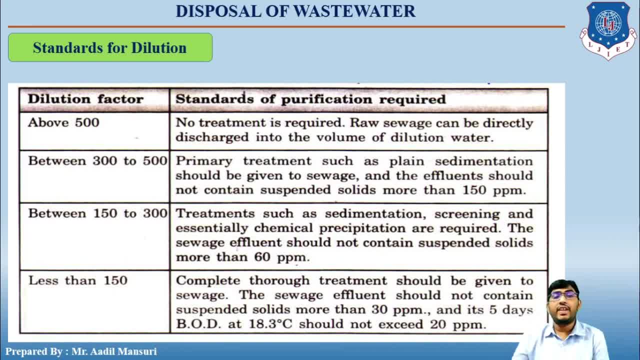 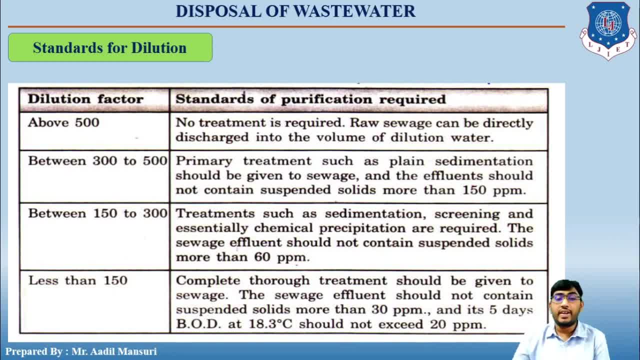 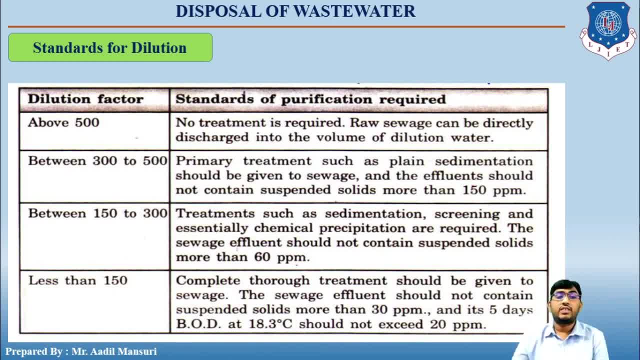 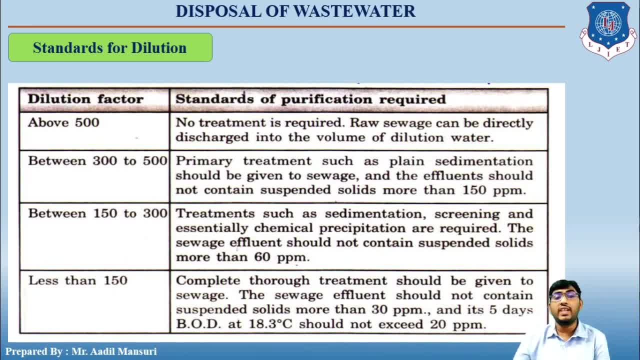 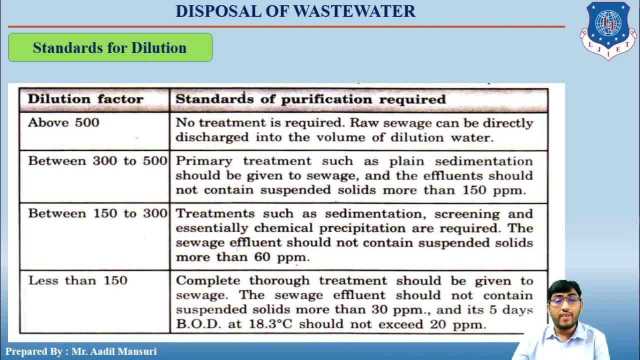 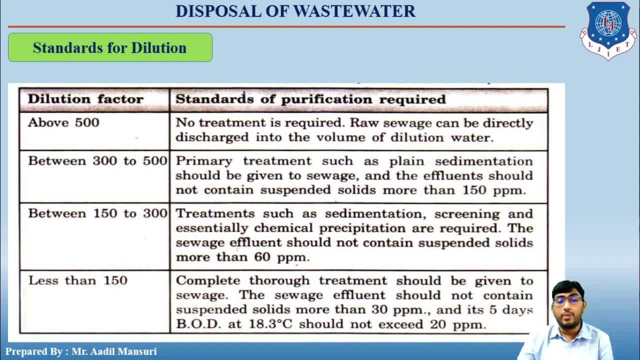 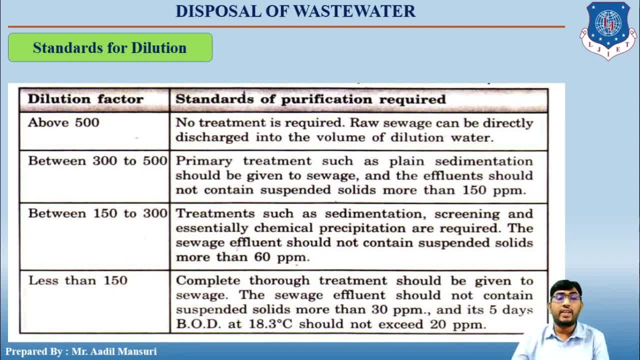 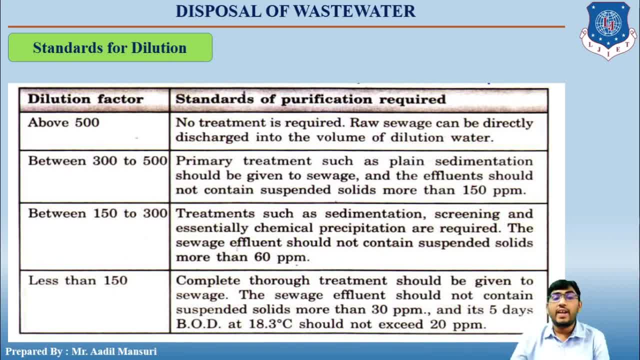 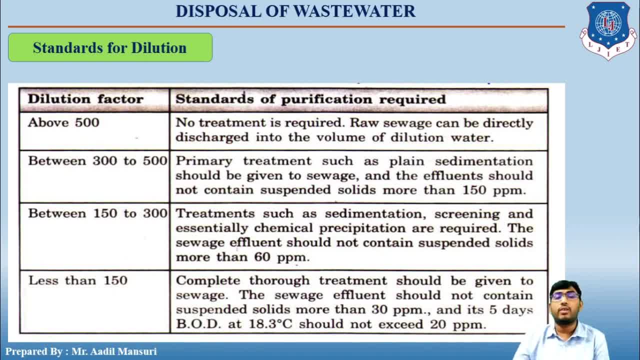 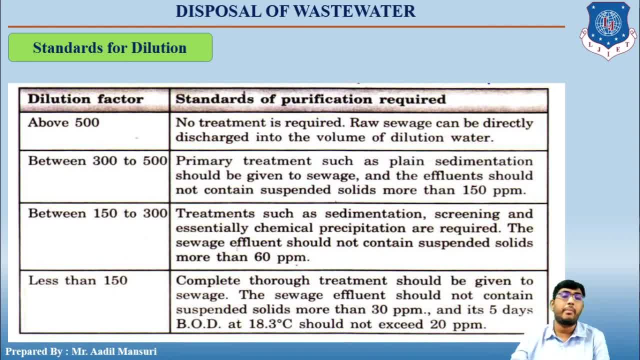 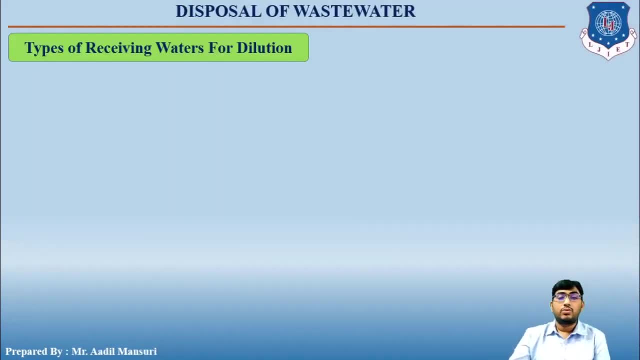 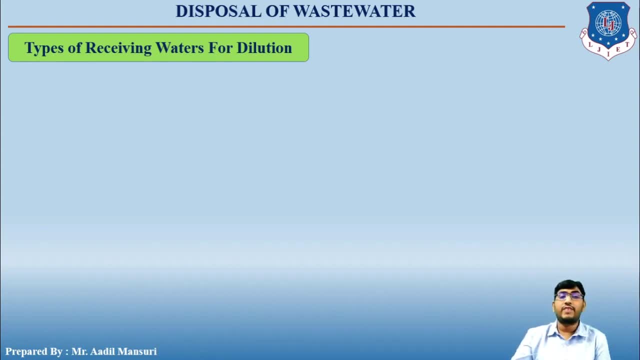 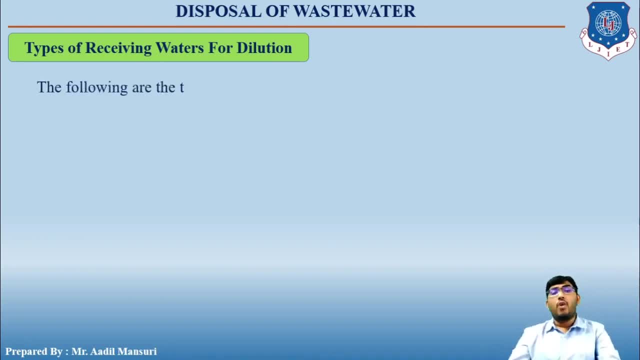 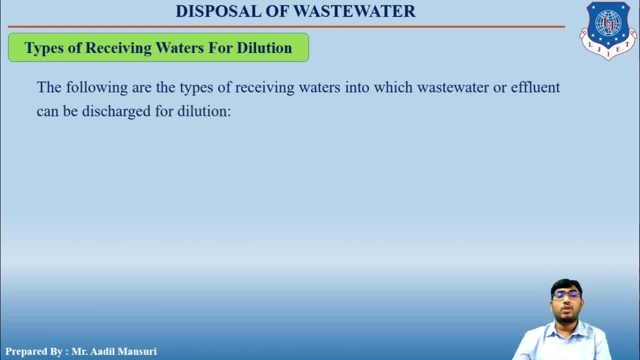 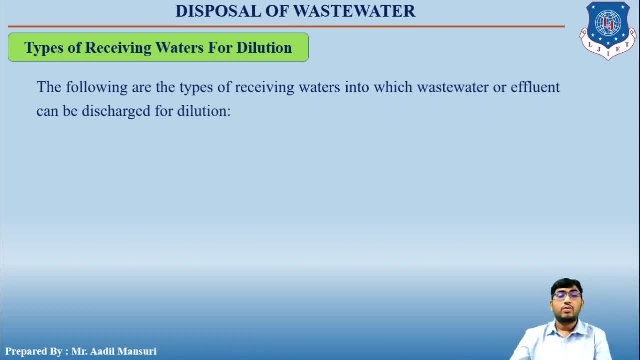 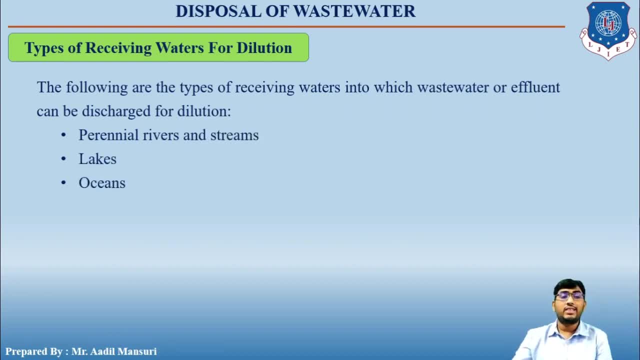 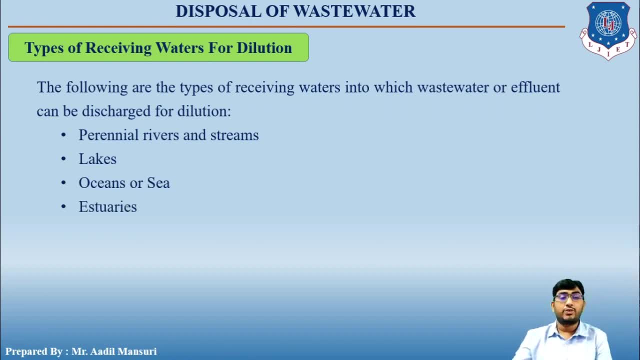 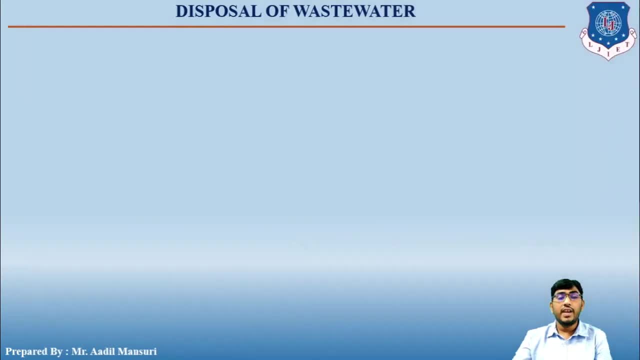 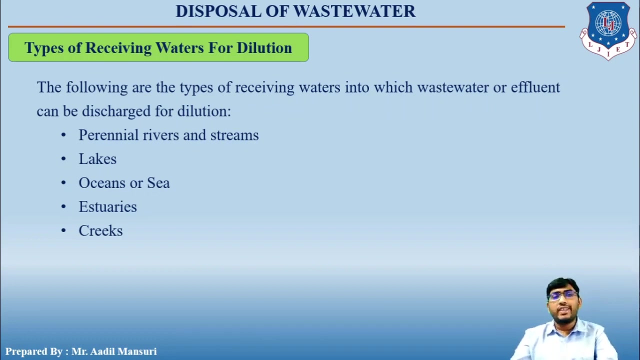 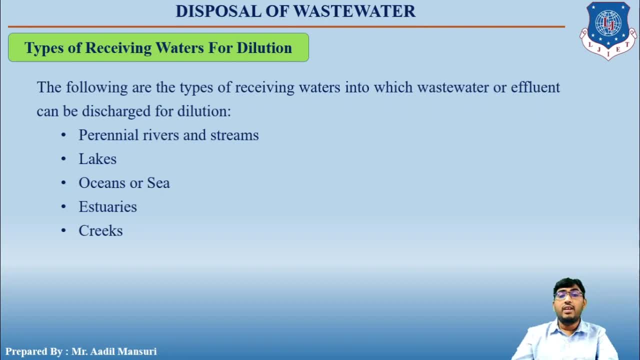 So the dilution factor may be low, And also higher temperature of water may result in low solubility of oxygen, necessitating proper treatment before dilution. Okay, So this was regarding perennial rivers and streams. Then sometimes, especially when perennial streams are not available, then you go for lakes. 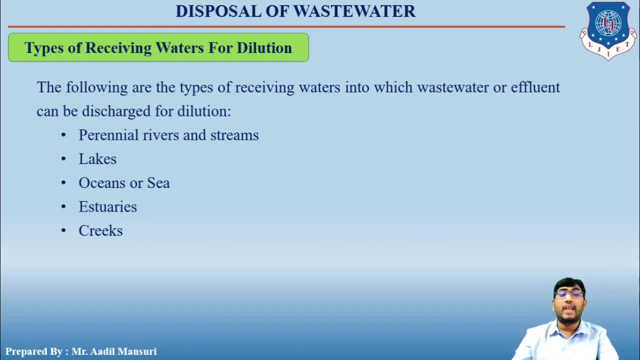 Okay, So various characteristics of lakes, such as size, shape, volume of fresh water flowing into it, etc. should be critically examined before deciding the self-puring capacity. Okay, Then talking about oceans, or sea. oceans has abundant water. 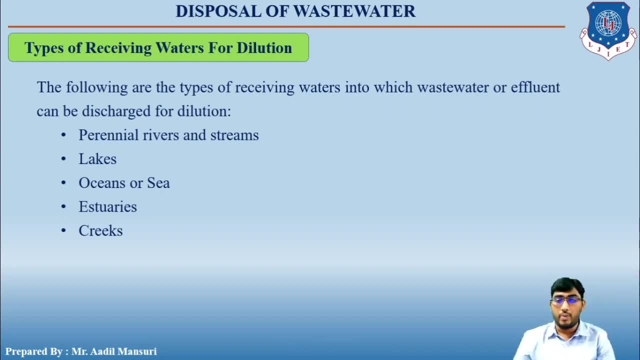 so that dilution factor is unlimited. Number one, Okay. However, seawater has about 20% less dissolved oxygen than river or stream. The water is turbid due to dissolved impurities, and penetration of sun rays is also less Okay. 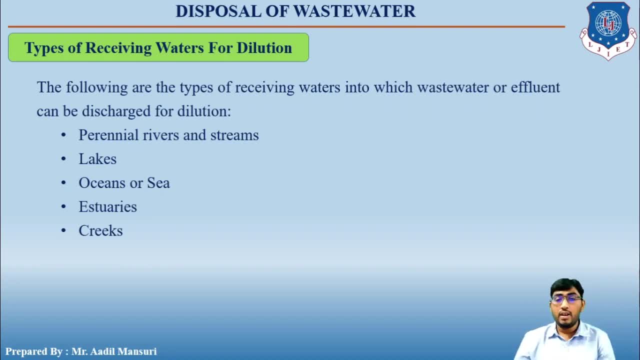 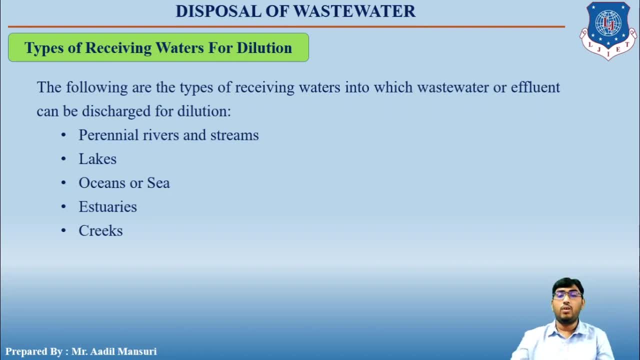 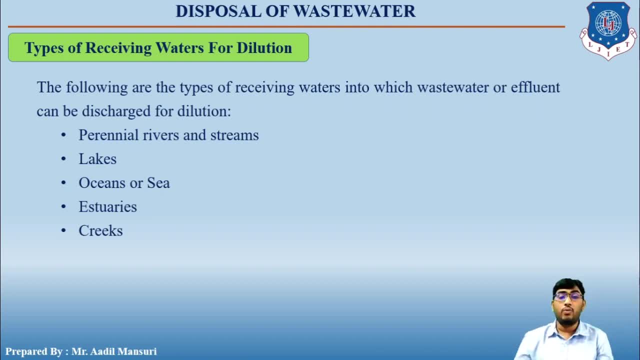 Okay, Which may not have dry weather flow during some part of the year. Due to this, great care should be taken in disposal of effluent into it. Clear. Then, talking about estuaries, it is wide lower tidal part of the river, hence dilution is an. dilution is affected both by ocean water. 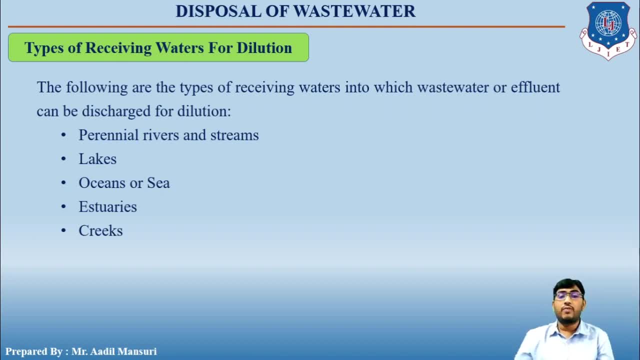 as well as river water. however, the process of dilution is generally satisfactory in such cases. okay, so these are the different types of receiving waters for dilution, so let us move ahead. so next topic is self-purification. okay, now, when the waste water or effluent is discharged into natural body of water. 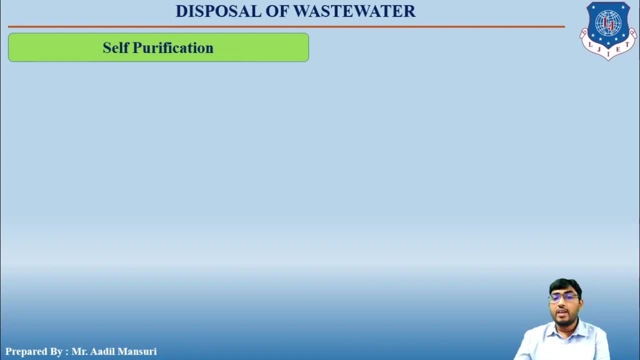 the receiving water gets polluted. right, because we are dumping waste products. okay, now the conditions do not remain so forever. okay, because it does not remain. that is polluted because the natural forces of purification or natural action of purification, such as dilution, sedimentation, oxidation reduction, etc. go on acting upon the pollutants and bring back the water. 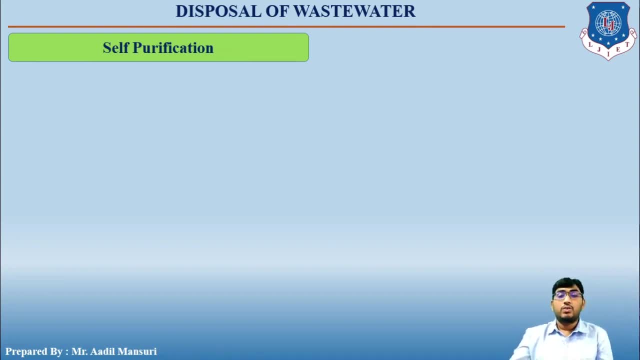 into original conditions. okay, so the actions which are involved in self-purification include dilution, dispersion, sunlight, which act as a dirty water from the water through biochemical reactions, chemical forces aided by biological factors called biochemical forces, which include oxygen oxidation, that is, bio oxidation, and 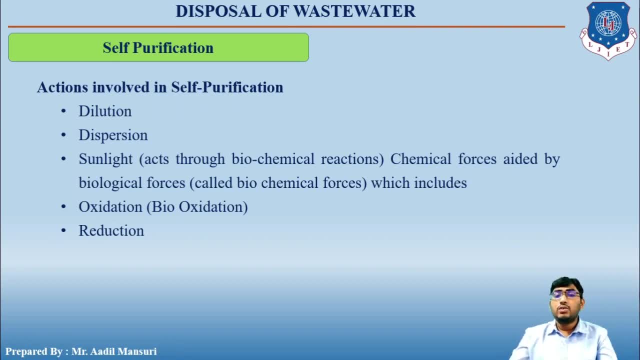 reduction. okay, so this automatic purification of water, polluted water in due course of time- is called the self-purification. okay now the organic matter present in the sewage is broken down by bacteria which are present in the streams of water, to ammonia, nitrate, sulfate and carbon dioxide. now in the 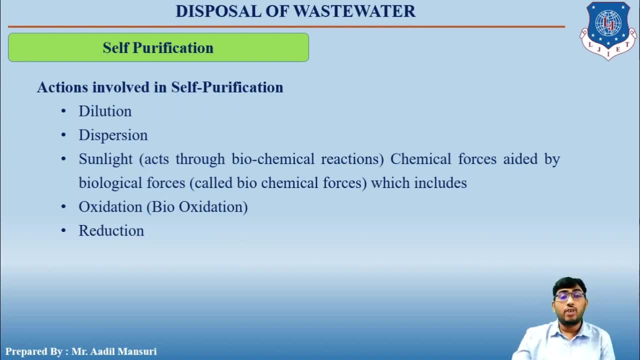 process of. in this process, dissolved oxygen content of the natural water decreases and deficiency of dissolved oxygen is created now. Now the dissolved oxygen is replenished by diffusion of oxygen from the atmosphere, which is known as reaeration. The stable byproduct of oxidation mentioned above are utilized by the plants and algae to form the foods for protozoa, rotifers or crustaceans. 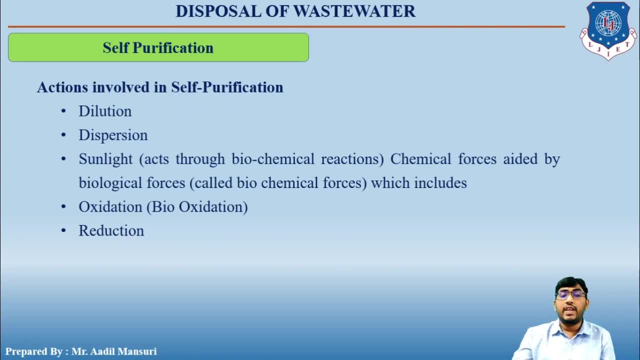 They in turn become food for tiny fishes, which become food for man. So the man discharges his waste back into the stream. Thus the natural cycle of self-purification continues and the river water regains its original quality. 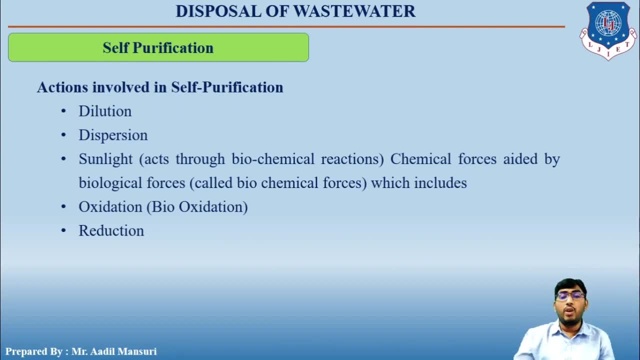 Now, the complete self-purification process is only possible if the concentration of pollutants is less than the total amount of oxygen that is released from the atmosphere. So the self-purification process is only possible if the concentration of pollutants is less than the total amount of oxygen that is released from the atmosphere. 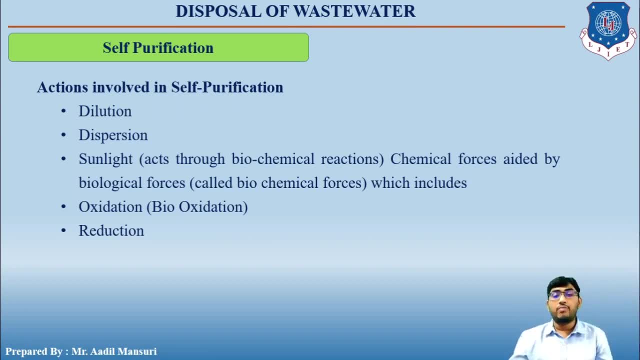 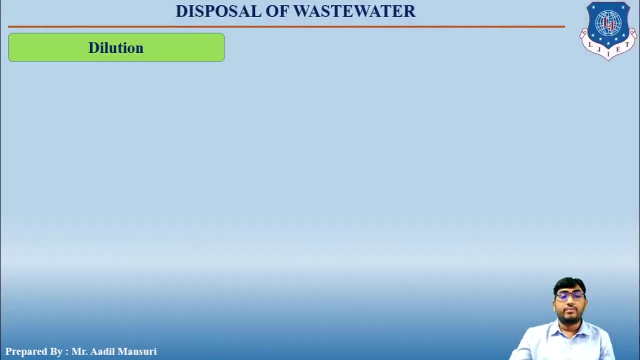 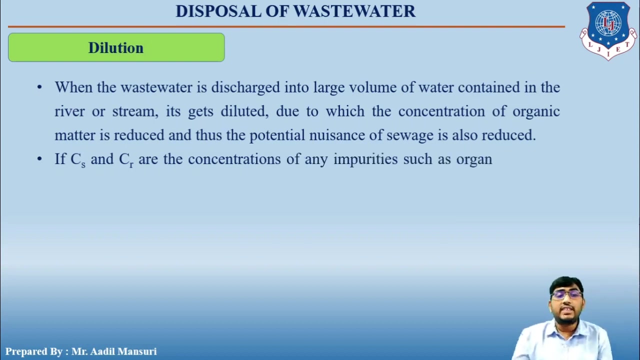 Thus, the self-purification process is only possible if the concentration of pollutants is less than the total amount of oxygen that is released from the atmosphere. Thus, the self-purification process is only possible if the concentration of pollutants is less than the total amount of oxygen that is released from the atmosphere. 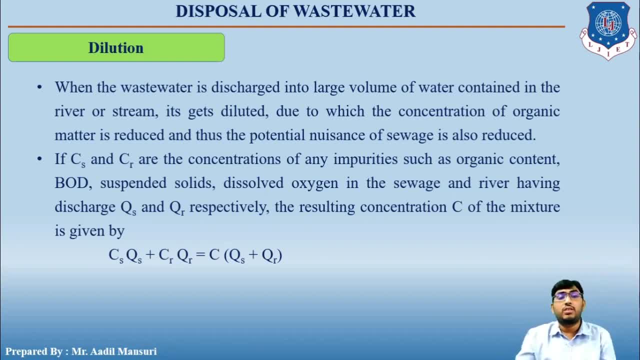 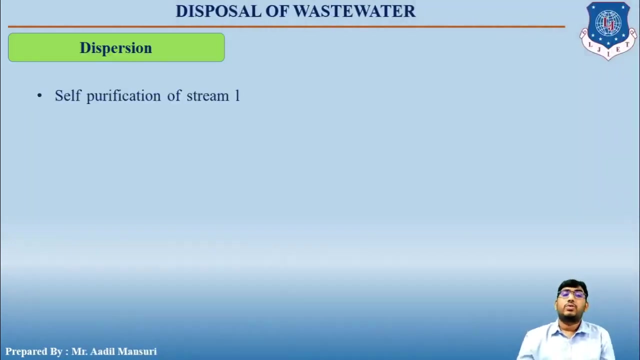 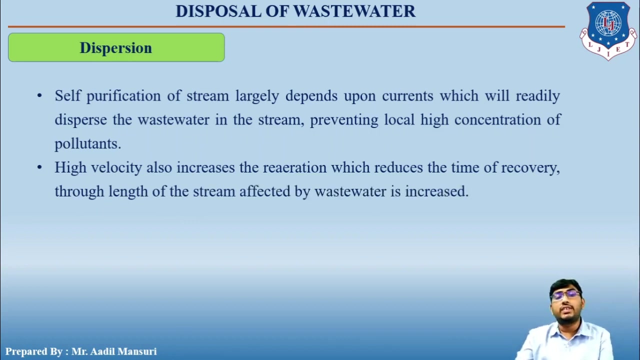 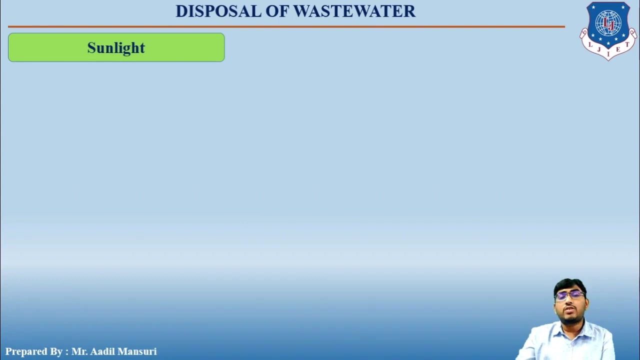 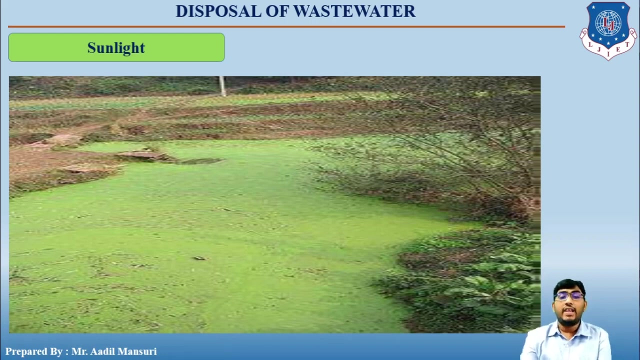 Thus, the self-purification process is only possible if the concentration of pollutants is less than the total amount of oxygen that is released from the atmosphere. Thus, the self-purification process is only possible if the concentration of pollutants is less than the total amount of oxygen that is released from the atmosphere. 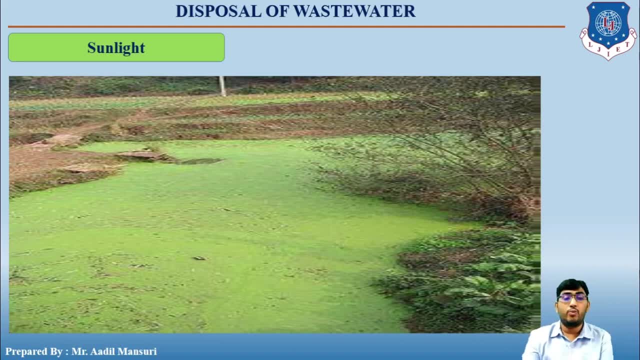 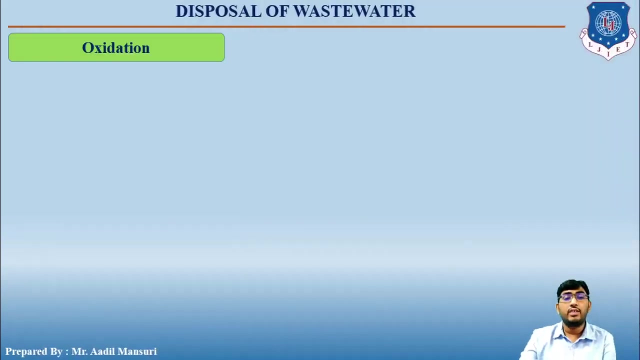 Thus, the self-purification process is only possible if the concentration of pollutants is less than the total amount of oxygen that is released from the atmosphere. Thus, the self-purification process is only possible if the concentration of pollutants is less than the total amount of oxygen that is released from the atmosphere. 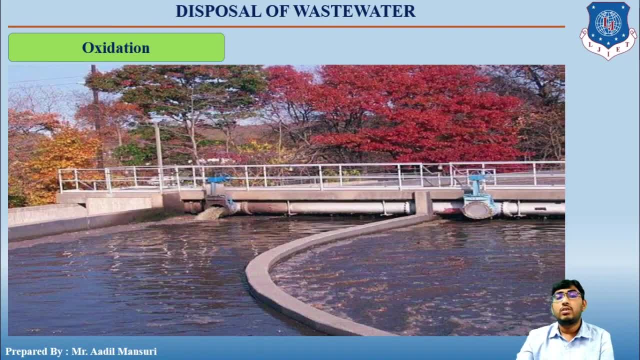 Thus, the self-purification process is only possible if the concentration of pollutants is less than the total amount of oxygen that is released from the atmosphere. Thus, the self-purification process is only possible if the concentration of pollutants is less than the total amount of oxygen that is released from the atmosphere. 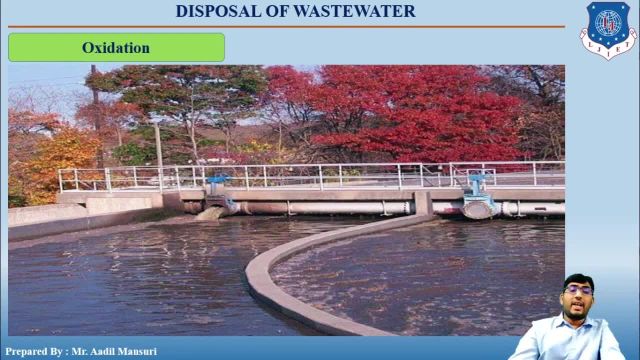 Thus, the self-purification process is only possible if the concentration of pollutants is less than the total amount of oxygen that is released from the atmosphere. Thus, the self-purification process is only possible if the concentration of pollutants is less than the total amount of oxygen that is released from the atmosphere. 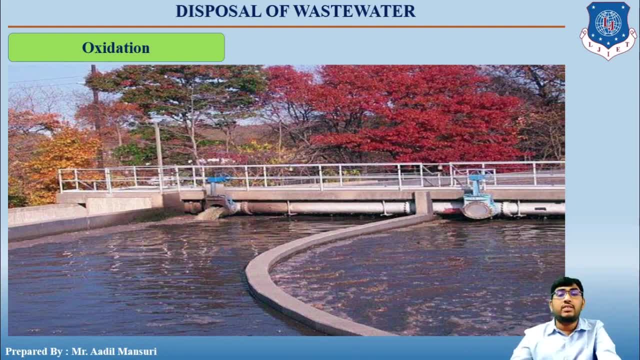 Thus, the self-purification process is only possible if the concentration of pollutants is less than the total amount of oxygen that is released from the atmosphere. Thus, the self-purification process is only possible if the concentration of pollutants is less than the total amount of oxygen that is released from the atmosphere. 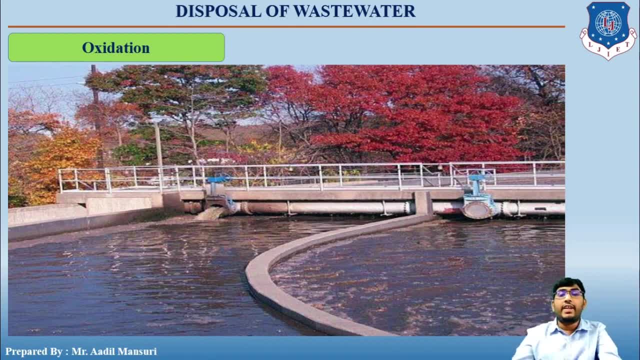 Thus, the self-purification process is only possible if the concentration of pollutants is less than the total amount of oxygen that is released from the atmosphere. Thus, the self-purification process is only possible if the concentration of pollutants is less than the total amount of oxygen that is released from the atmosphere. 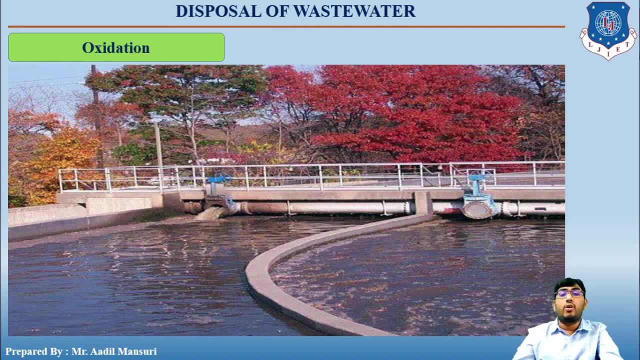 Thus, the self-purification process is only possible if the concentration of pollutants is less than the total amount of oxygen that is released from the atmosphere. Thus, the self-purification process is only possible if the concentration of pollutants is less than the total amount of oxygen that is released from the atmosphere. 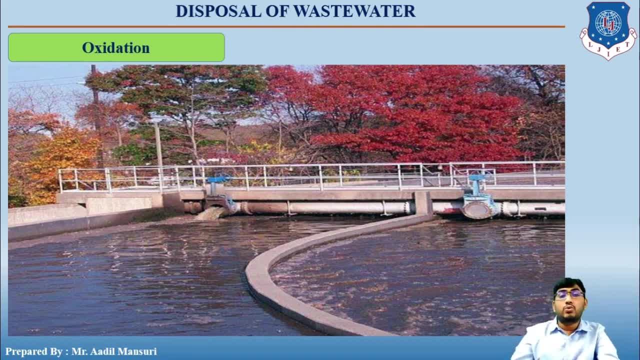 Thus, the self-purification process is only possible if the concentration of pollutants is less than the total amount of oxygen that is released from the atmosphere. Thus, the self-purification process is only possible if the concentration of pollutants is less than the total amount of oxygen that is released from the atmosphere. 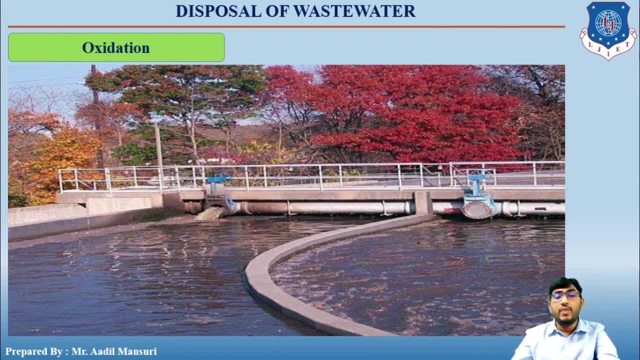 Thus, the self-purification process is only possible if the concentration of pollutants is less than the total amount of oxygen that is released from the atmosphere. Thus, the self-purification process is only possible if the concentration of pollutants is less than the total amount of oxygen that is released from the atmosphere. 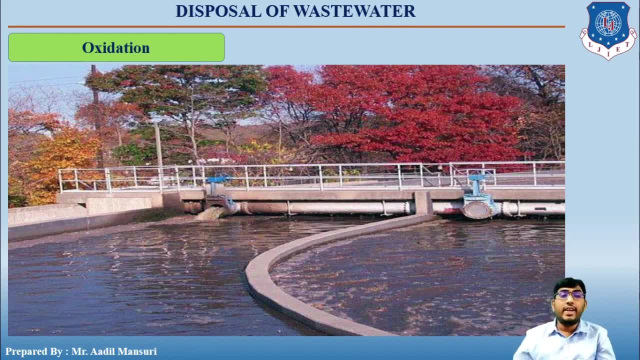 Thus, the self-purification process is only possible if the concentration of pollutants is less than the total amount of oxygen that is released from the atmosphere. Thus, the self-purification process is only possible if the concentration of pollutants is less than the total amount of oxygen that is released from the atmosphere. 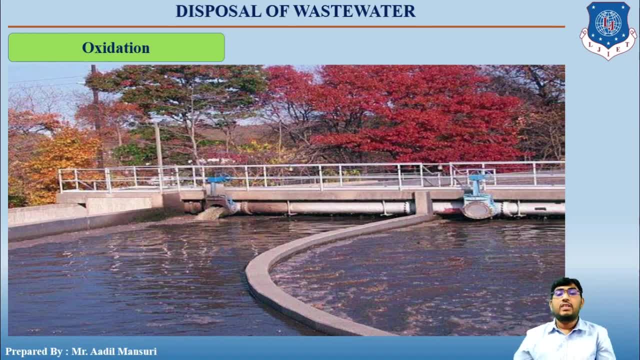 Thus, the self-purification process is only possible if the concentration of pollutants is less than the total amount of oxygen that is released from the atmosphere. Thus, the self-purification process is only possible if the concentration of pollutants is less than the total amount of oxygen that is released from the atmosphere. 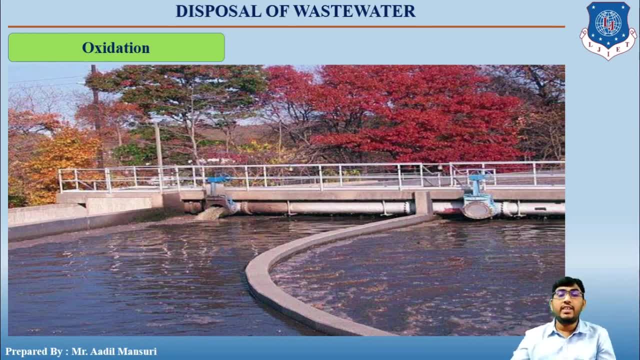 Thus, the self-purification process is only possible if the concentration of pollutants is less than the total amount of oxygen that is released from the atmosphere. Thus, the self-purification process is only possible if the concentration of pollutants is less than the total amount of oxygen that is released from the atmosphere. 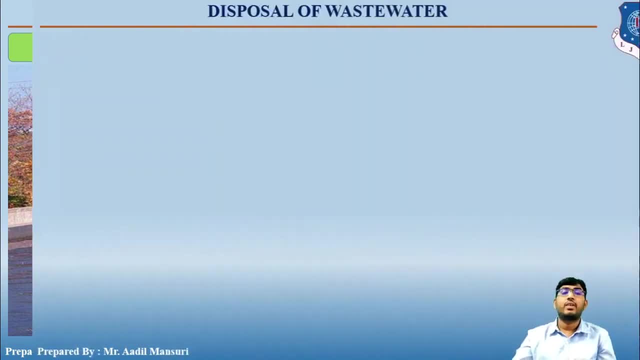 Thus, the self-purification process is only possible if the concentration of pollutants is less than the total amount of oxygen that is released from the atmosphere. Thus, the self-purification process is only possible if the concentration of pollutants is less than the total amount of oxygen that is released from the atmosphere. 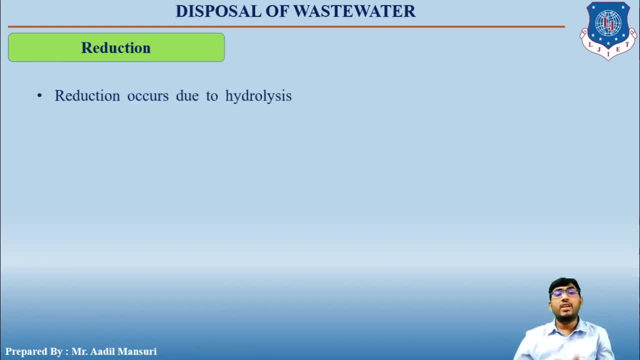 Thus, the self-purification process is only possible if the concentration of pollutants is less than the total amount of oxygen that is released from the atmosphere. Thus, the self-purification process is only possible if the concentration of pollutants is less than the total amount of oxygen that is released from the atmosphere. 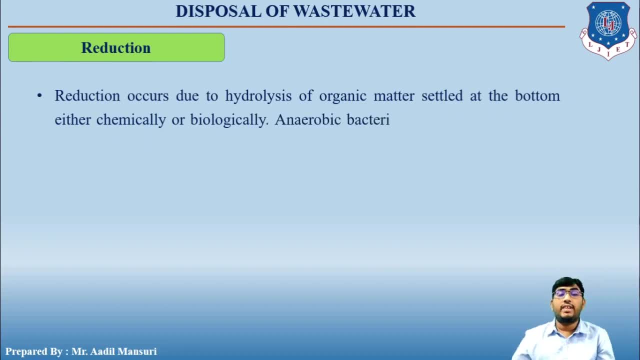 Thus, the self-purification process is only possible if the concentration of pollutants is less than the total amount of oxygen that is released from the atmosphere. Thus, the self-purification process is only possible if the concentration of pollutants is less than the total amount of oxygen that is released from the atmosphere. 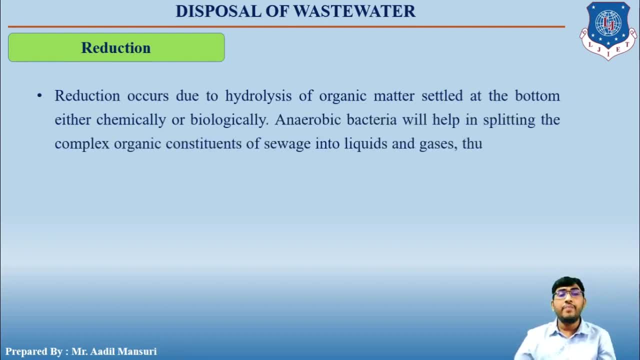 Thus, the self-purification process is only possible if the concentration of pollutants is less than the total amount of oxygen that is released from the atmosphere. Thus, the self-purification process is only possible if the concentration of pollutants is less than the total amount of oxygen that is released from the atmosphere. 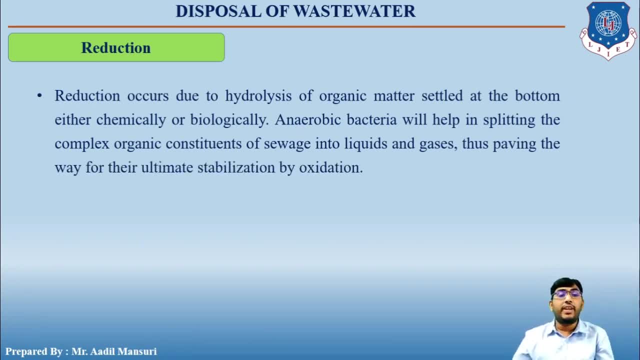 Thus, the self-purification process is only possible if the concentration of pollutants is less than the total amount of oxygen that is released from the atmosphere. Thus, the self-purification process is only possible if the concentration of pollutants is less than the total amount of oxygen that is released from the atmosphere. 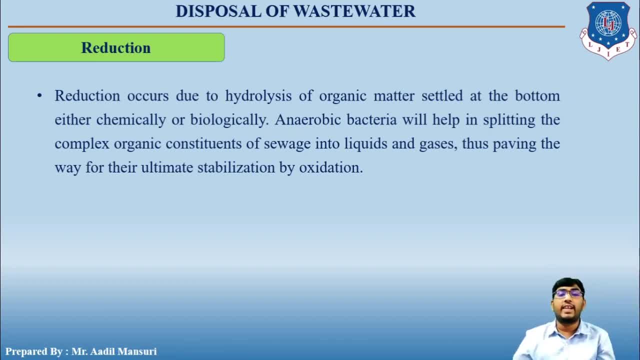 Thus, the self-purification process is only possible if the concentration of pollutants is less than the total amount of oxygen that is released from the atmosphere. Thus, the self-purification process is only possible if the concentration of pollutants is less than the total amount of oxygen that is released from the atmosphere. 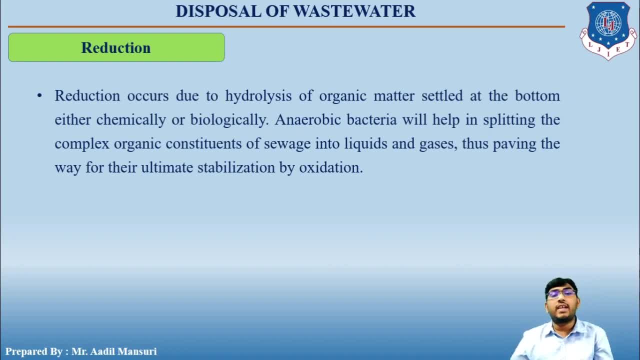 Thus, the self-purification process is only possible if the concentration of pollutants is less than the total amount of oxygen that is released from the atmosphere. Thus, the self-purification process is only possible if the concentration of pollutants is less than the total amount of oxygen that is released from the atmosphere. 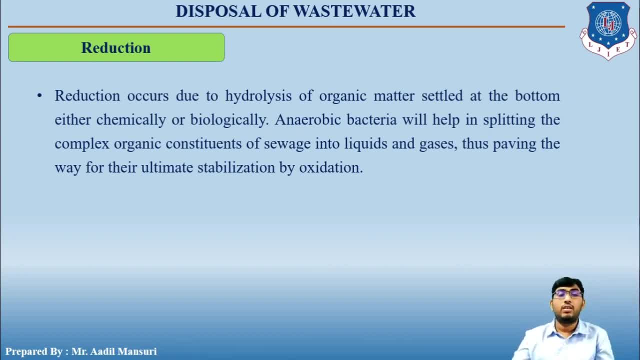 Thus, the self-purification process is only possible if the concentration of pollutants is less than the total amount of oxygen that is released from the atmosphere. Thus, the self-purification process is only possible if the concentration of pollutants is less than the total amount of oxygen that is released from the atmosphere. 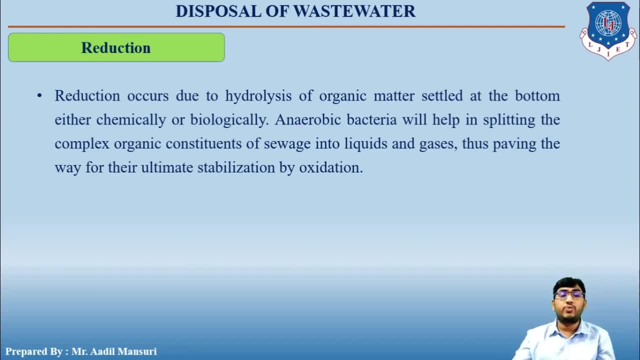 Thus, the self-purification process is only possible if the concentration of pollutants is less than the total amount of oxygen that is released from the atmosphere. Thus, the self-purification process is only possible if the concentration of pollutants is less than the total amount of oxygen that is released from the atmosphere. 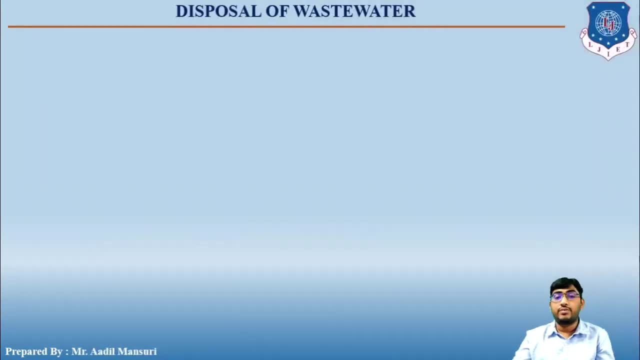 Thus, the self-purification process is only possible if the concentration of pollutants is less than the total amount of oxygen that is released from the atmosphere. Thus, the self-purification process is only possible if the concentration of pollutants is less than the total amount of oxygen that is released from the atmosphere. 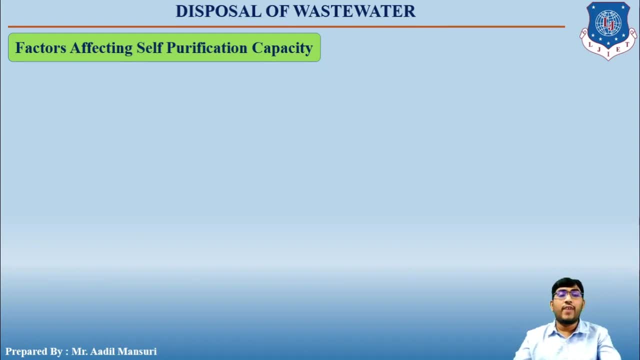 Thus, the self-purification process is only possible if the concentration of pollutants is less than the total amount of oxygen that is released from the atmosphere. Thus, the self-purification process is only possible if the concentration of pollutants is less than the total amount of oxygen that is released from the atmosphere. 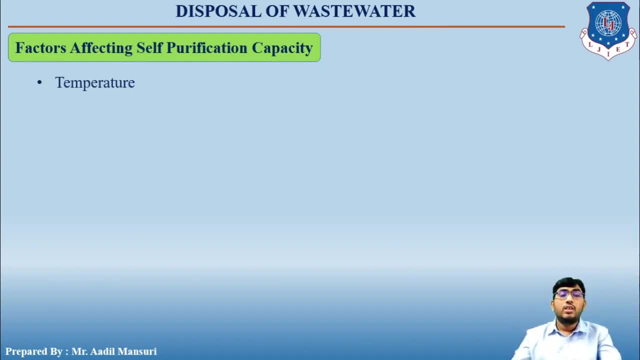 Thus, the self-purification process is only possible if the concentration of pollutants is less than the total amount of oxygen that is released from the atmosphere. Thus, the self-purification process is only possible if the concentration of pollutants is less than the total amount of oxygen that is released from the atmosphere. 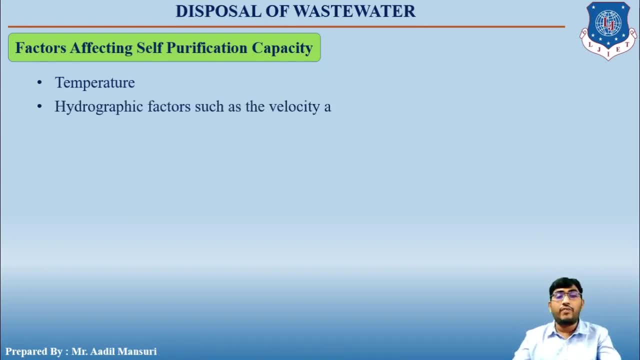 Thus, the self-purification process is only possible if the concentration of pollutants is less than the total amount of oxygen that is released from the atmosphere. Thus, the self-purification process is only possible if the concentration of pollutants is less than the total amount of oxygen that is released from the atmosphere. 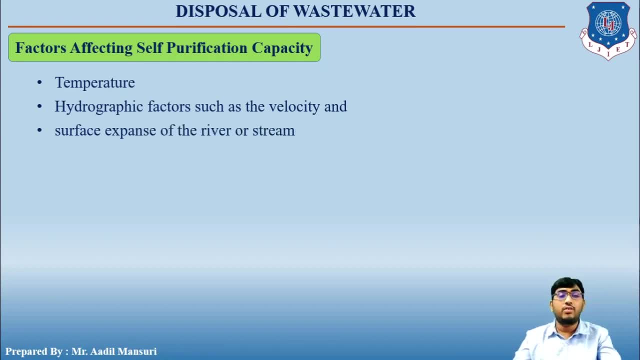 Thus, the self-purification process is only possible if the concentration of pollutants is less than the total amount of oxygen that is released from the atmosphere. Thus, the self-purification process is only possible if the concentration of pollutants is less than the total amount of oxygen that is released from the atmosphere. 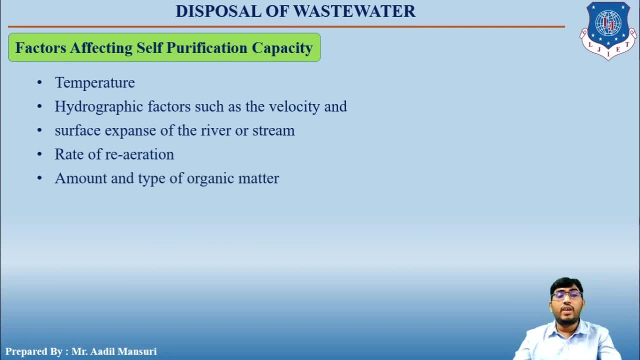 Thus, the self-purification process is only possible if the concentration of pollutants is less than the total amount of oxygen that is released from the atmosphere. Thus, the self-purification process is only possible if the concentration of pollutants is less than the total amount of oxygen that is released from the atmosphere. 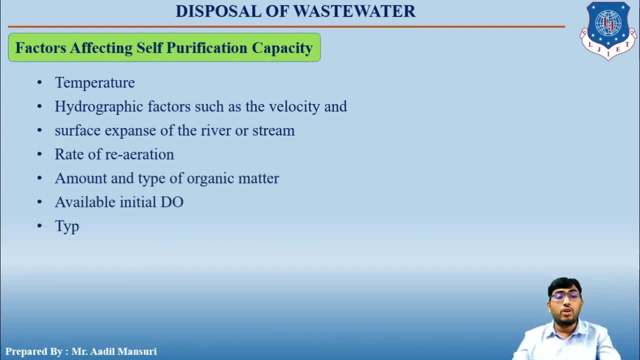 Thus, the self-purification process is only possible if the concentration of pollutants is less than the total amount of oxygen that is released from the atmosphere. Thus, the self-purification process is only possible if the concentration of pollutants is less than the total amount of oxygen that is released from the atmosphere. 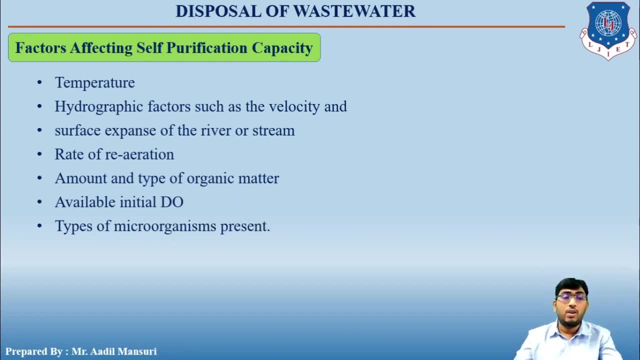 Thus, the self-purification process is only possible if the concentration of pollutants is less than the total amount of oxygen that is released from the atmosphere. Thus, the self-purification process is only possible if the concentration of pollutants is less than the total amount of oxygen that is released from the atmosphere. 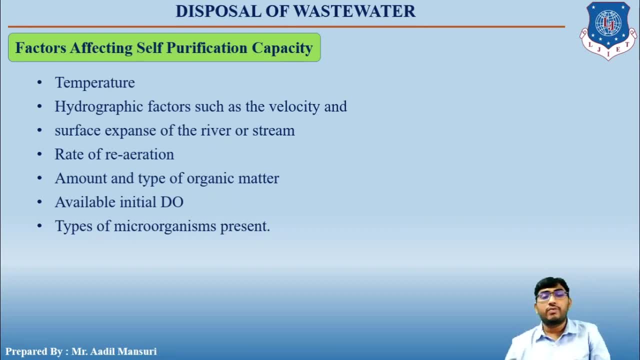 Thus, the self-purification process is only possible if the concentration of pollutants is less than the total amount of oxygen that is released from the atmosphere. Thus, the self-purification process is only possible if the concentration of pollutants is less than the total amount of oxygen that is released from the atmosphere. 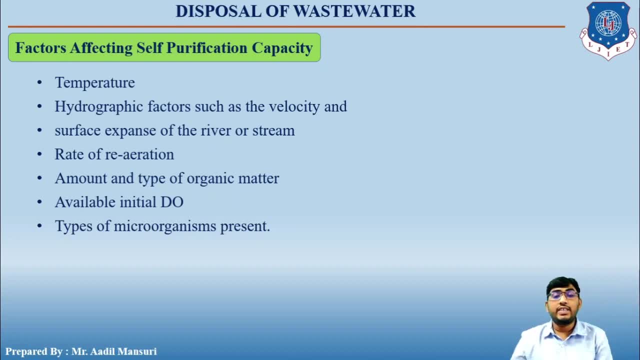 Thus, the self-purification process is only possible if the concentration of pollutants is less than the total amount of oxygen that is released from the atmosphere. Thus, the self-purification process is only possible if the concentration of pollutants is less than the total amount of oxygen that is released from the atmosphere. 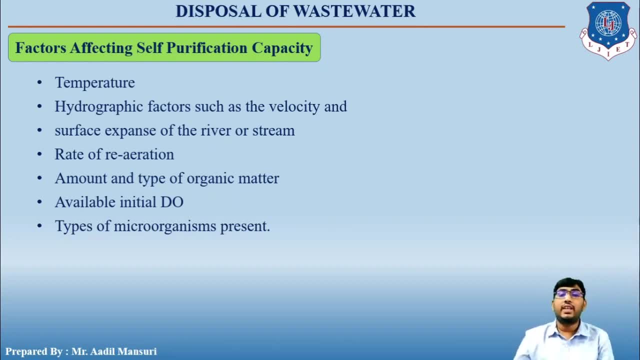 Thus, the self-purification process is only possible if the concentration of pollutants is less than the total amount of oxygen that is released from the atmosphere. Thus, the self-purification process is only possible if the concentration of pollutants is less than the total amount of oxygen that is released from the atmosphere. 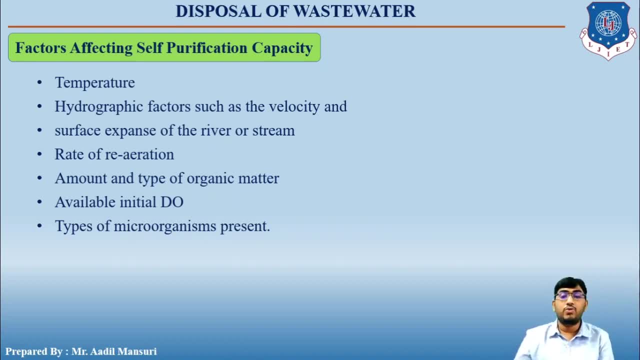 Thus, the self-purification process is only possible if the concentration of pollutants is less than the total amount of oxygen that is released from the atmosphere. Thus, the self-purification process is only possible if the concentration of pollutants is less than the total amount of oxygen that is released from the atmosphere. 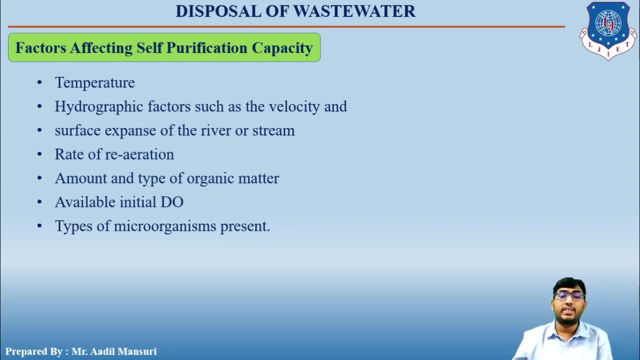 Thus, the self-purification process is only possible if the concentration of pollutants is less than the total amount of oxygen that is released from the atmosphere. Thus, the self-purification process is only possible if the concentration of pollutants is less than the total amount of oxygen that is released from the atmosphere. 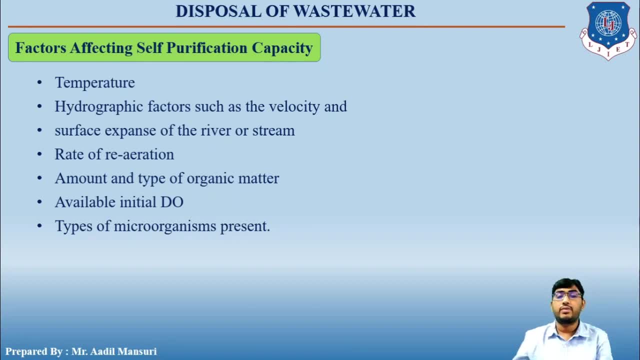 Thus, the self-purification process is only possible if the concentration of pollutants is less than the total amount of oxygen that is released from the atmosphere. Thus, the self-purification process is only possible if the concentration of pollutants is less than the total amount of oxygen that is released from the atmosphere. 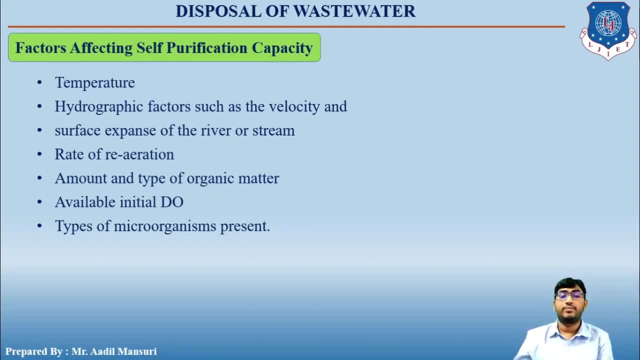 Thus, the self-purification process is only possible if the concentration of pollutants is less than the total amount of oxygen that is released from the atmosphere. Thus, the self-purification process is only possible if the concentration of pollutants is less than the total amount of oxygen that is released from the atmosphere. 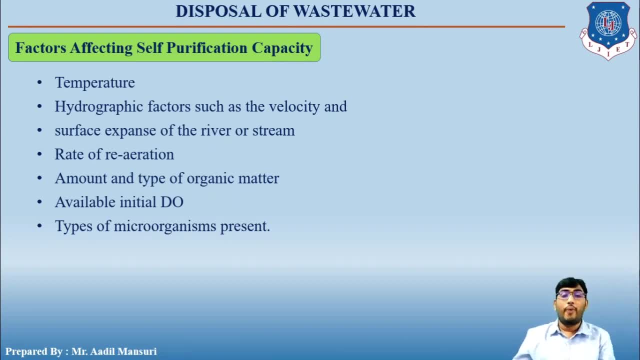 Thus, the self-purification process is only possible if the concentration of pollutants is less than the total amount of oxygen that is released from the atmosphere. Thus, the self-purification process is only possible if the concentration of pollutants is less than the total amount of oxygen that is released from the atmosphere. 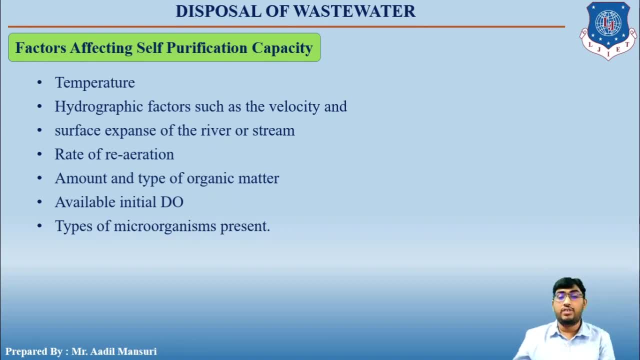 Thus, the self-purification process is only possible if the concentration of pollutants is less than the total amount of oxygen that is released from the atmosphere. Thus, the self-purification process is only possible if the concentration of pollutants is less than the total amount of oxygen that is released from the atmosphere. 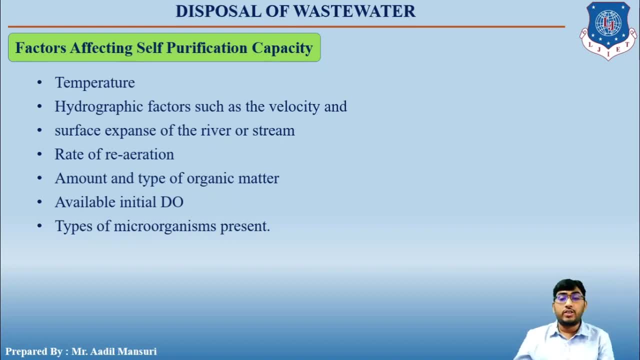 Thus, the self-purification process is only possible if the concentration of pollutants is less than the total amount of oxygen that is released from the atmosphere. Thus, the self-purification process is only possible if the concentration of pollutants is less than the total amount of oxygen that is released from the atmosphere. 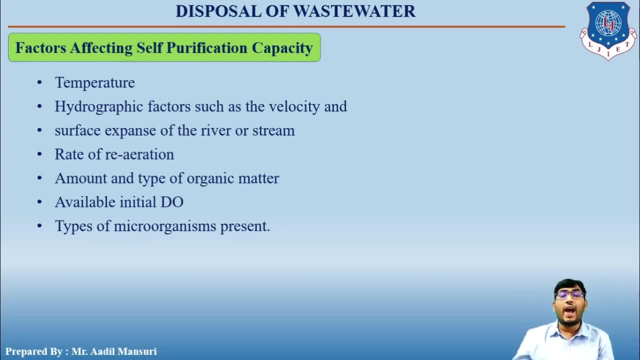 Thus, the self-purification process is only possible if the concentration of pollutants is less than the total amount of oxygen that is released from the atmosphere. Thus, the self-purification process is only possible if the concentration of pollutants is less than the total amount of oxygen that is released from the atmosphere. 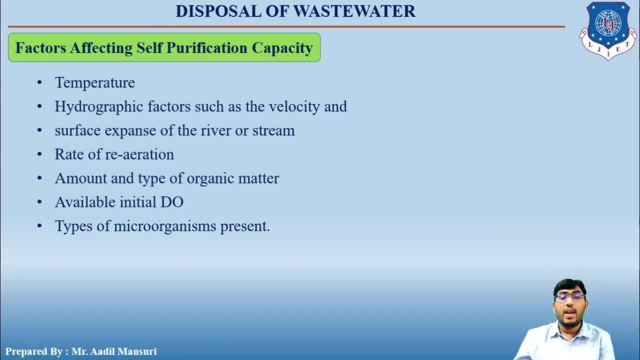 Thus, the self-purification process is only possible if the concentration of pollutants is less than the total amount of oxygen that is released from the atmosphere. Thus, the self-purification process is only possible if the concentration of pollutants is less than the total amount of oxygen that is released from the atmosphere. 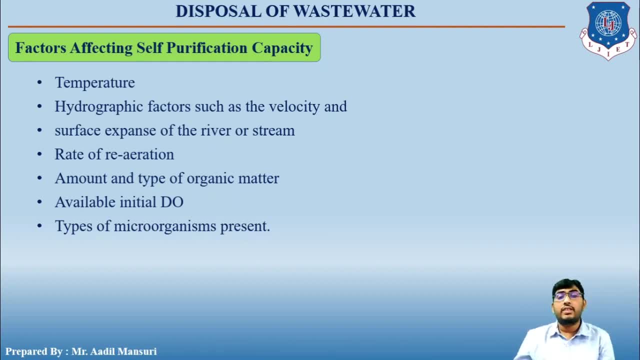 Thus, the self-purification process is only possible if the concentration of pollutants is less than the total amount of oxygen that is released from the atmosphere. Thus, the self-purification process is only possible if the concentration of pollutants is less than the total amount of oxygen that is released from the atmosphere. 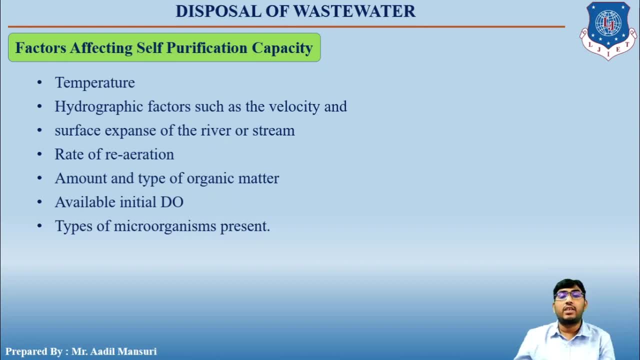 Thus, the self-purification process is only possible if the concentration of pollutants is less than the total amount of oxygen that is released from the atmosphere. Thus, the self-purification process is only possible if the concentration of pollutants is less than the total amount of oxygen that is released from the atmosphere. 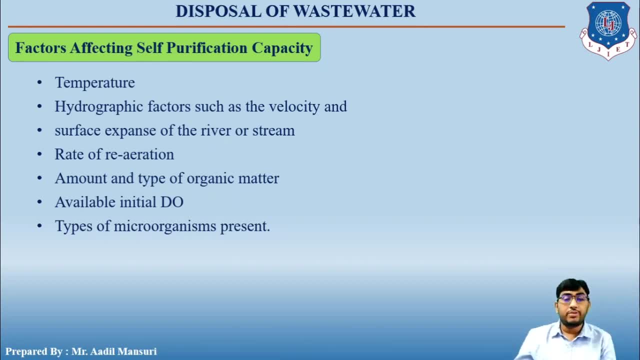 Thus, the self-purification process is only possible if the concentration of pollutants is less than the total amount of oxygen that is released from the atmosphere. Thus, the self-purification process is only possible if the concentration of pollutants is less than the total amount of oxygen that is released from the atmosphere. 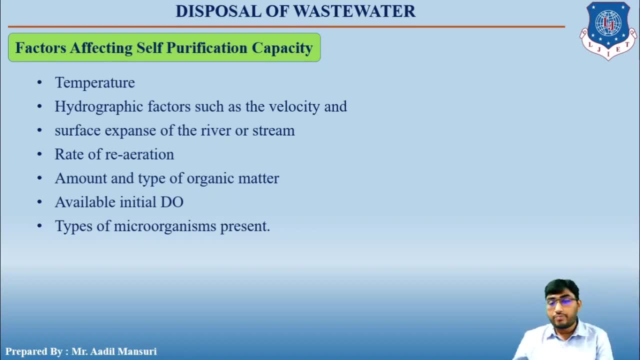 Thus, the self-purification process is only possible if the concentration of pollutants is less than the total amount of oxygen that is released from the atmosphere. Thus, the self-purification process is only possible if the concentration of pollutants is less than the total amount of oxygen that is released from the atmosphere. 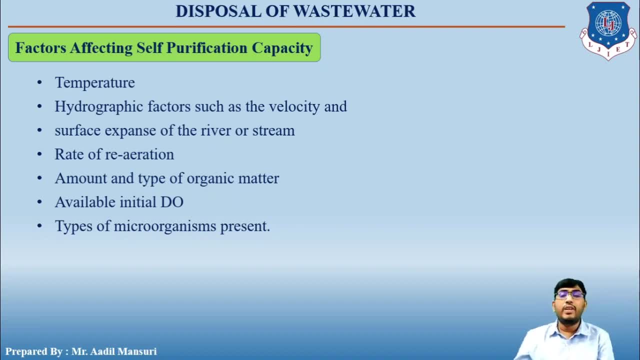 Thus, the self-purification process is only possible if the concentration of pollutants is less than the total amount of oxygen that is released from the atmosphere. Thus, the self-purification process is only possible if the concentration of pollutants is less than the total amount of oxygen that is released from the atmosphere. 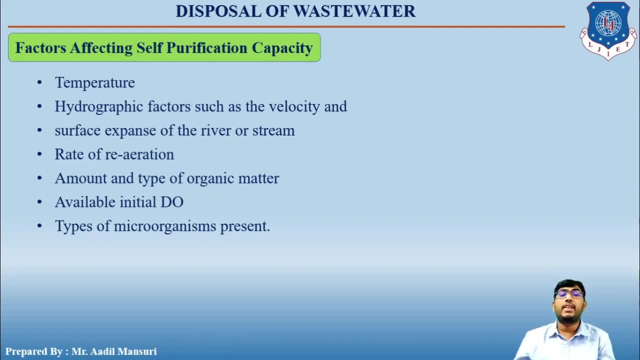 Thus, the self-purification process is only possible if the concentration of pollutants is less than the total amount of oxygen that is released from the atmosphere. Thus, the self-purification process is only possible if the concentration of pollutants is less than the total amount of oxygen that is released from the atmosphere. 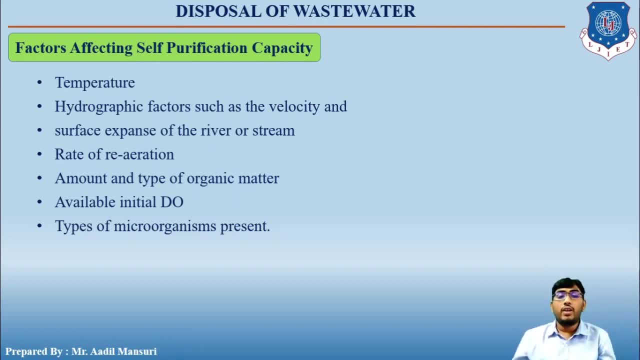 Thus, the self-purification process is only possible if the concentration of pollutants is less than the total amount of oxygen that is released from the atmosphere. Thus, the self-purification process is only possible if the concentration of pollutants is less than the total amount of oxygen that is released from the atmosphere. 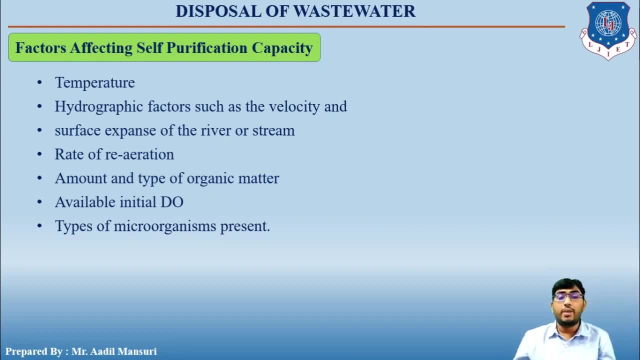 Thus, the self-purification process is only possible if the concentration of pollutants is less than the total amount of oxygen that is released from the atmosphere. Thus, the self-purification process is only possible if the concentration of pollutants is less than the total amount of oxygen that is released from the atmosphere. 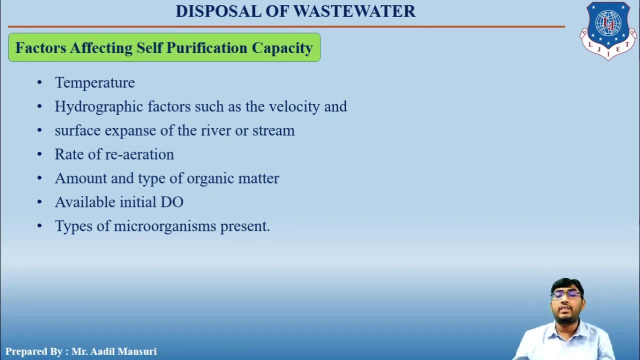 Thus, the self-purification process is only possible if the concentration of pollutants is less than the total amount of oxygen that is released from the atmosphere. Thus, the self-purification process is only possible if the concentration of pollutants is less than the total amount of oxygen that is released from the atmosphere. 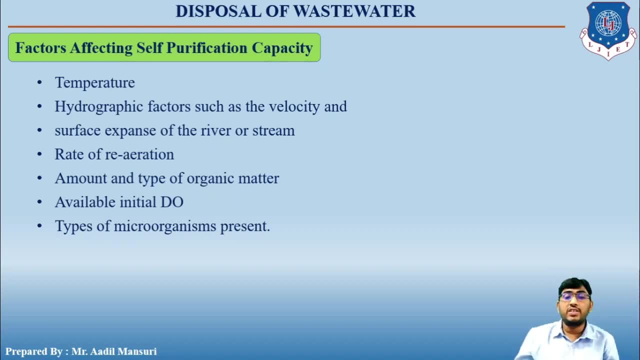 Thus, the self-purification process is only possible if the concentration of pollutants is less than the total amount of oxygen that is released from the atmosphere. Thus, the self-purification process is only possible if the concentration of pollutants is less than the total amount of oxygen that is released from the atmosphere. 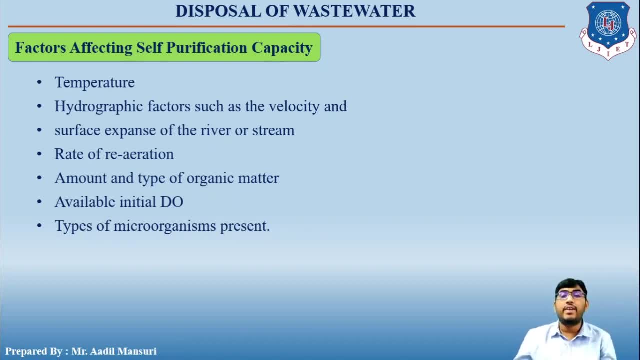 Thus, the self-purification process is only possible if the concentration of pollutants is less than the total amount of oxygen that is released from the atmosphere. Thus, the self-purification process is only possible if the concentration of pollutants is less than the total amount of oxygen that is released from the atmosphere. 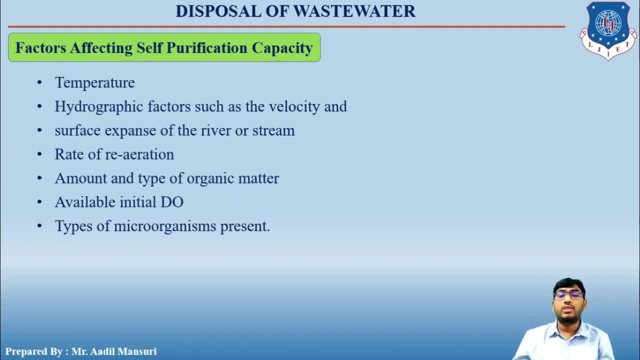 Thus, the self-purification process is only possible if the concentration of pollutants is less than the total amount of oxygen that is released from the atmosphere. Thus, the self-purification process is only possible if the concentration of pollutants is less than the total amount of oxygen that is released from the atmosphere. 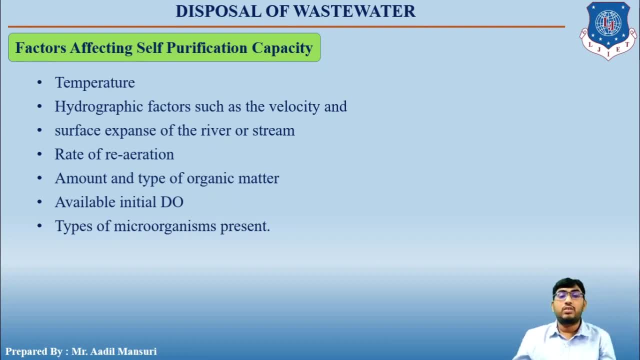 Thus, the self-purification process is only possible if the concentration of pollutants is less than the total amount of oxygen that is released from the atmosphere. Thus, the self-purification process is only possible if the concentration of pollutants is less than the total amount of oxygen that is released from the atmosphere. 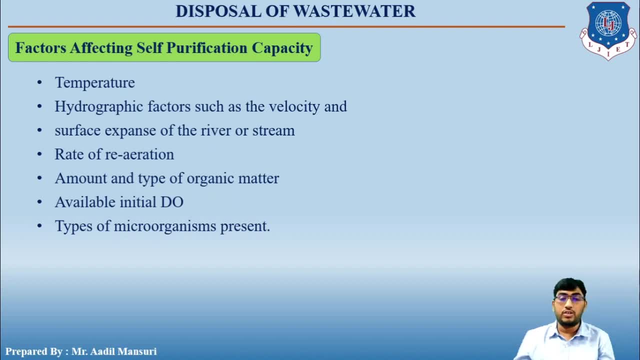 Thus, the self-purification process is only possible if the concentration of pollutants is less than the total amount of oxygen that is released from the atmosphere. Thus, the self-purification process is only possible if the concentration of pollutants is less than the total amount of oxygen that is released from the atmosphere. 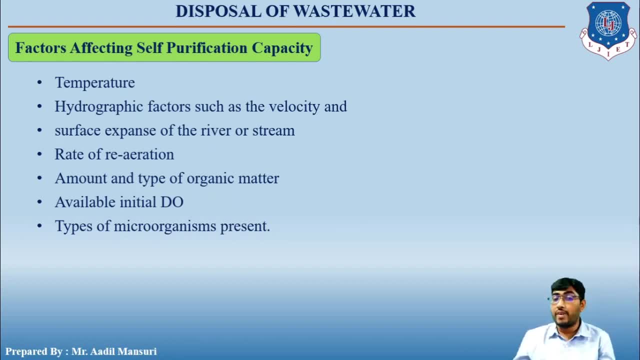 Thus, the self-purification process is only possible if the concentration of pollutants is less than the total amount of oxygen that is released from the atmosphere. Thus, the self-purification process is only possible if the concentration of pollutants is less than the total amount of oxygen that is released from the atmosphere. 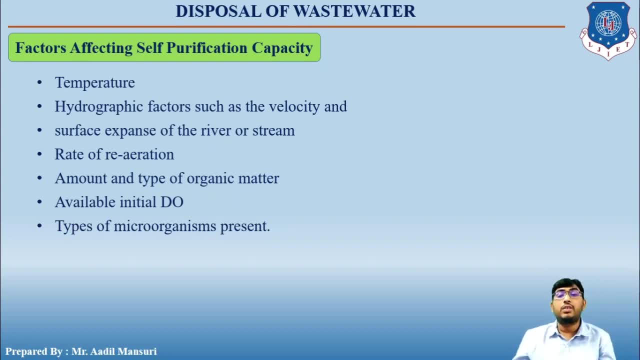 Thus, the self-purification process is only possible if the concentration of pollutants is less than the total amount of oxygen that is released from the atmosphere. Thus, the self-purification process is only possible if the concentration of pollutants is less than the total amount of oxygen that is released from the atmosphere. 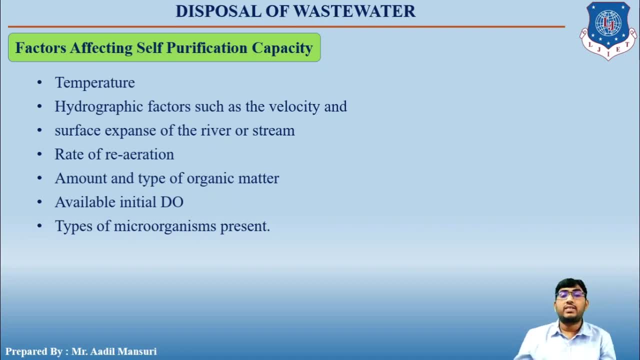 Thus, the self-purification process is only possible if the concentration of pollutants is less than the total amount of oxygen that is released from the atmosphere. Thus, the self-purification process is only possible if the concentration of pollutants is less than the total amount of oxygen that is released from the atmosphere. 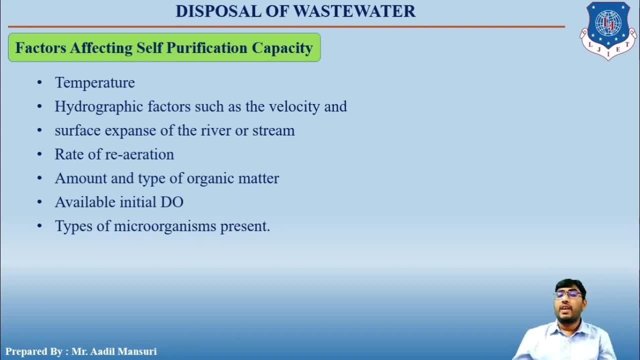 Thus, the self-purification process is only possible if the concentration of pollutants is less than the total amount of oxygen that is released from the atmosphere. Thus, the self-purification process is only possible if the concentration of pollutants is less than the total amount of oxygen that is released from the atmosphere. 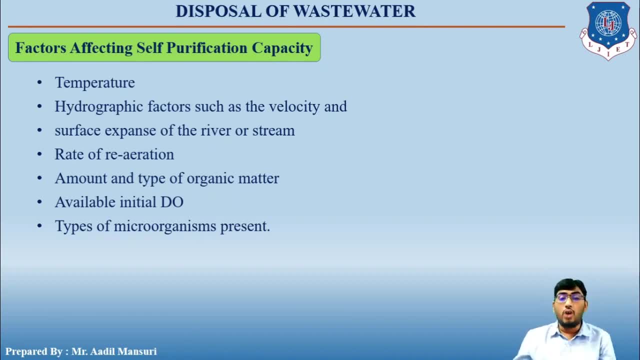 Thus, the self-purification process is only possible if the concentration of pollutants is less than the total amount of oxygen that is released from the atmosphere. Thus, the self-purification process is only possible if the concentration of pollutants is less than the total amount of oxygen that is released from the atmosphere. 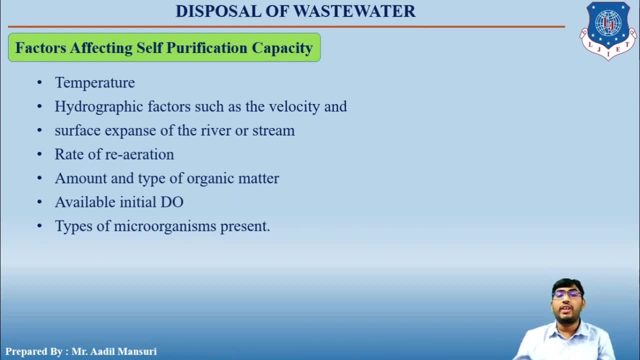 Thus, the self-purification process is only possible if the concentration of pollutants is less than the total amount of oxygen that is released from the atmosphere. Thus, the self-purification process is only possible if the concentration of pollutants is less than the total amount of oxygen that is released from the atmosphere. 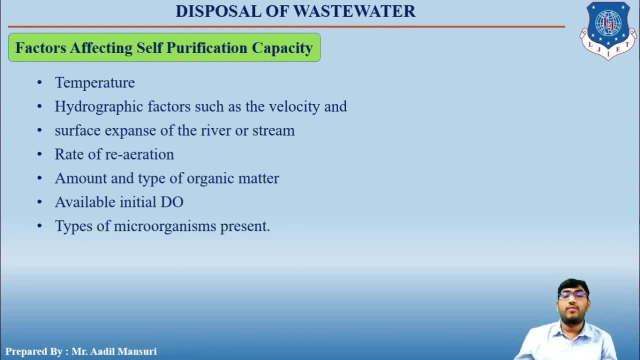 Thus, the self-purification process is only possible if the concentration of pollutants is less than the total amount of oxygen that is released from the atmosphere. Thus, the self-purification process is only possible if the concentration of pollutants is less than the total amount of oxygen that is released from the atmosphere. 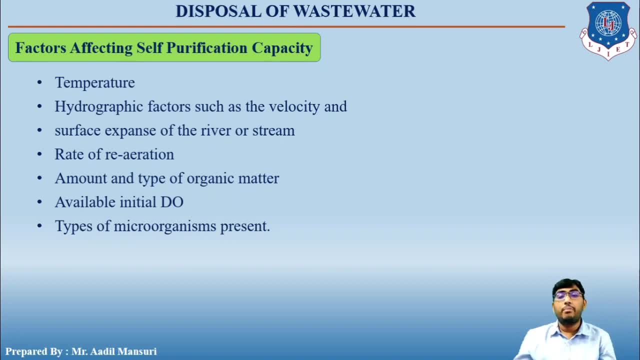 Thus, the self-purification process is only possible if the concentration of pollutants is less than the total amount of oxygen that is released from the atmosphere. Thus, the self-purification process is only possible if the concentration of pollutants is less than the total amount of oxygen that is released from the atmosphere. 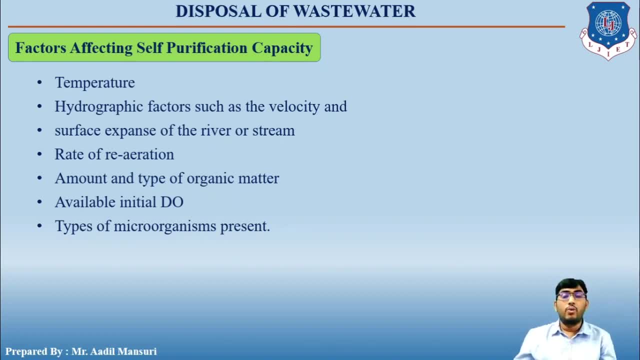 Thus, the self-purification process is only possible if the concentration of pollutants is less than the total amount of oxygen that is released from the atmosphere. Thus, the self-purification process is only possible if the concentration of pollutants is less than the total amount of oxygen that is released from the atmosphere. 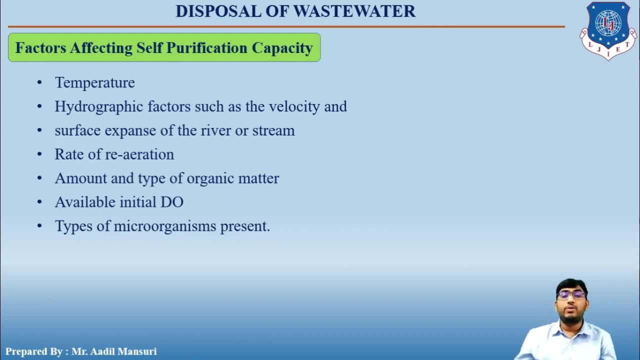 Thus, the self-purification process is only possible if the concentration of pollutants is less than the total amount of oxygen that is released from the atmosphere. Thus, the self-purification process is only possible if the concentration of pollutants is less than the total amount of oxygen that is released from the atmosphere. 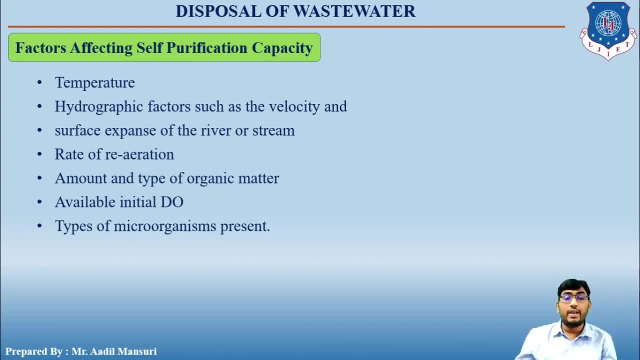 Thus, the self-purification process is only possible if the concentration of pollutants is less than the total amount of oxygen that is released from the atmosphere. Thus, the self-purification process is only possible if the concentration of pollutants is less than the total amount of oxygen that is released from the atmosphere. 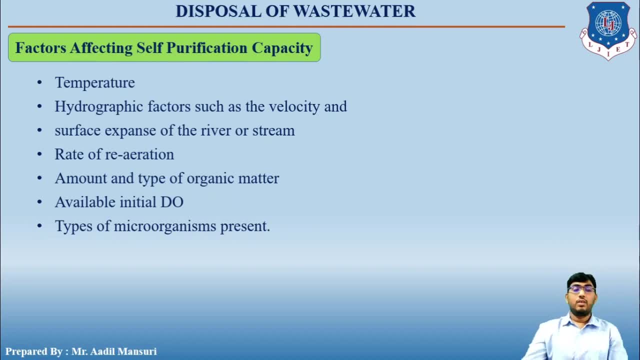 Thus, the self-purification process is only possible if the concentration of pollutants is less than the total amount of oxygen that is released from the atmosphere. Thus, the self-purification process is only possible if the concentration of pollutants is less than the total amount of oxygen that is released from the atmosphere. 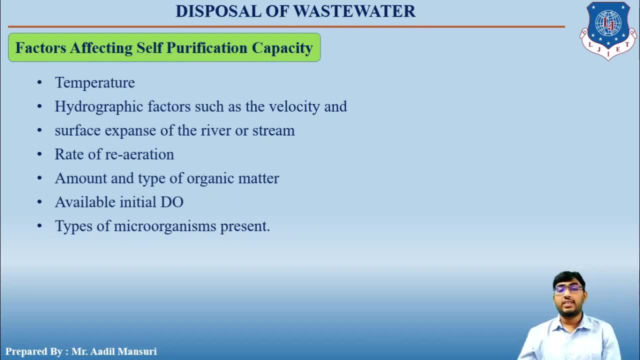 Thus, the self-purification process is only possible if the concentration of pollutants is less than the total amount of oxygen that is released from the atmosphere. Thus, the self-purification process is only possible if the concentration of pollutants is less than the total amount of oxygen that is released from the atmosphere. 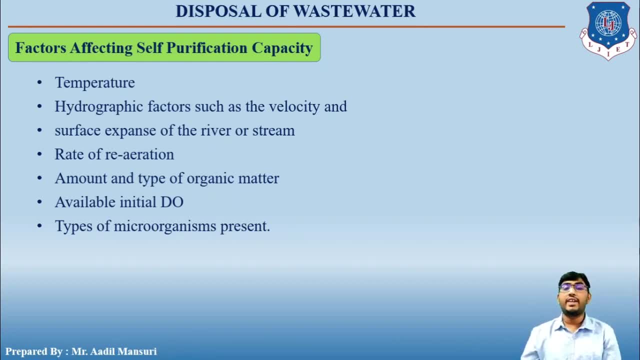 Thus, the self-purification process is only possible if the concentration of pollutants is less than the total amount of oxygen that is released from the atmosphere. Thus, the self-purification process is only possible if the concentration of pollutants is less than the total amount of oxygen that is released from the atmosphere. 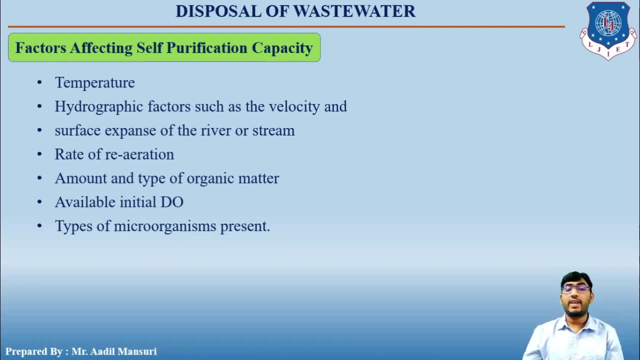 Thus, the self-purification process is only possible if the concentration of pollutants is less than the total amount of oxygen that is released from the atmosphere. Thus, the self-purification process is only possible if the concentration of pollutants is less than the total amount of oxygen that is released from the atmosphere. 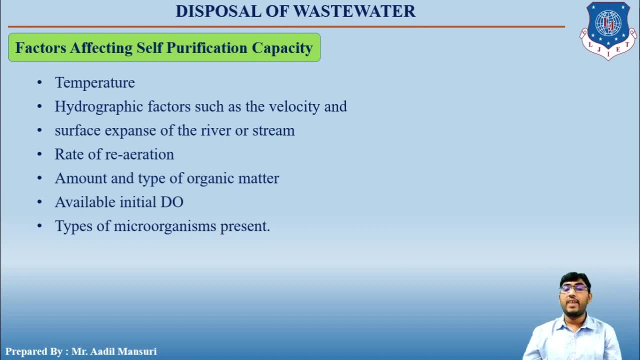 Thus, the self-purification process is only possible if the concentration of pollutants is less than the total amount of oxygen that is released from the atmosphere. Thus, the self-purification process is only possible if the concentration of pollutants is less than the total amount of oxygen that is released from the atmosphere. 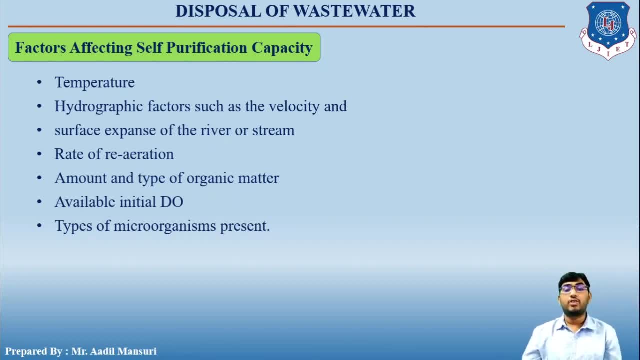 Thus, the self-purification process is only possible if the concentration of pollutants is less than the total amount of oxygen that is released from the atmosphere. Thus, the self-purification process is only possible if the concentration of pollutants is less than the total amount of oxygen that is released from the atmosphere. 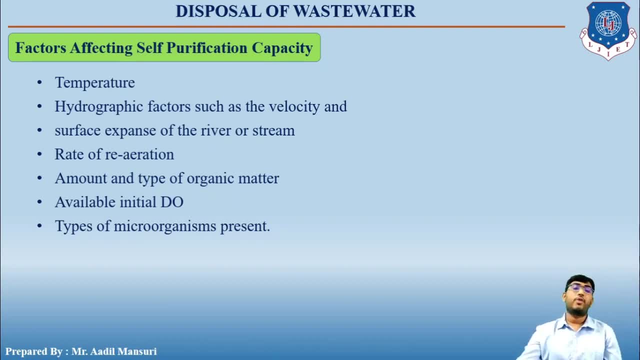 Thus, the self-purification process is only possible if the concentration of pollutants is less than the total amount of oxygen that is released from the atmosphere. Thus, the self-purification process is only possible if the concentration of pollutants is less than the total amount of oxygen that is released from the atmosphere. 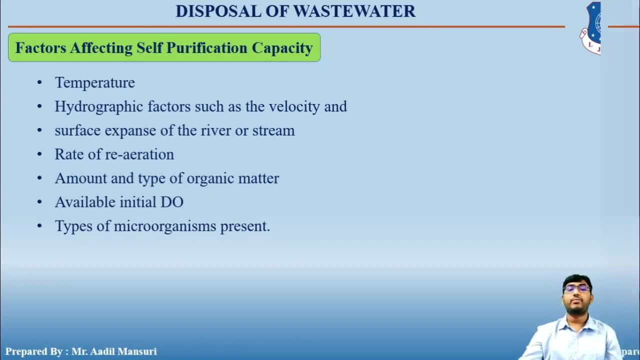 Thus, the self-purification process is only possible if the concentration of pollutants is less than the total amount of oxygen that is released from the atmosphere. Thus, the self-purification process is only possible if the concentration of pollutants is less than the total amount of oxygen that is released from the atmosphere. 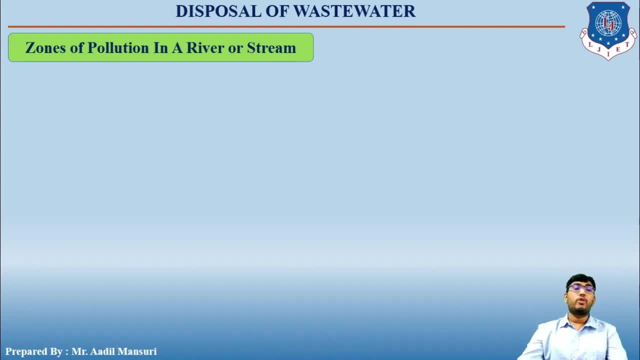 Thus, the self-purification process is only possible if the concentration of pollutants is less than the total amount of oxygen that is released from the atmosphere. Thus, the self-purification process is only possible if the concentration of pollutants is less than the total amount of oxygen that is released from the atmosphere. 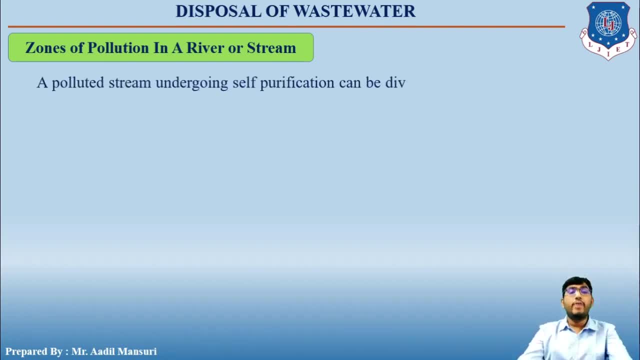 Thus, the self-purification process is only possible if the concentration of pollutants is less than the total amount of oxygen that is released from the atmosphere. Thus, the self-purification process is only possible if the concentration of pollutants is less than the total amount of oxygen that is released from the atmosphere. 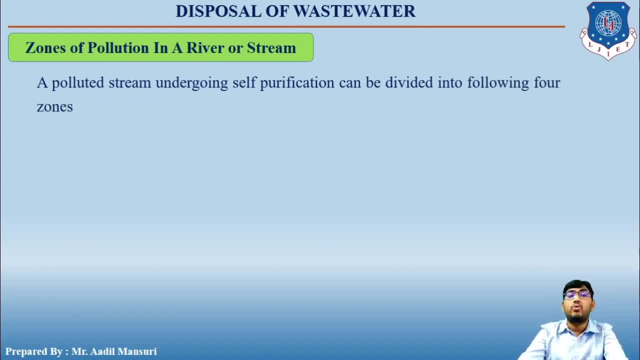 Thus, the self-purification process is only possible if the concentration of pollutants is less than the total amount of oxygen that is released from the atmosphere. Thus, the self-purification process is only possible if the concentration of pollutants is less than the total amount of oxygen that is released from the atmosphere. 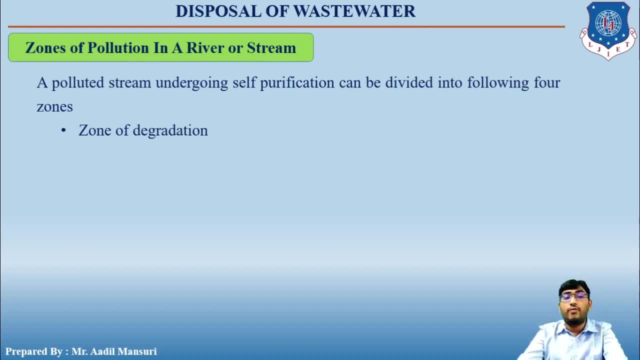 Thus, the self-purification process is only possible if the concentration of pollutants is less than the total amount of oxygen that is released from the atmosphere. Thus, the self-purification process is only possible if the concentration of pollutants is less than the total amount of oxygen that is released from the atmosphere. 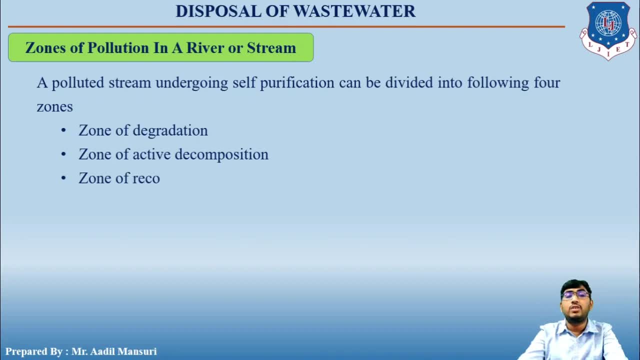 Thus, the self-purification process is only possible if the concentration of pollutants is less than the total amount of oxygen that is released from the atmosphere. Thus, the self-purification process is only possible if the concentration of pollutants is less than the total amount of oxygen that is released from the atmosphere. 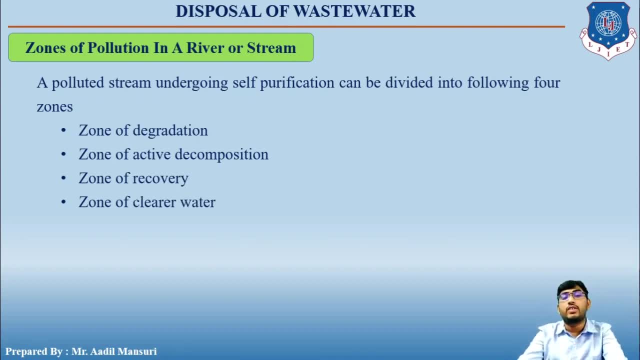 Thus, the self-purification process is only possible if the concentration of pollutants is less than the total amount of oxygen that is released from the atmosphere. Thus, the self-purification process is only possible if the concentration of pollutants is less than the total amount of oxygen that is released from the atmosphere. 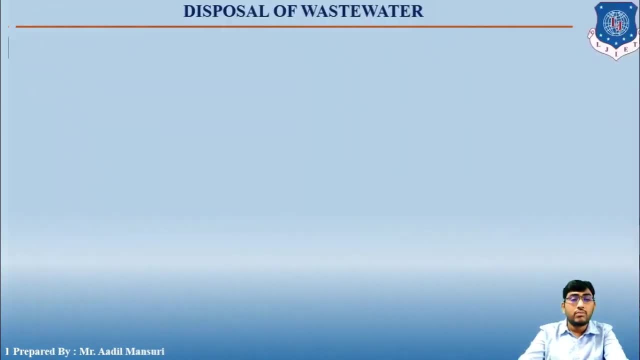 Thus, the self-purification process is only possible if the concentration of pollutants is less than the total amount of oxygen that is released from the atmosphere. Thus, the self-purification process is only possible if the concentration of pollutants is less than the total amount of oxygen that is released from the atmosphere. 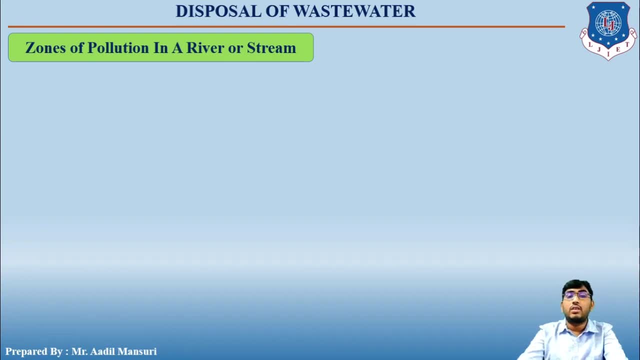 Thus, the self-purification process is only possible if the concentration of pollutants is less than the total amount of oxygen that is released from the atmosphere. Thus, the self-purification process is only possible if the concentration of pollutants is less than the total amount of oxygen that is released from the atmosphere. 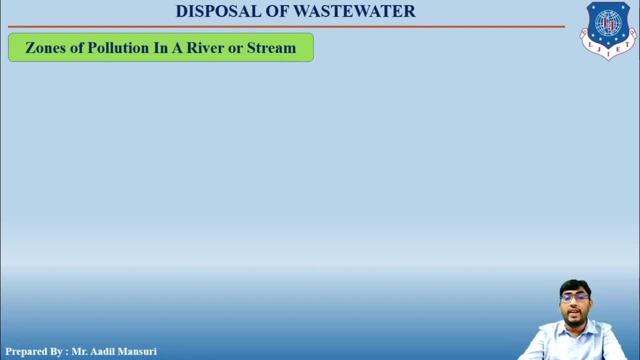 Thus, the self-purification process is only possible if the concentration of pollutants is less than the total amount of oxygen that is released from the atmosphere. Thus, the self-purification process is only possible if the concentration of pollutants is less than the total amount of oxygen that is released from the atmosphere. 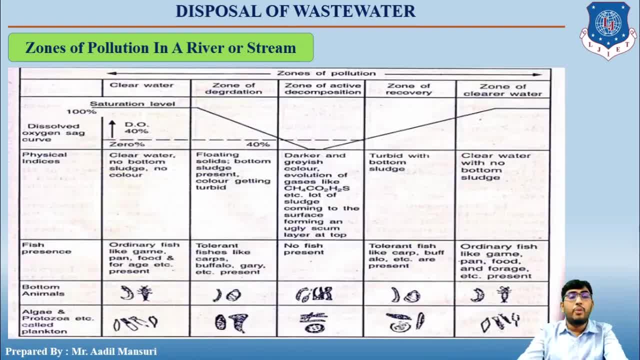 Thus, the self-purification process is only possible if the concentration of pollutants is less than the total amount of oxygen that is released from the atmosphere. Thus, the self-purification process is only possible if the concentration of pollutants is less than the total amount of oxygen that is released from the atmosphere. 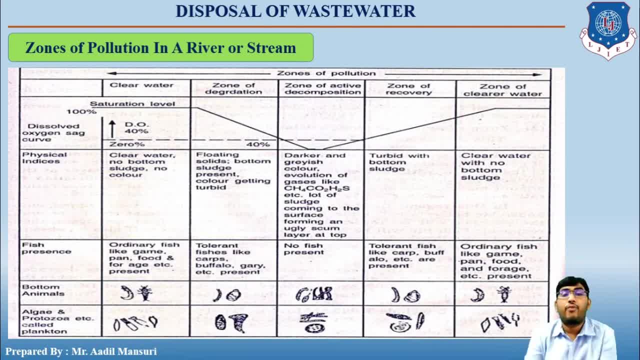 Thus, the self-purification process is only possible if the concentration of pollutants is less than the total amount of oxygen that is released from the atmosphere. Thus, the self-purification process is only possible if the concentration of pollutants is less than the total amount of oxygen that is released from the atmosphere. 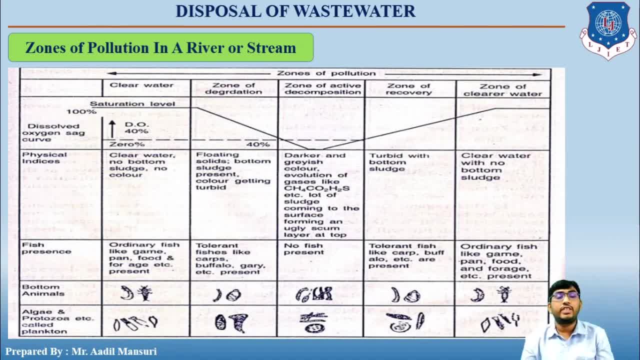 Thus, the self-purification process is only possible if the concentration of pollutants is less than the total amount of oxygen that is released from the atmosphere. Thus, the self-purification process is only possible if the concentration of pollutants is less than the total amount of oxygen that is released from the atmosphere. 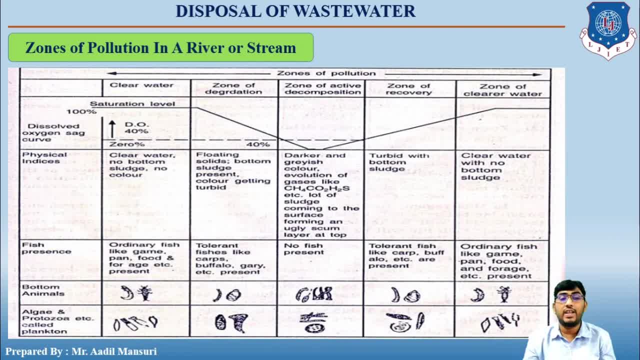 Thus, the self-purification process is only possible if the concentration of pollutants is less than the total amount of oxygen that is released from the atmosphere. Thus, the self-purification process is only possible if the concentration of pollutants is less than the total amount of oxygen that is released from the atmosphere. 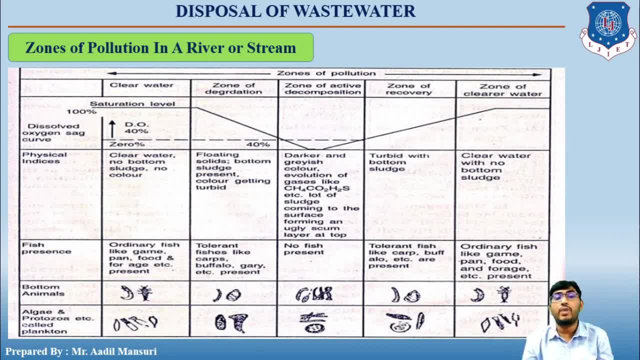 Thus, the self-purification process is only possible if the concentration of pollutants is less than the total amount of oxygen that is released from the atmosphere. Thus, the self-purification process is only possible if the concentration of pollutants is less than the total amount of oxygen that is released from the atmosphere. 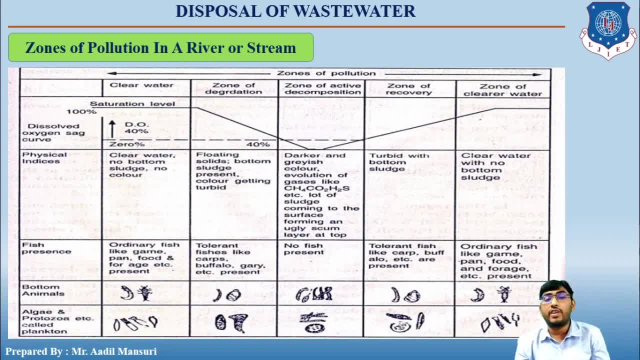 Thus, the self-purification process is only possible if the concentration of pollutants is less than the total amount of oxygen that is released from the atmosphere. Thus, the self-purification process is only possible if the concentration of pollutants is less than the total amount of oxygen that is released from the atmosphere. 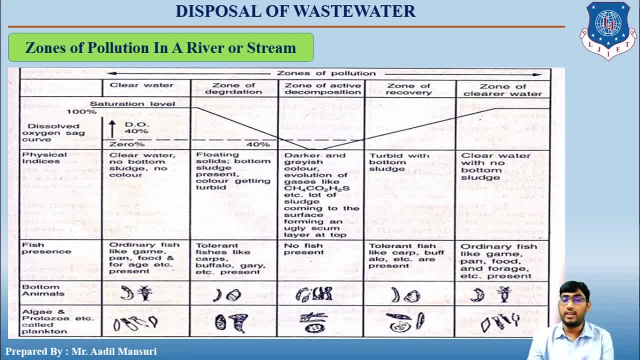 Thus, the self-purification process is only possible if the concentration of pollutants is less than the total amount of oxygen that is released from the atmosphere. Thus, the self-purification process is only possible if the concentration of pollutants is less than the total amount of oxygen that is released from the atmosphere. 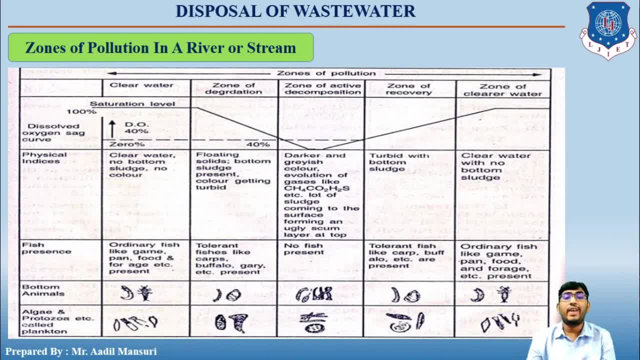 Thus, the self-purification process is only possible if the concentration of pollutants is less than the total amount of oxygen that is released from the atmosphere. Thus, the self-purification process is only possible if the concentration of pollutants is less than the total amount of oxygen that is released from the atmosphere. 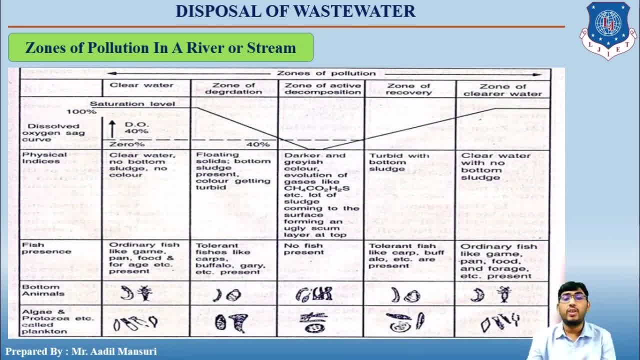 Thus, the self-purification process is only possible if the concentration of pollutants is less than the total amount of oxygen that is released from the atmosphere. Thus, the self-purification process is only possible if the concentration of pollutants is less than the total amount of oxygen that is released from the atmosphere. 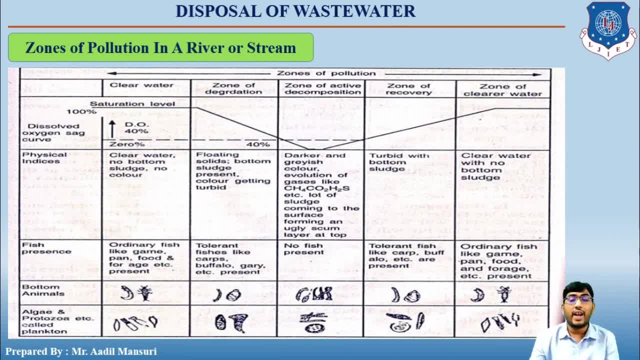 Thus, the self-purification process is only possible if the concentration of pollutants is less than the total amount of oxygen that is released from the atmosphere. Thus, the self-purification process is only possible if the concentration of pollutants is less than the total amount of oxygen that is released from the atmosphere. 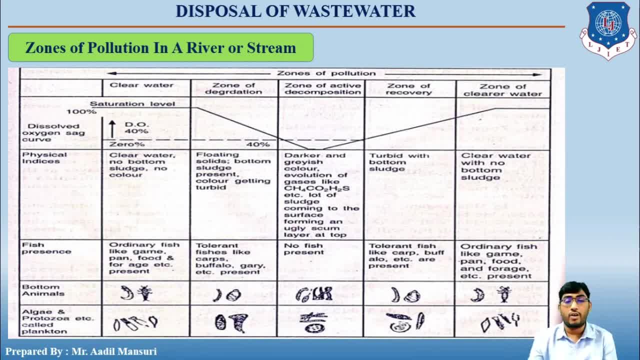 Thus, the self-purification process is only possible if the concentration of pollutants is less than the total amount of oxygen that is released from the atmosphere. Thus, the self-purification process is only possible if the concentration of pollutants is less than the total amount of oxygen that is released from the atmosphere. 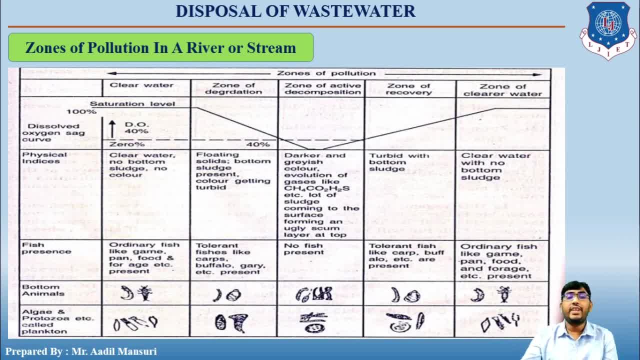 Thus, the self-purification process is only possible if the concentration of pollutants is less than the total amount of oxygen that is released from the atmosphere. Thus, the self-purification process is only possible if the concentration of pollutants is less than the total amount of oxygen that is released from the atmosphere. 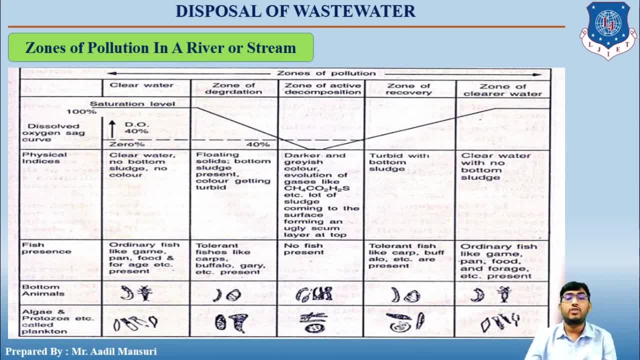 Thus, the self-purification process is only possible if the concentration of pollutants is less than the total amount of oxygen that is released from the atmosphere. Thus, the self-purification process is only possible if the concentration of pollutants is less than the total amount of oxygen that is released from the atmosphere. 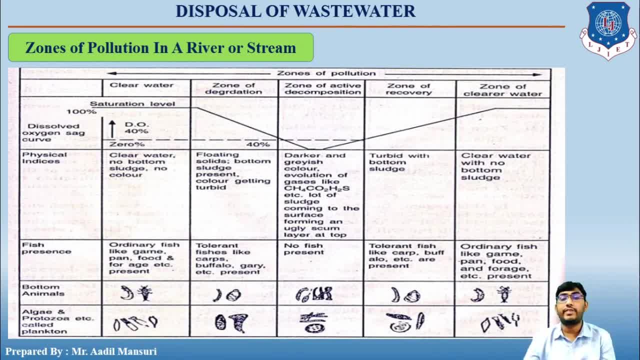 Thus, the self-purification process is only possible if the concentration of pollutants is less than the total amount of oxygen that is released from the atmosphere. Thus, the self-purification process is only possible if the concentration of pollutants is less than the total amount of oxygen that is released from the atmosphere. 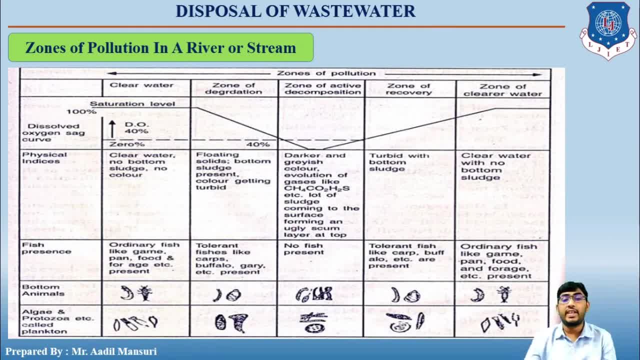 Thus, the self-purification process is only possible if the concentration of pollutants is less than the total amount of oxygen that is released from the atmosphere. Thus, the self-purification process is only possible if the concentration of pollutants is less than the total amount of oxygen that is released from the atmosphere. 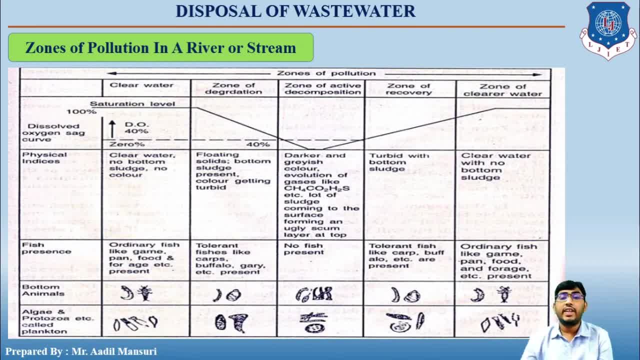 Thus, the self-purification process is only possible if the concentration of pollutants is less than the total amount of oxygen that is released from the atmosphere. Thus, the self-purification process is only possible if the concentration of pollutants is less than the total amount of oxygen that is released from the atmosphere. 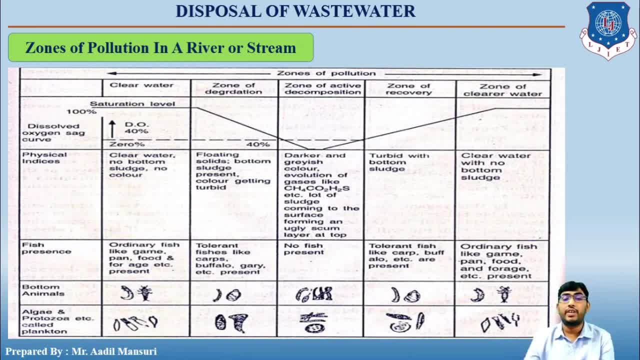 Thus, the self-purification process is only possible if the concentration of pollutants is less than the total amount of oxygen that is released from the atmosphere. Thus, the self-purification process is only possible if the concentration of pollutants is less than the total amount of oxygen that is released from the atmosphere. 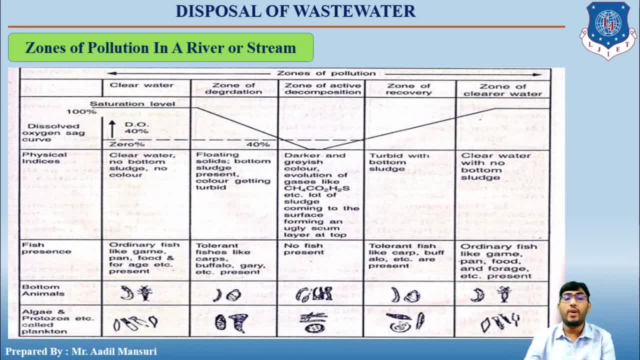 Thus, the self-purification process is only possible if the concentration of pollutants is less than the total amount of oxygen that is released from the atmosphere. Thus, the self-purification process is only possible if the concentration of pollutants is less than the total amount of oxygen that is released from the atmosphere. 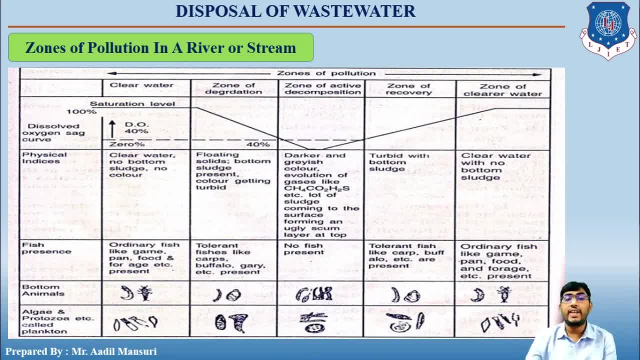 Thus, the self-purification process is only possible if the concentration of pollutants is less than the total amount of oxygen that is released from the atmosphere. Thus, the self-purification process is only possible if the concentration of pollutants is less than the total amount of oxygen that is released from the atmosphere. 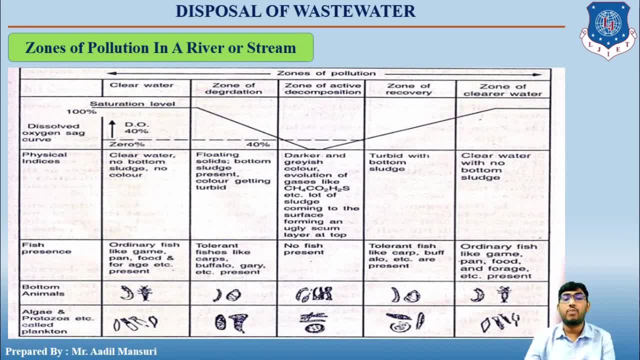 Thus, the self-purification process is only possible if the concentration of pollutants is less than the total amount of oxygen that is released from the atmosphere. Thus, the self-purification process is only possible if the concentration of pollutants is less than the total amount of oxygen that is released from the atmosphere. 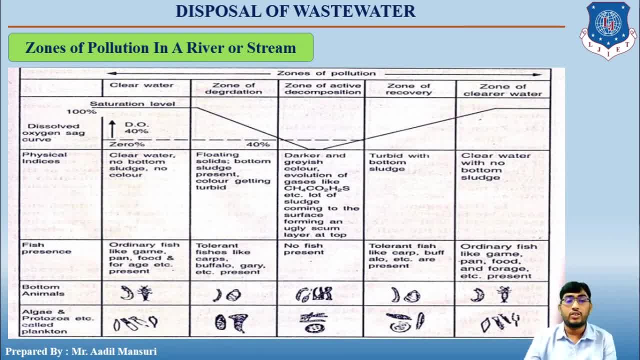 Thus, the self-purification process is only possible if the concentration of pollutants is less than the total amount of oxygen that is released from the atmosphere. Thus, the self-purification process is only possible if the concentration of pollutants is less than the total amount of oxygen that is released from the atmosphere. 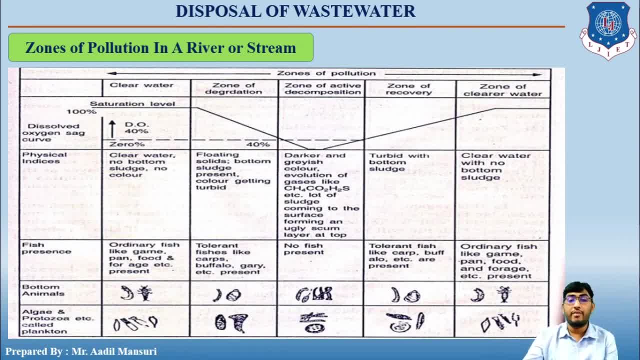 Thus, the self-purification process is only possible if the concentration of pollutants is less than the total amount of oxygen that is released from the atmosphere. Thus, the self-purification process is only possible if the concentration of pollutants is less than the total amount of oxygen that is released from the atmosphere. 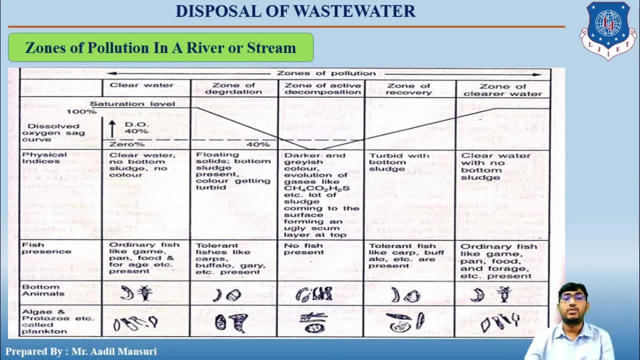 Thus, the self-purification process is only possible if the concentration of pollutants is less than the total amount of oxygen that is released from the atmosphere. Thus, the self-purification process is only possible if the concentration of pollutants is less than the total amount of oxygen that is released from the atmosphere. 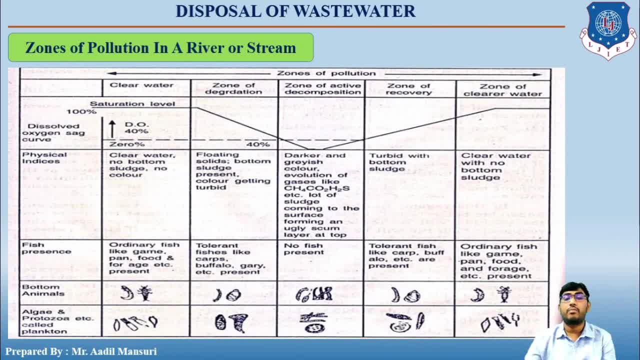 Thus, the self-purification process is only possible if the concentration of pollutants is less than the total amount of oxygen that is released from the atmosphere. Thus, the self-purification process is only possible if the concentration of pollutants is less than the total amount of oxygen that is released from the atmosphere. 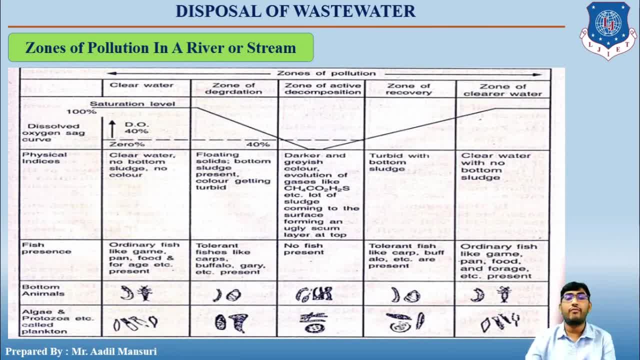 Thus, the self-purification process is only possible if the concentration of pollutants is less than the total amount of oxygen that is released from the atmosphere. Thus, the self-purification process is only possible if the concentration of pollutants is less than the total amount of oxygen that is released from the atmosphere. 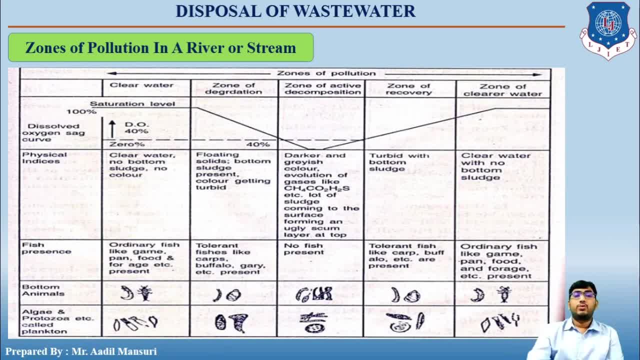 Thus, the self-purification process is only possible if the concentration of pollutants is less than the total amount of oxygen that is released from the atmosphere. Thus, the self-purification process is only possible if the concentration of pollutants is less than the total amount of oxygen that is released from the atmosphere. 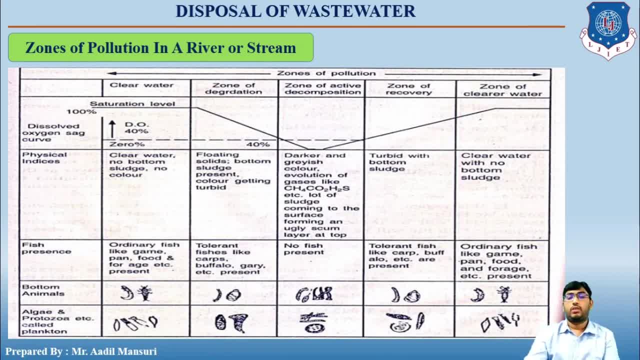 Thus, the self-purification process is only possible if the concentration of pollutants is less than the total amount of oxygen that is released from the atmosphere. Thus, the self-purification process is only possible if the concentration of pollutants is less than the total amount of oxygen that is released from the atmosphere. 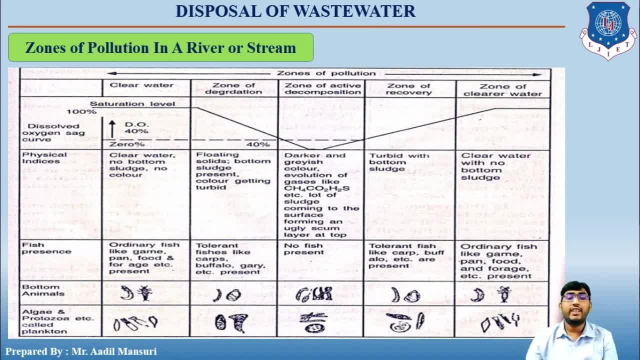 Thus, the self-purification process is only possible if the concentration of pollutants is less than the total amount of oxygen that is released from the atmosphere. Thus, the self-purification process is only possible if the concentration of pollutants is less than the total amount of oxygen that is released from the atmosphere. 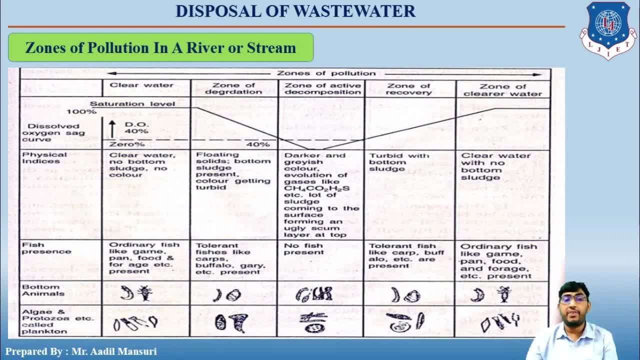 Thus, the self-purification process is only possible if the concentration of pollutants is less than the total amount of oxygen that is released from the atmosphere. Thus, the self-purification process is only possible if the concentration of pollutants is less than the total amount of oxygen that is released from the atmosphere. 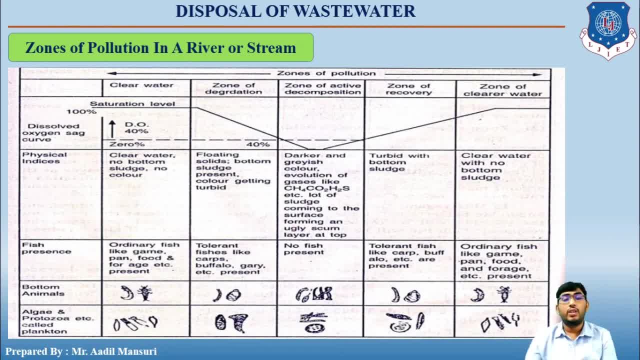 Thus, the self-purification process is only possible if the concentration of pollutants is less than the total amount of oxygen that is released from the atmosphere. In this zone, dissolved oxygen concentration falls down to zero, right. as a result, anaerobic conditions will set up, resulting in formation of gases like methane, carbon dioxide, hydrogen sulfide, okay. and lot of sludge is coming to the surface, forming an ugly scum layer at the top, okay. 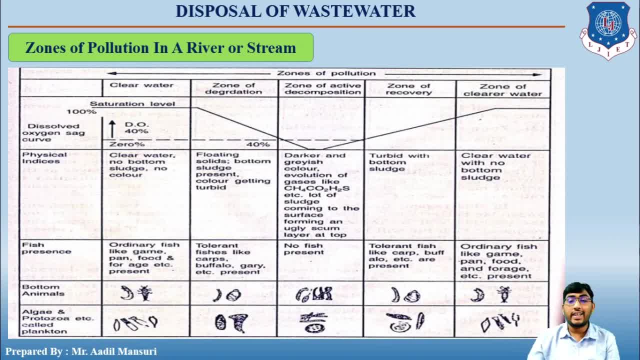 Now, as the organic decomposition slackens due to stabilization of organic matter, rate of deoxygenating becomes lesser than the re-aeration rate and dissolved oxygen again rises to the original level. okay, So initially what happens? Decomposition at a higher rate and dissolved oxygen will reduce to zero. but as it will reduce the decomposition rate, so the dissolved oxygen. 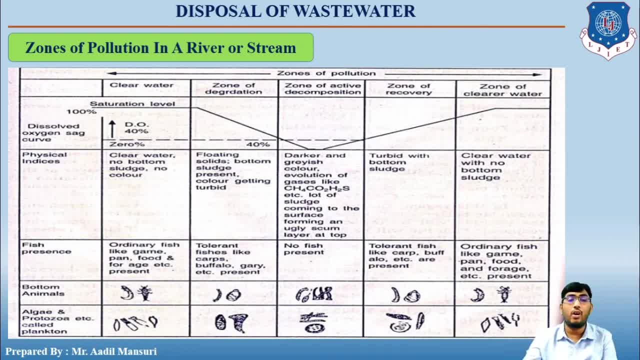 will start on increasing and it will again rise to the original level of 40%. Now, in this region, the bacteria or flora will flourish. At the upper end, anaerobic bacteria will replace the aerobic bacteria, while at the lower end the position will be reversed. 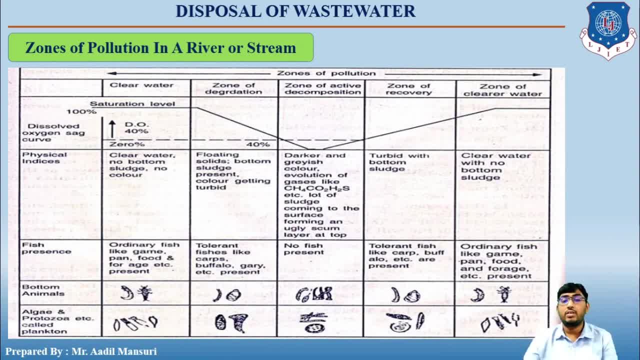 Protozoa and fungi first disappear, then reappear. Fish life will be absent. Algae tubifacts will also be absent. Maggots and psychoda, that is, sewage fly larvae, will, however, be present in all but most septic sewage. okay. 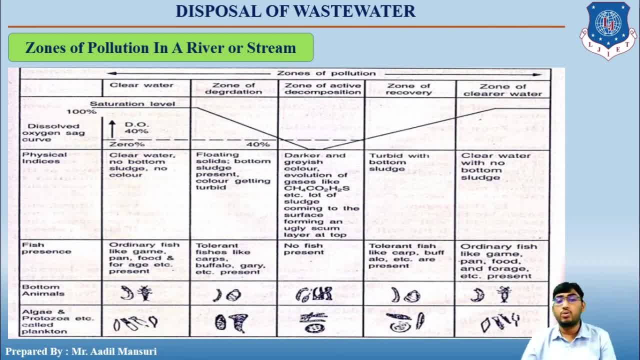 Next is zone of recovery. So in this zone of recovery, the river stream tries to recover from degraded condition to its former appearance. The water becomes clearer, and so the algae re-evolves. So in this zone of recovery, the river stream tries to recover from degraded condition to its former appearance. The water becomes clearer, and so the algae re-evolves. 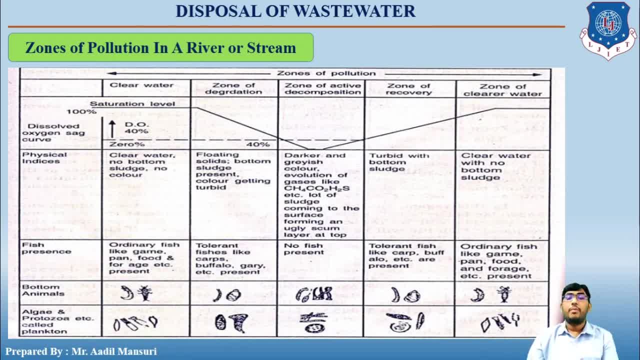 If the area of water gets 1978, BOD decreases and dissolved oxygen content rises above 40 percent of the saturation value. and protozoa rotiferous and large plants like sponges. BOD decreases and dissolved oxygen content rises above 44% of the saturation value. and protozoa rotiferous and large plants like sponges. 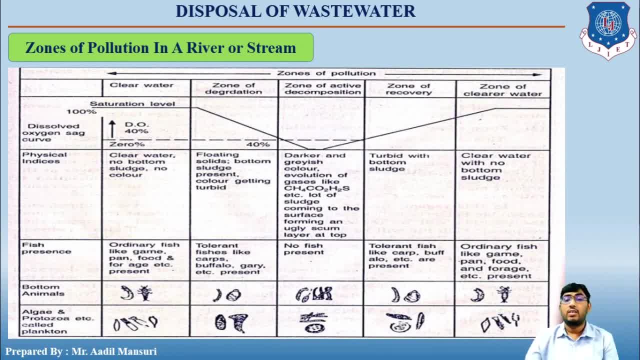 andalı own Etc will occur. The organic material will be mineralized to form nitrate, phosphate and carbonates. okay, Last is the zone of the celiac disease cure. Last is the zone of the celiac disease cure. 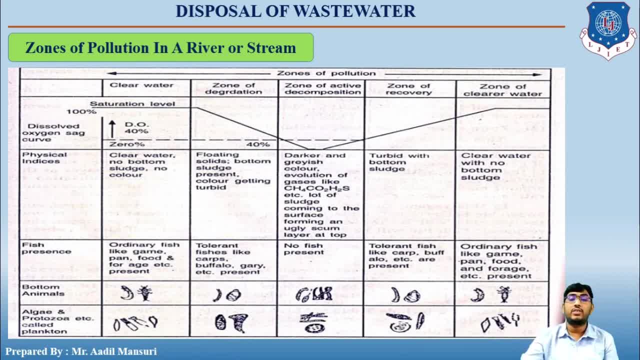 zone of clearer water. so in this zone the river attains its original condition, with dissolved oxygen rising up to the saturation level that is um okay. water becomes attractive in appearance. fish, which requires at least four to five milligram per liter of dissolved oxygen, and usual aquatic life prevails. some paragonic organisms may still, however, survive and remain. 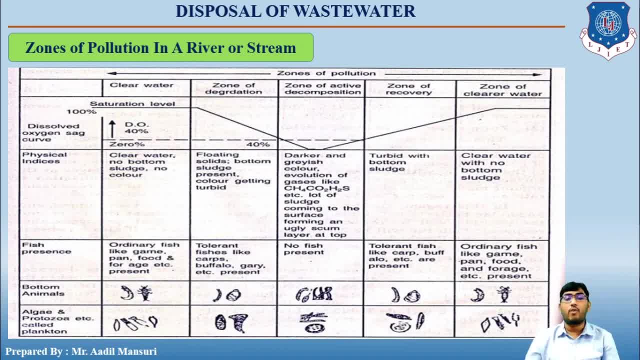 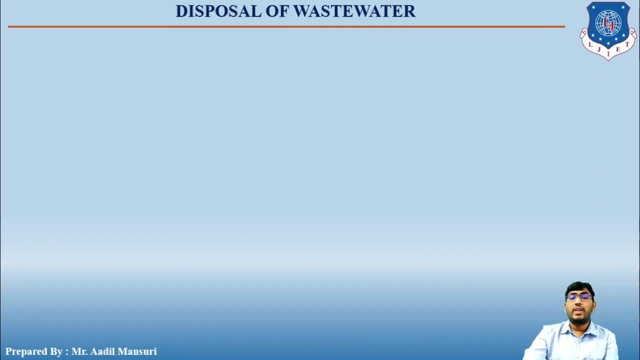 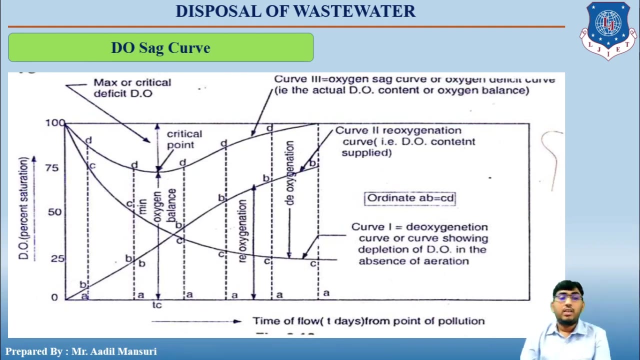 present, which confirms the fact that once the river water has been polluted, it will not be safe for drinking unless it is properly treated. okay, so these are the different zones of pollution in a river or stream. so let us now talk about deosec. okay, so you can see in the screen, uh. 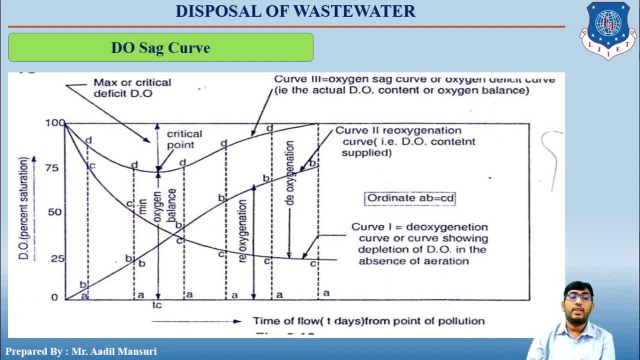 on the y-axis, that is dissolved oxygen, okay, it is in percentage, and on the y-axis it is time of flow, okay, so first let me talk about deoxygenation. okay, so the curve one is the deoxygenation curve, which shows that with the passage of time, the 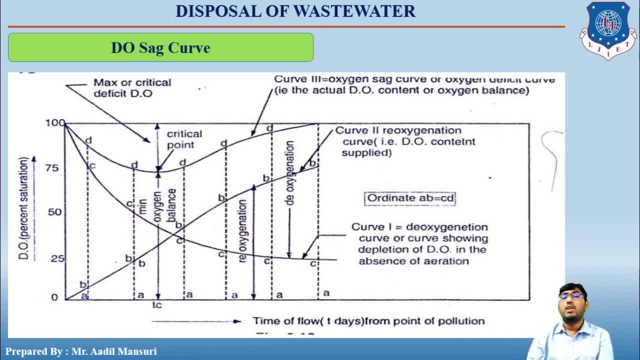 dissolved oxygen is reducing, okay, so deoxygenation curve. what does it mean? so in a polluted stream, the dissolved oxygen content goes on reducing due to decomposition of volatile organic matter. now the rate of deoxygenation depends upon the amount of organic matter remaining to be oxidized. 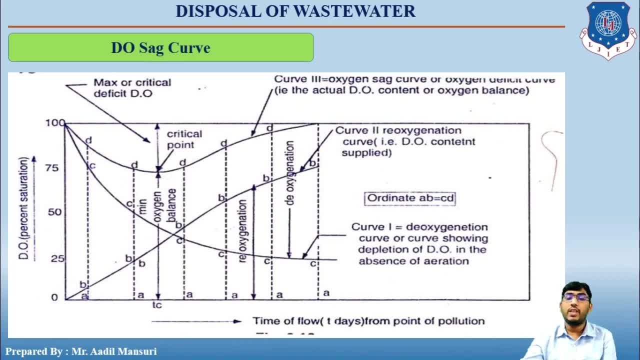 at the given time, as well as the temperature of the reaction. hence, at a given temperature, the curve showing depletion of dissolved oxygen with time, which is called deoxygenation curve, is also similar to the first stage of bod. okay, so here on the screen you can see the curve which is 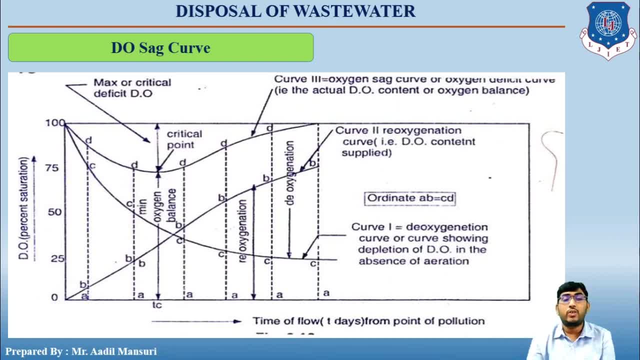 showing downwards right, which is showing curve one, deoxygenation curve, or curve showing the depletion of do in the absence of aeration. okay now. next curve, curve two: it is re-oxygenation curve. okay, that is do content supplied. okay, now oxygen which is consumed by the bacteria. 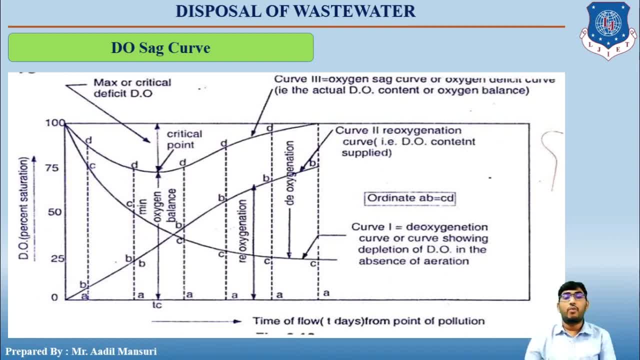 in oxidation of organic matter is replenished from the atmosphere, and this process is known as re-oxygenation process. okay, the rate at which the oxygen is supplied by the atmosphere to the polluted water depends on different factors like velocity of the stream and the resulting turbulence created. more the velocity, more will be the oxygenation rate. now, second is the depth. 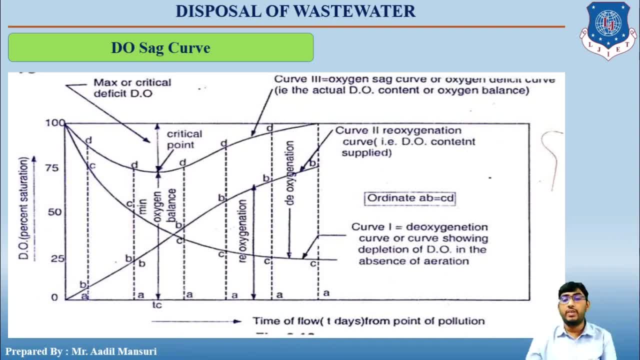 of the receiving water. lesser is the depth, more will be, more will be the rate of re-oxygenation. rate of re-oxygenation decreases with increase in temperature- okay. and then the saturation deficit, or the oxygen deficit below the saturation value: okay, depending upon these factors, 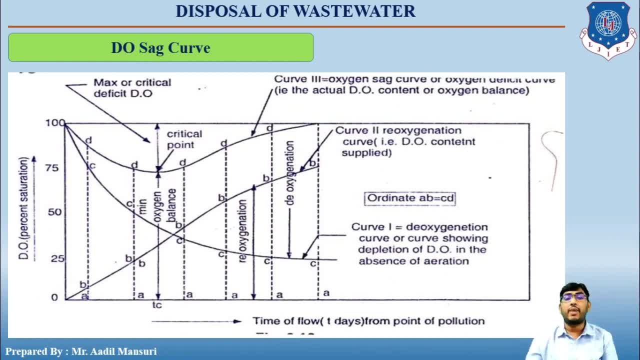 the rate of deoxygenation can be expressed mathematically and plotted in the form of curve called re-oxygenation curve. okay, and finally, the next curve, which is known as oxygen sac curve, or oxygen deficit curve, or do sac curve, is the curve which is on the top portion. 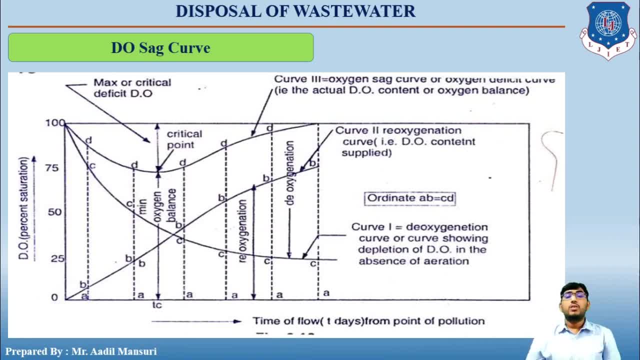 that is curve three oxygen sac curve. okay, so in running polluted stream exposed to the atmosphere the deoxygenation and re-oxygenation processes occur simultaneously. if the deoxygenation is more rapid, then the reoxygenation and oxygen deficit occurs. number one and the amount of the 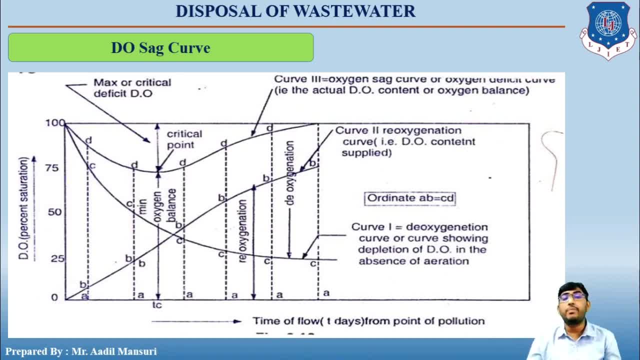 the resultant oxygen deficit can be obtained by algebrically adding the deoxygenation and the reoxygenation curves. okay, the resultant curve so obtained is known as the oxygen sac curve or oxygen deficit curve. okay, clear. so, as you can see that with the passage of time the rate of 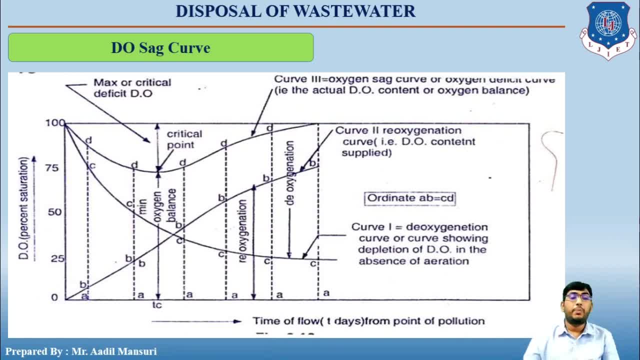 dissolved oxygen reduces, which is denoted by curve one. with the passage of time, reoxygenation occurs from the atmosphere, which is shown by curve two and the deficit of the oxygen right. the deficit of the oxygen will be obtained by algebrically adding those two curves, which is known as. 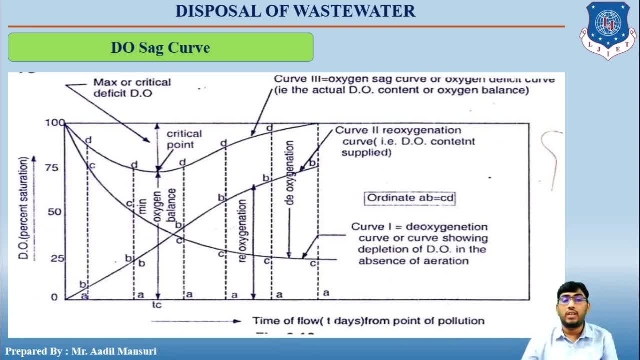 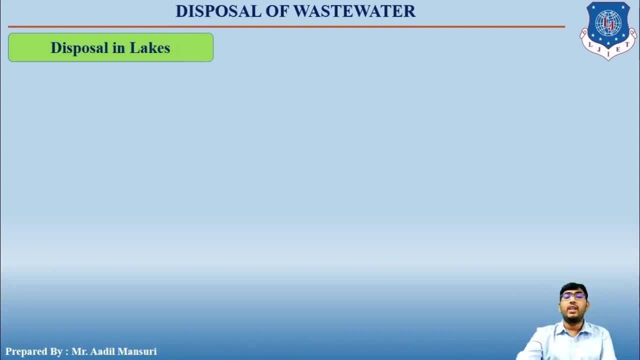 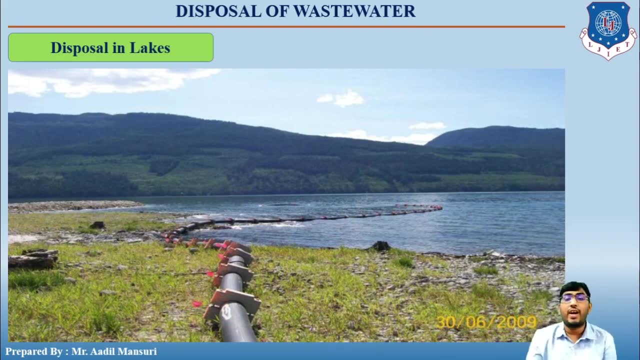 deoxy curves. that is the curve number three. okay, so next is disposal in lake. okay, so disposal of displacement, displacement, displacement velocity water in confined in, much more harmful than its disposal in flowing stream and reverse water quality management is entirely different from that is in reverse. now the river is flowing water body, while lake is stagnant water body. 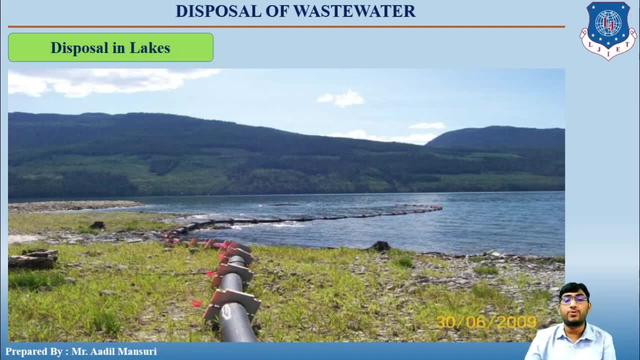 okay. so in lakes only top surface would become saturated with this all oxygen, but the bottom layers would not have enough oxygen. over turning of the layers would not occur frequently, so the dissolved oxygen content would not be uniform throughout the depth of the lake. overturning takes place only when there. 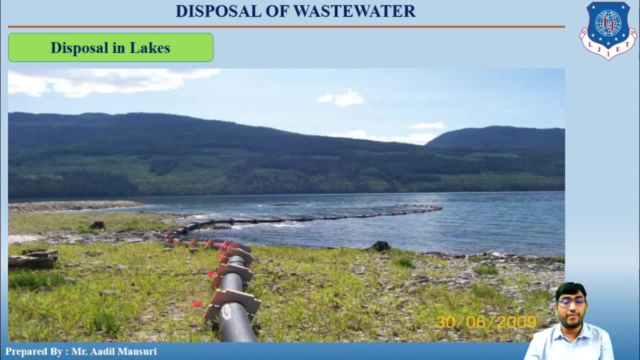 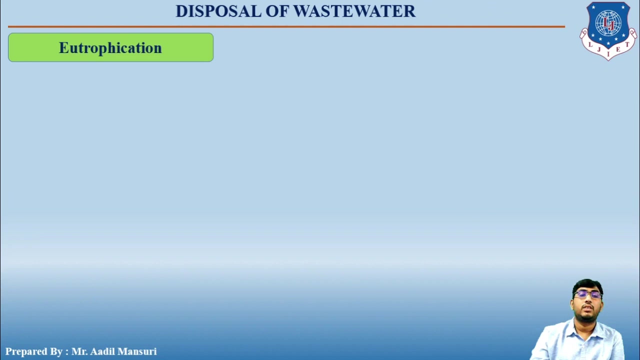 is a change in the season, due to which there will be temperature difference between water in different layers, which causes change in the density of different layers and overturning occurs. okay, so this is the disposal in lakes. okay, students, so let us see the next slide. now move towards the next topic, that is, the eutrophication. so you might have seen. 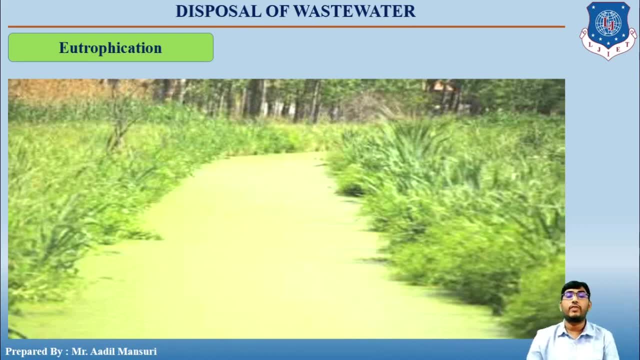 in different water bodies that the top layer of the water body is covered with algae or any other aquatic plants. okay, so phosphorus acts as the nutrients for algal growth. okay, an increase in phosphorus content would increase the algal growth. excessive amount of the phosphorus content would increase the algal growth. 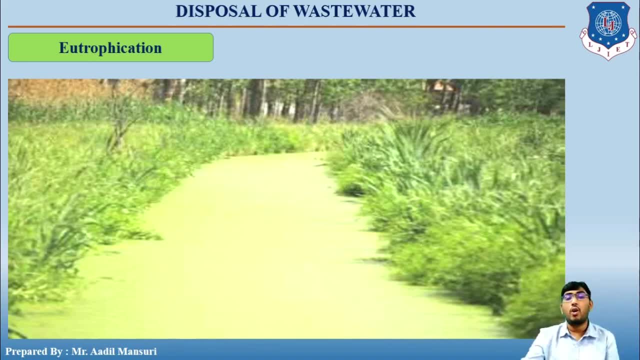 so excessive algal growth will create lot of problems like taste odor, problems in oxygen diffusion in lower layer. ultimately, the entire lake gets covered with the algae and it may become useless for other organisms. so this process is known as eutrophication. okay, so let us now move towards the next topic, that is, 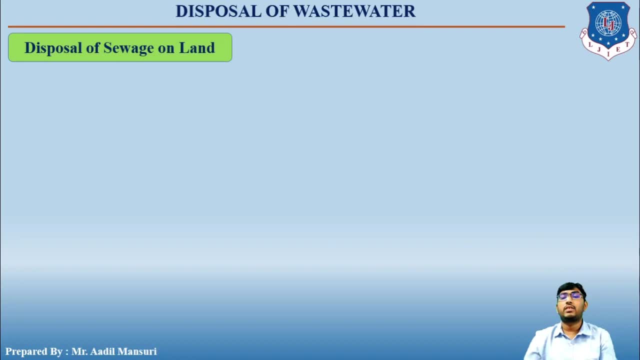 disposal of sewage on land. okay, so in this method, the sewage effluent, treated or either it's raw, is disposed of on the land by applying on it, and the most common forms of land application are irrigation. that is known as sewage farming or rapid infiltration. okay, when raw or partly. 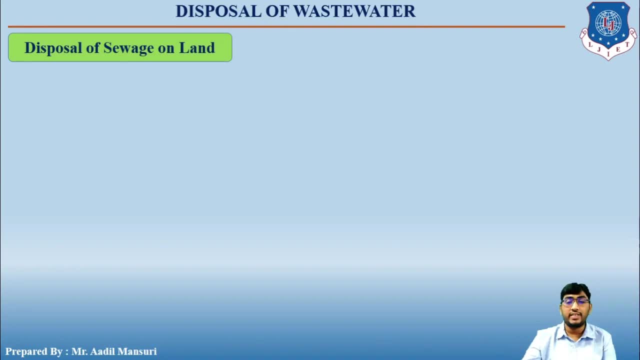 treated sewage is applied on land, a part of it evaporates and remaining portion percolates in the soil. if proper voids are made, then the soil will sedimentate in the soil. maintained in the soil, the organic sewage solids are oxidized by the bacteria present in the soil. 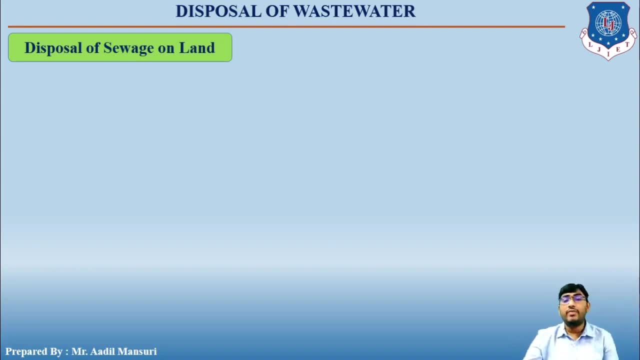 under aerobic condition. However, if the soil is made of heavy, sticky and fine-grained material, the void space will soon get clogged, resulting in non-aeration of these voids, which would lead to anaerobic condition and subsequent evolution of foul gases. Application of too strong or too 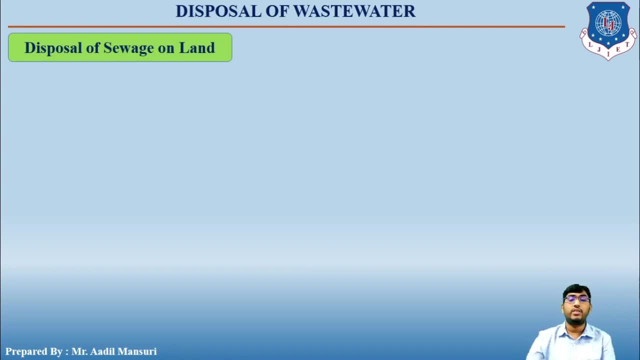 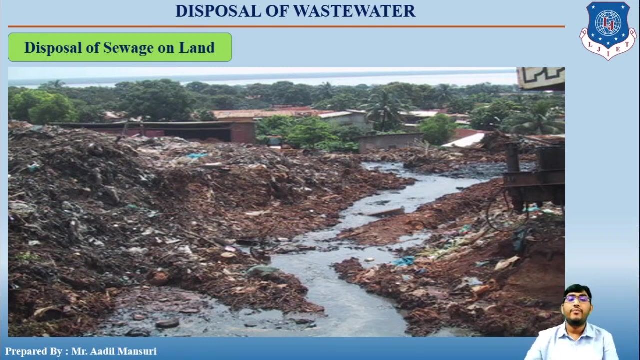 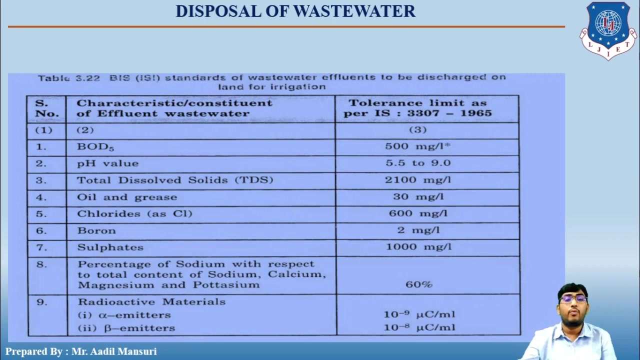 hard sewage will also result in quick formation of anaerobic condition, and the load of sewage can be reduced by dilution or pretreatment. So you can see the picture of sewage disposal on land. okay, And these are different standards of wastewater effluents to be discharged. 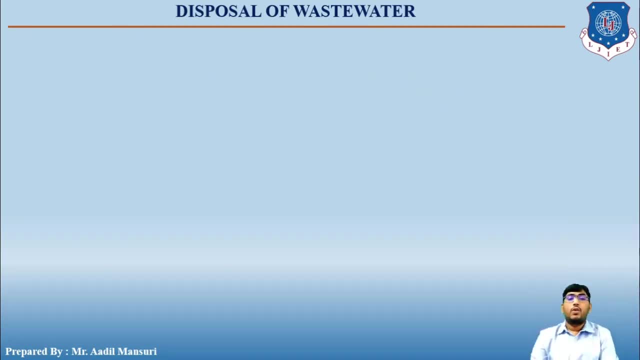 on land for irrigation. Okay, students. So let us now move towards the next topic, that is, sewage farming. Okay, So in irrigation, sewage is used for irrigation of crops. Okay, In this method, this not only disposing of sewage. 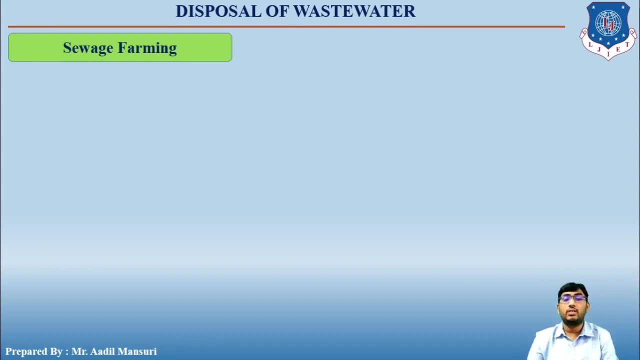 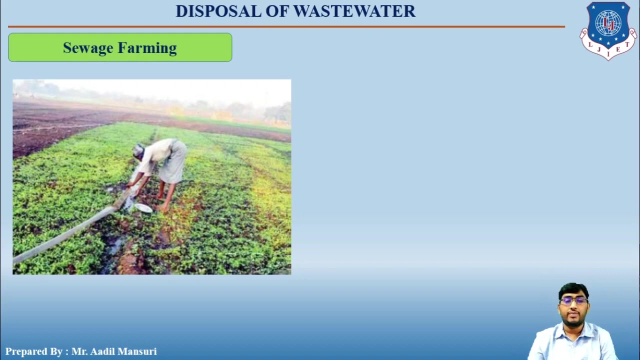 occurs, but also it helps in yielding the crops- Okay. It increases the yield capacity of the crops because sewage contains lots of nutrients- Okay. However, the sewage effluent may be made before using it for the irrigation- Okay. So you can see the pictures of sewage farming. 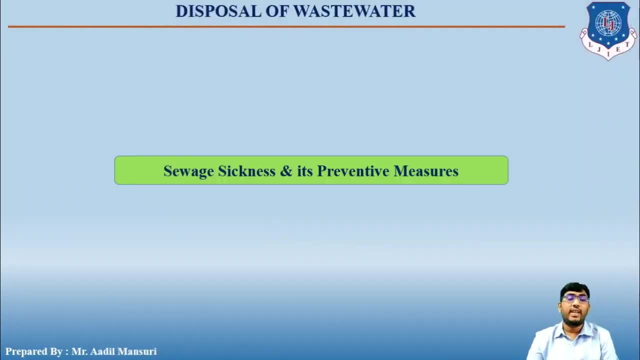 So next topic is sewage sickness and its preventive measures. So when sewage is applied continuously on a piece of land, the soil, pores or voids may get filled up or clogged up with sewage matter retained in them. The time taken for such clogging will depend upon the type of soil and the 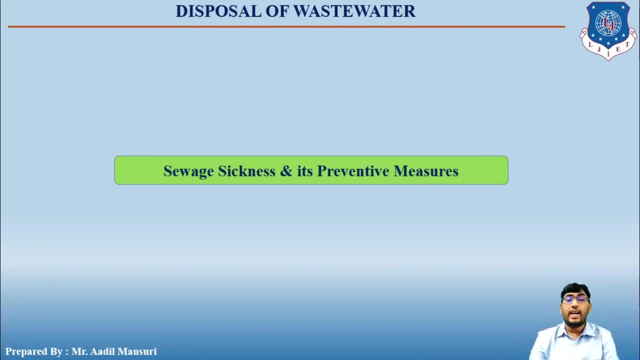 load present in the sewage, But once these voids get clogged, free circulation of air will be prevented and anaerobic condition will develop within the pores. This results in decomposition of the organic matter right under an anaerobic condition and this results in evolution of foul gases like hydrogen sulfide and 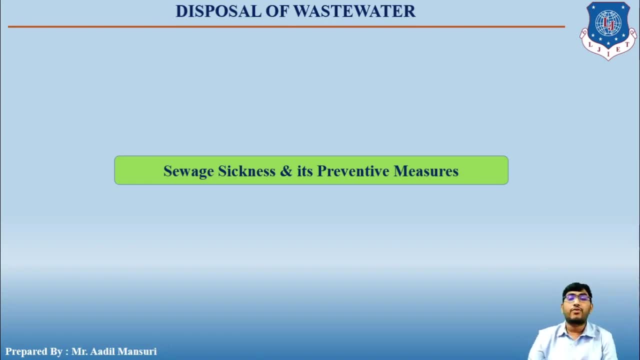 carbon dioxide and methane. This phenomenon of soil getting clogged is known as sewage sickness. Okay, Talking about its preventive measures, then primary treatment of sewage should be done, So the sewage should be disposed of only after primary treatment, such as screening, grit removal and sedimentation. 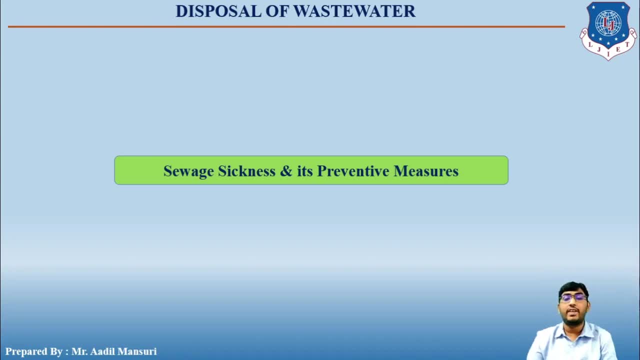 This will help in removing sedentary solids and reducing BOD load by 30% or so, and soil will not get clogged frequently. Then another preventive measure is a choice of land. The piece of land use for sewage disposal should normally be sandy or low�� Inspector. 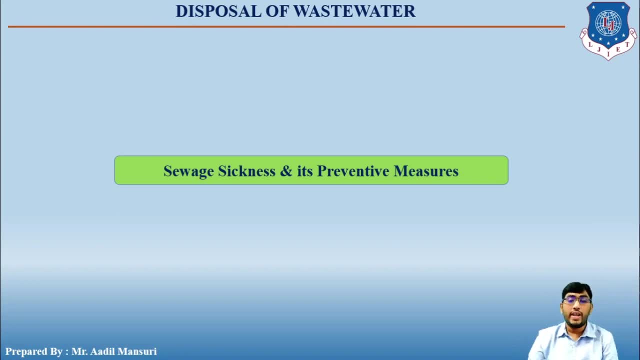 clayey soil or clayey land should be avoided. under drainage of soil is one of another preventive measures. that is, the land on which sewage is to being applied or disposed can be drained, and if system of underdrains is laid below to collect the effluent, then this will minimize. 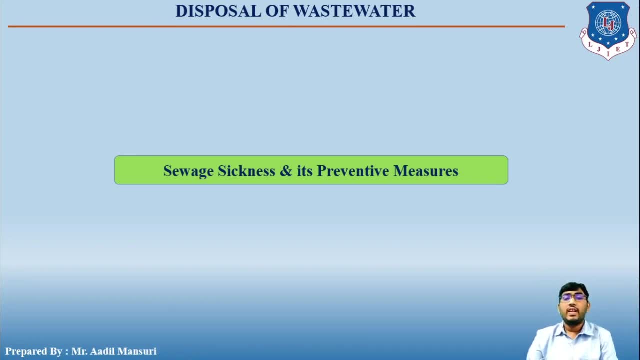 possibility of sewage sickness. then another one is giving rest to land. so the land being used for disposal should be given rest periodically, by keeping some extra land as a reserve and standby for diverting the sewage during the rest period. moreover, during the rest period, the land should 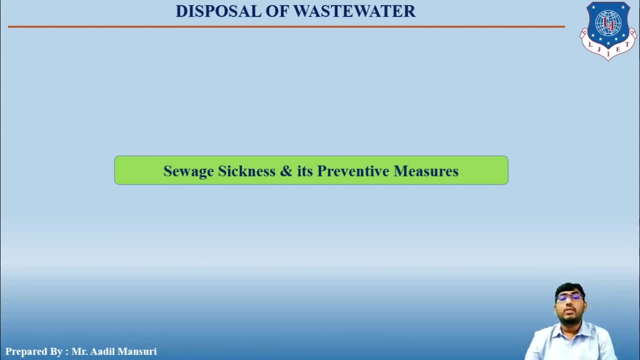 be thoroughly plowed so that it gets broken up and aerated. and last method is rotation of crop. so sewage sickness can be reduced by planting different crops and this will help in utilizing the fertilizing element of sewage and helping erosion of soil. okay, so with this, my dear students, we complete the portion of 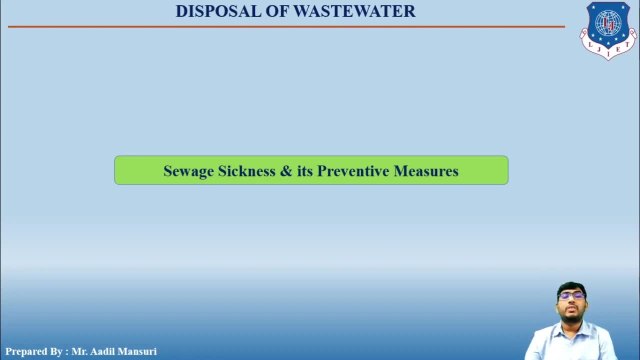 sewage disposal as well. okay, so we will be starting with the new topics in the next video.